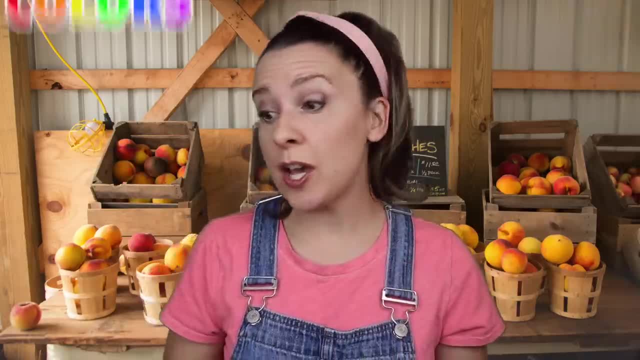 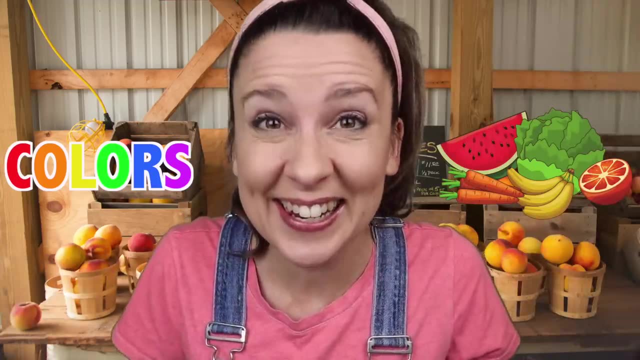 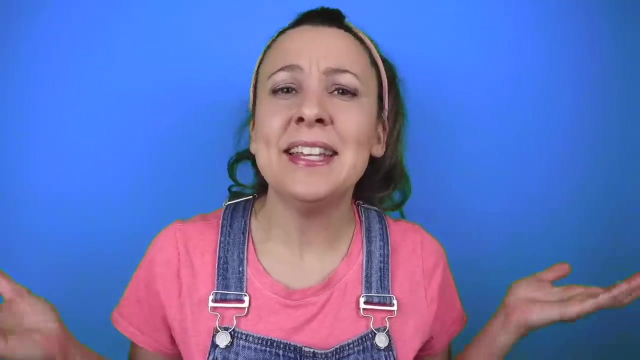 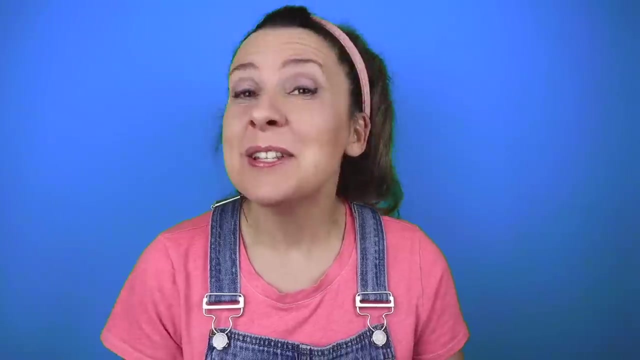 Hi friends, Today let's learn about colors and yummy fruits and vegetables. It's going to be so much fun. Can you think of any yellow foods? Hmm, Maybe if we say food, some yellow foods will come out. Say food, Food. 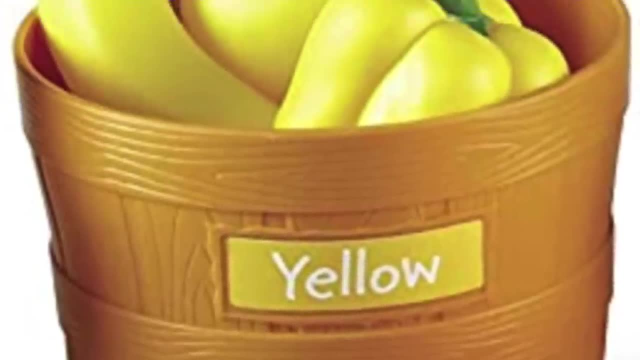 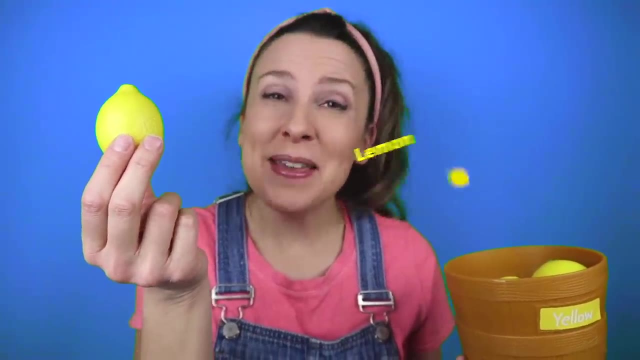 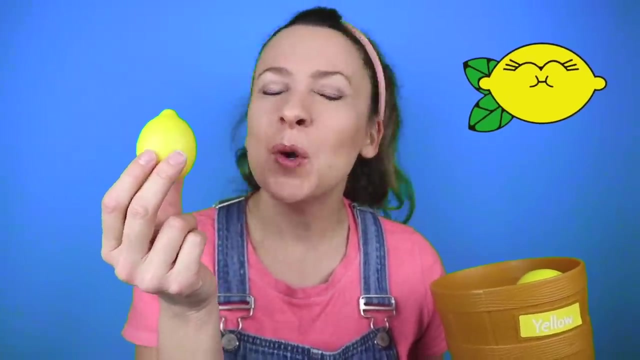 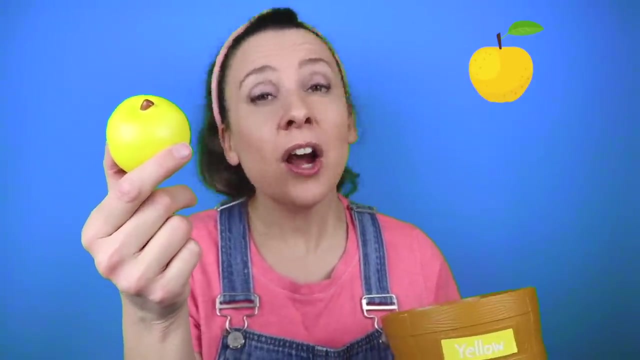 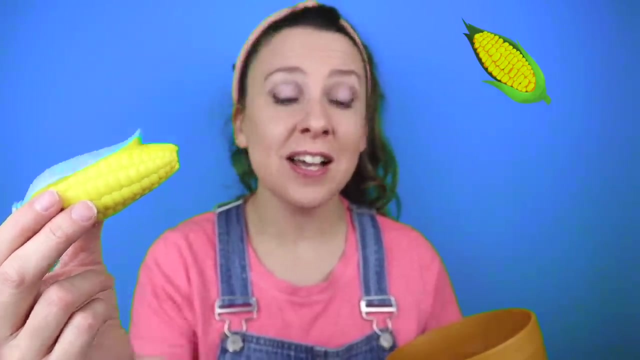 Wow, You said food, and the yellow foods came out. It's a little yellow lemon. Wow, Lemons are so sour. Can you do that? A yellow apple? Yeah, There are some apples that are yellow. This is corn. Good job. 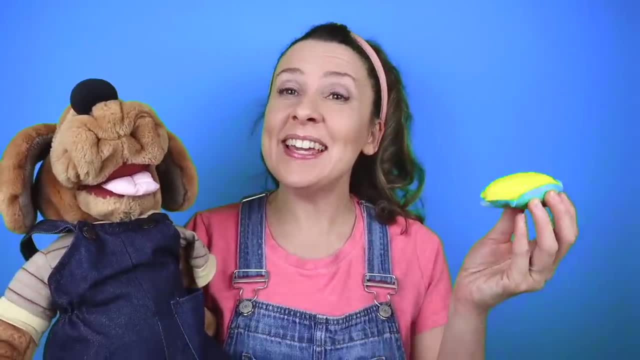 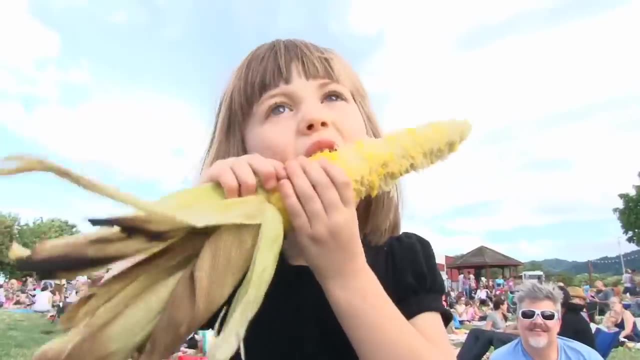 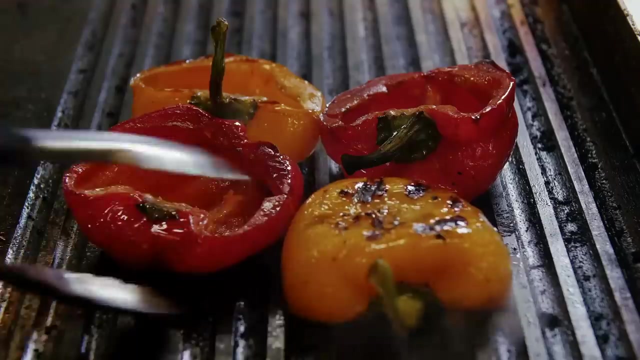 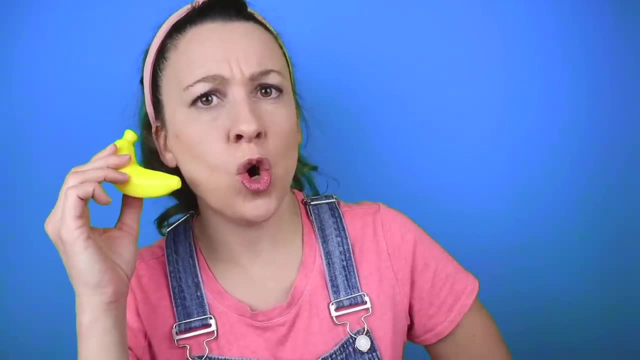 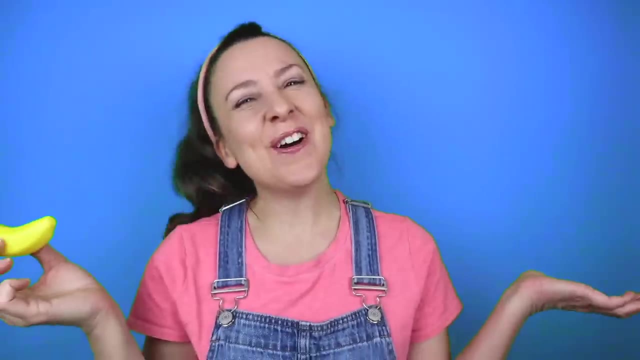 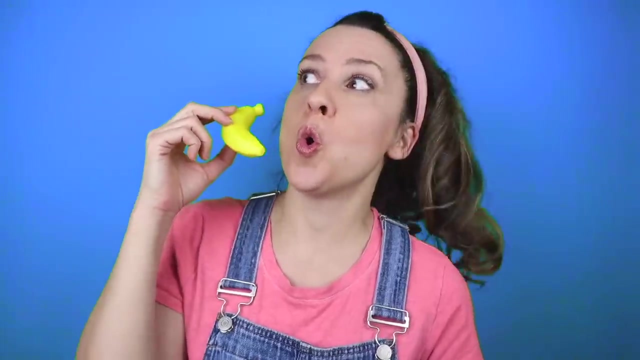 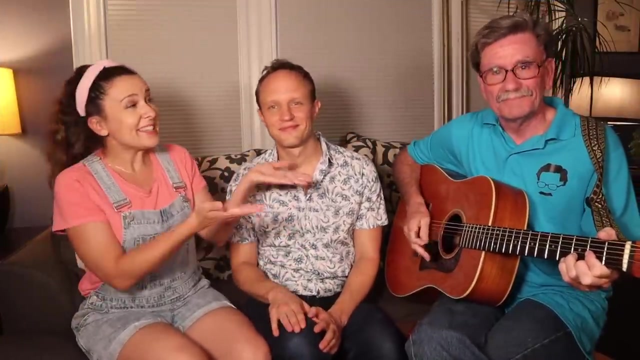 Banana Ring ring, Hello, Ring ring, Hello. This isn't a phone, That's so silly. I'm pretending that the banana is a phone, Hello, Hello. Let's sing apples and bananas with my stepdad, Papa Tim. 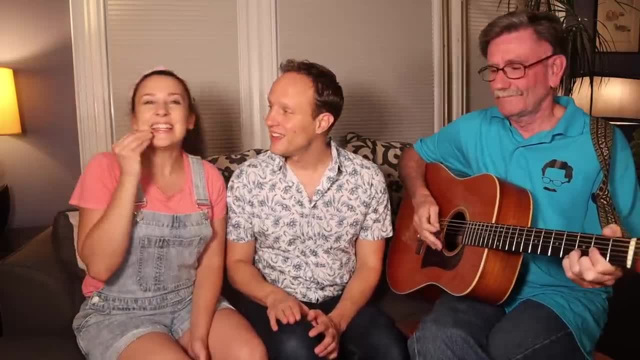 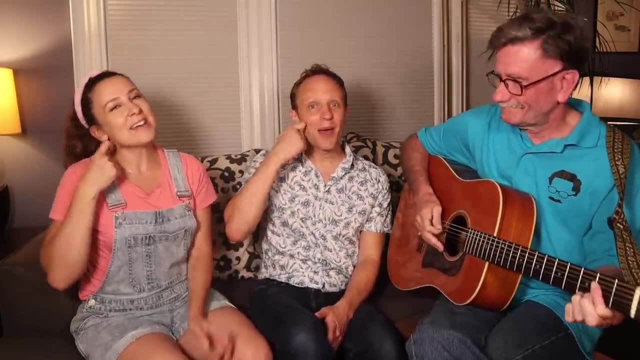 I like to eat Eat, Eat, Eat- Apples and bananas. I like to eat Eat, Eat, Eat- Apples and bananas. I like to eat- Eat, Eat- Apples and bananas. I like to eat. 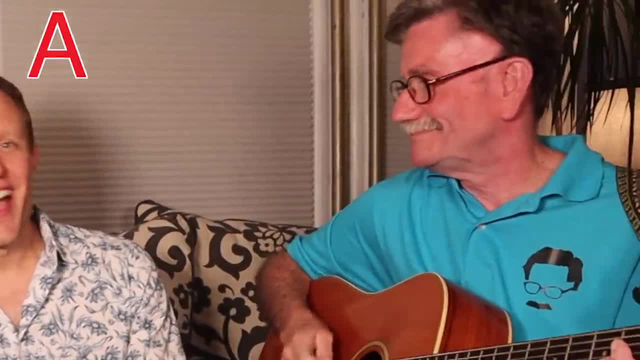 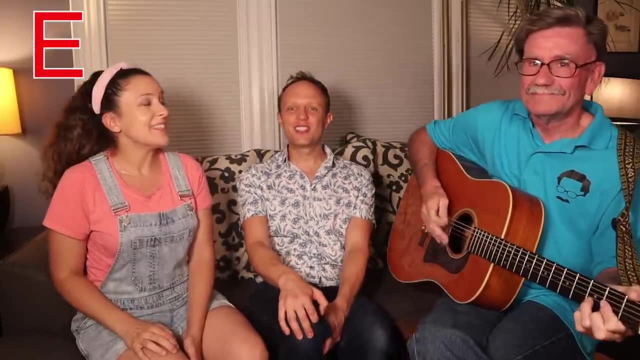 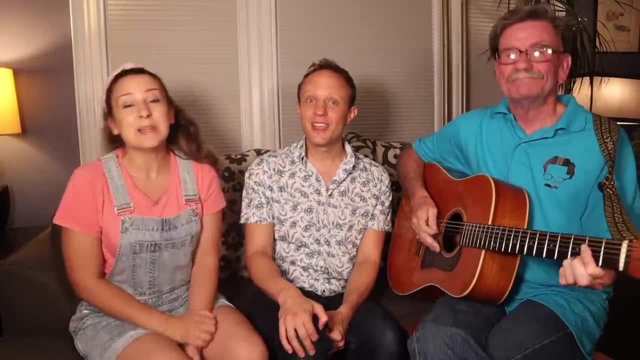 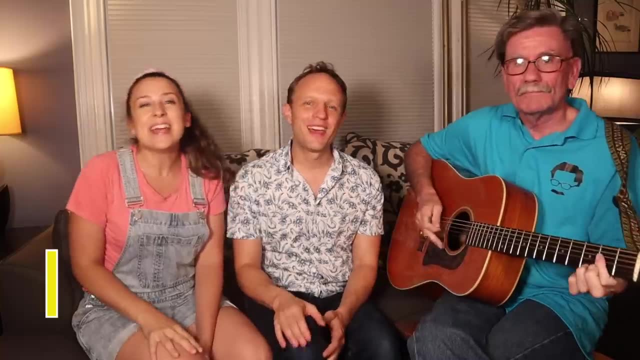 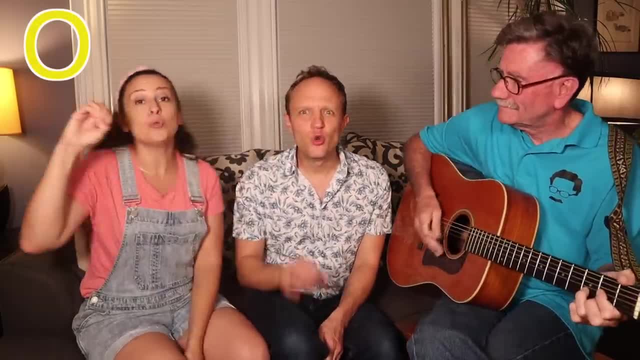 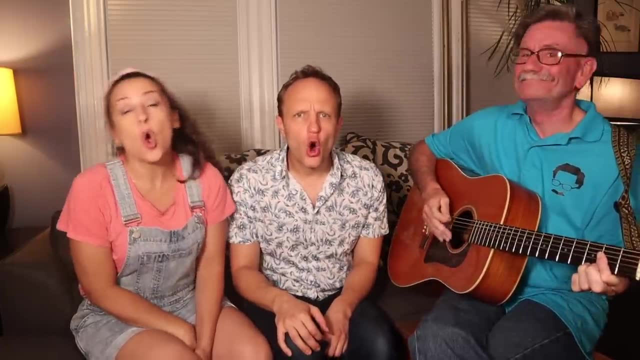 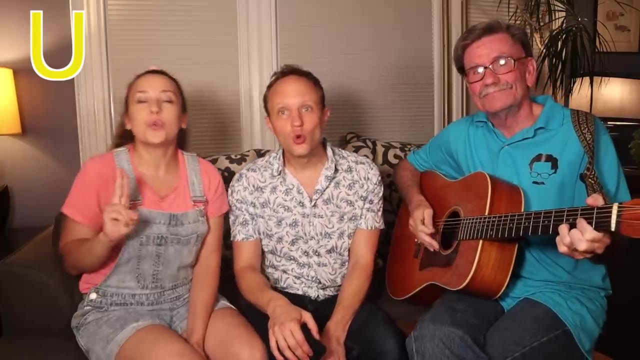 Eat, Eat, Eat- Apples and bananas. I like to eat, Eat, Eat, Eat- Apples and bananas. I like to eat, Eat, Eat- opals and banonos. I like to oot, oot, oot, oopals and banunus. I like to oot, oot, oot. 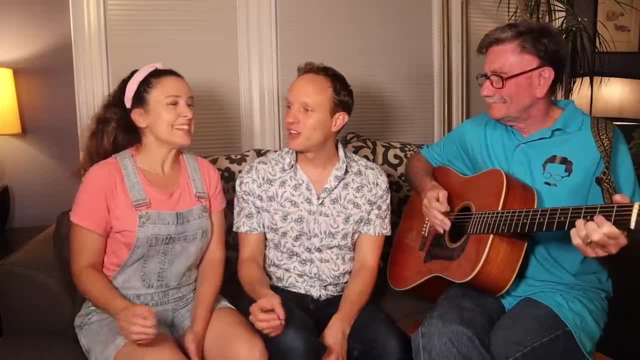 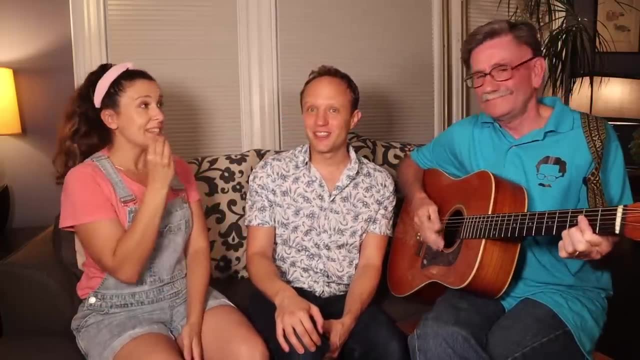 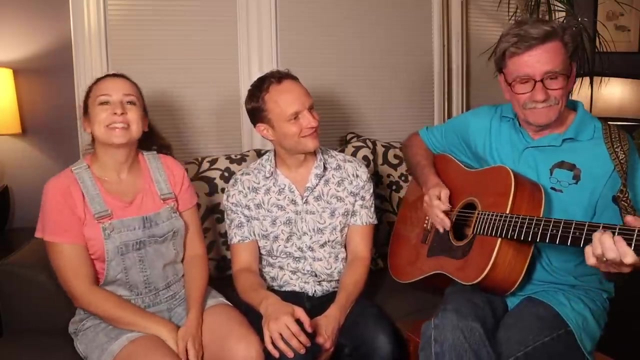 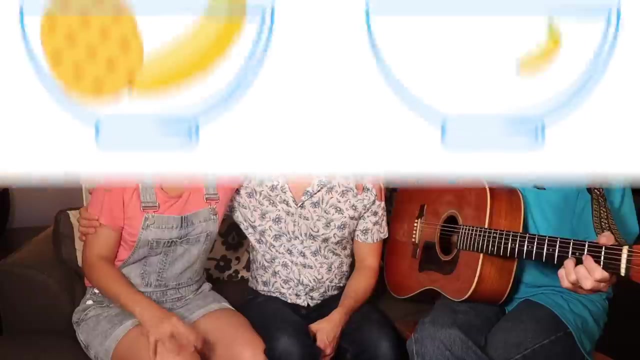 oopals and banunus. I like to eat, eat, eat apples and bananas. I like to eat, eat, eat apples and bananas. Wow, that was so much fun. Thanks guys. Which bowl of fruit has more fruit in it? 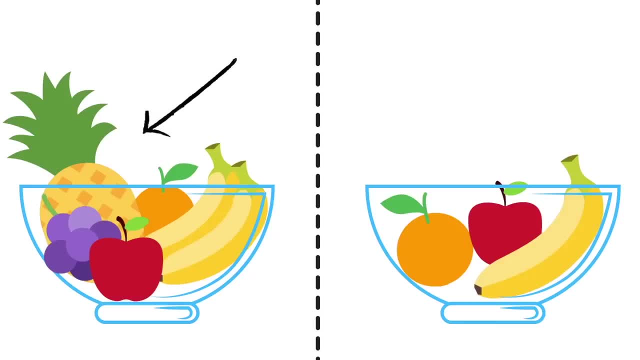 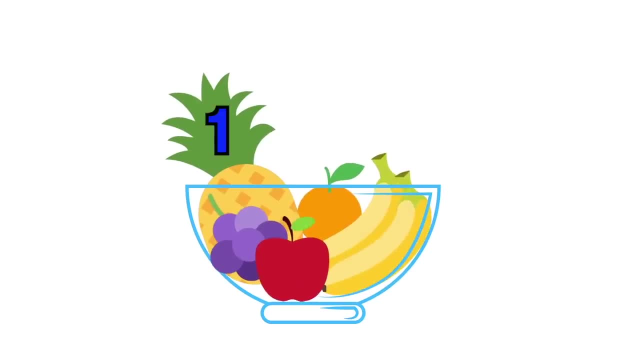 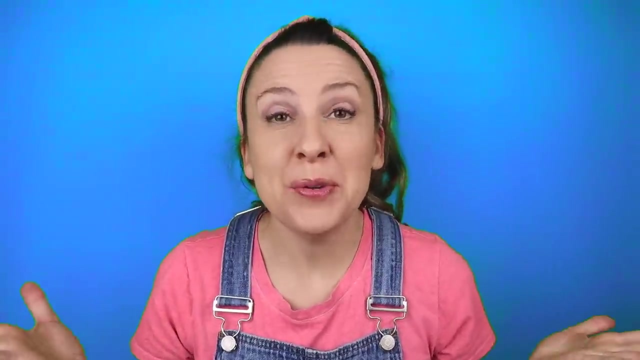 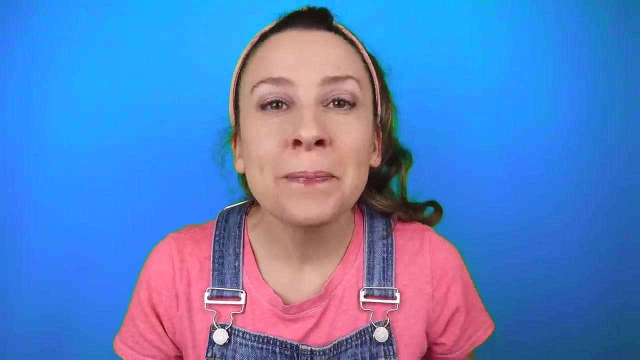 Yeah, this one. This one has more fruit. Let's count the fruit: One, two, three, four, five, six, Six pieces of fruit. What do we do with all this fruit? We eat it. Good job. Can you think of any red food? Hmm … Let's say food and maybe some red food. 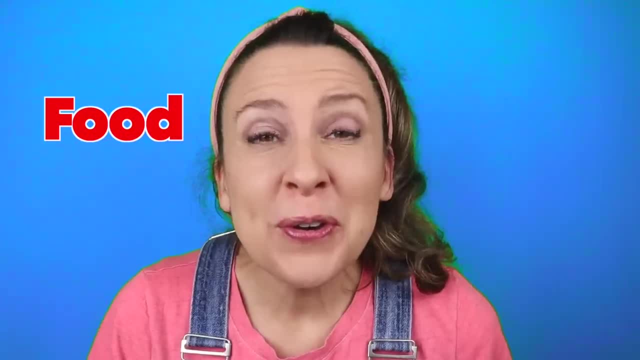 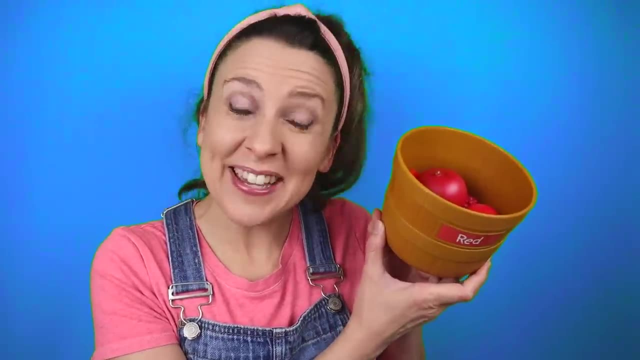 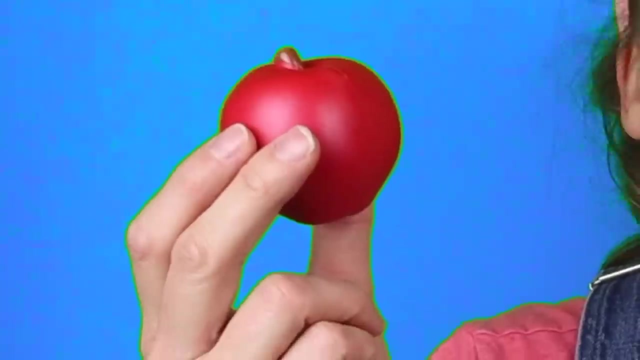 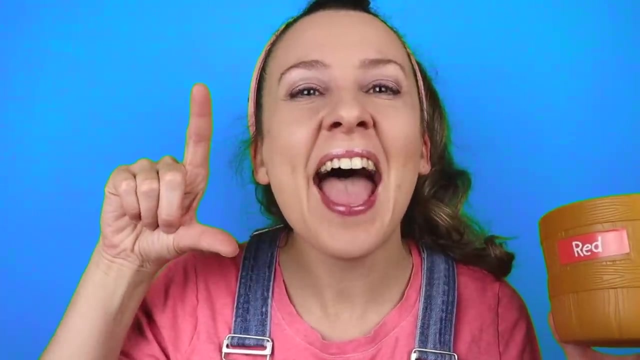 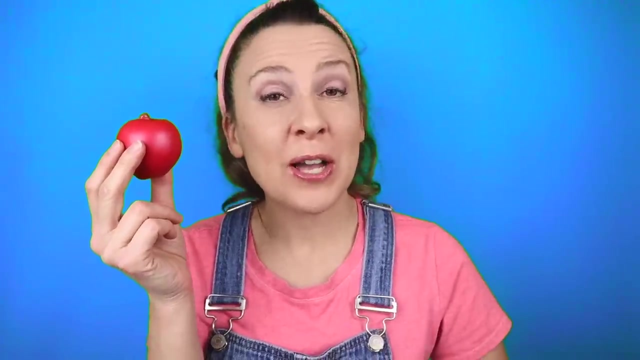 will help. will help. come out. Food, Let's do it louder: Food. Wow, A bucket of red food came out. Let's see what's inside: A red apple. Apple starts with A. Can you do the A sound? Good job? I know a song about an apple. 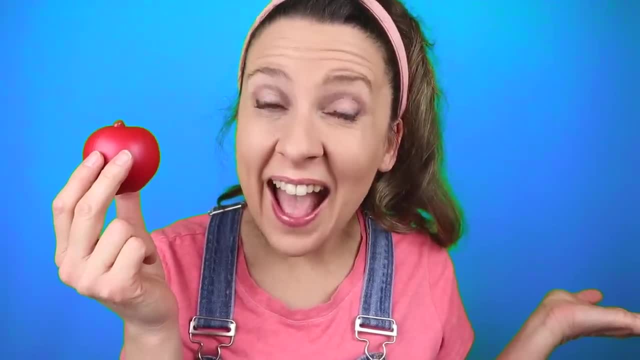 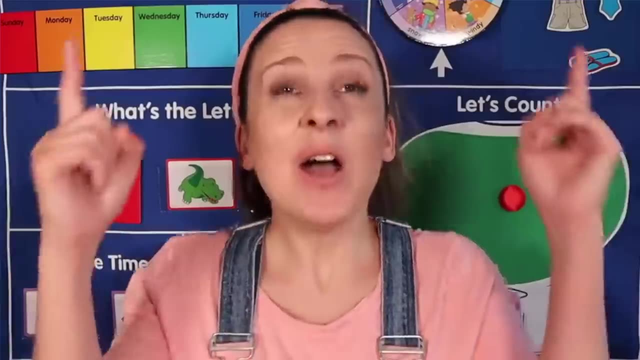 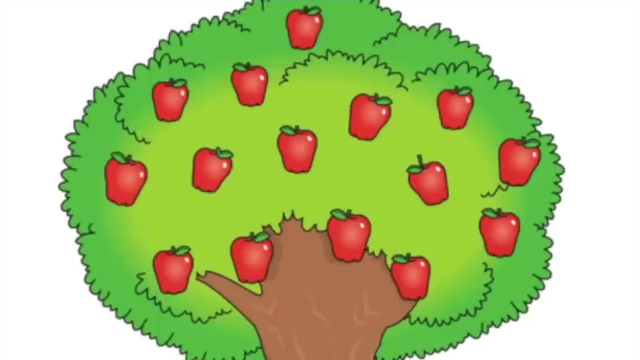 tree. Can you sing it with me? Yeah, Okay, let's sing it. Are you ready? Way up high In the tree, One red apple smiled down at me, So I shook that tree as hard as I could. Down came. 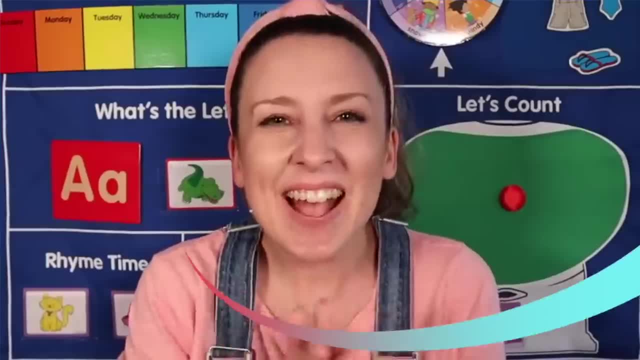 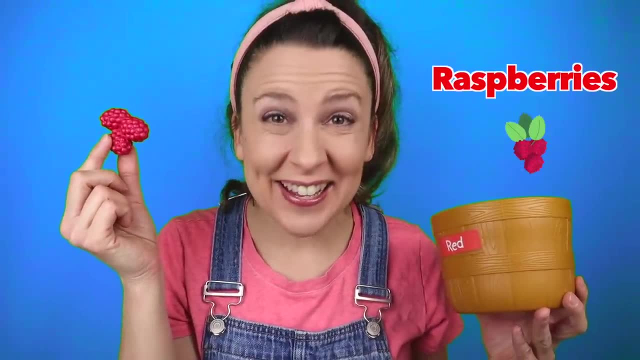 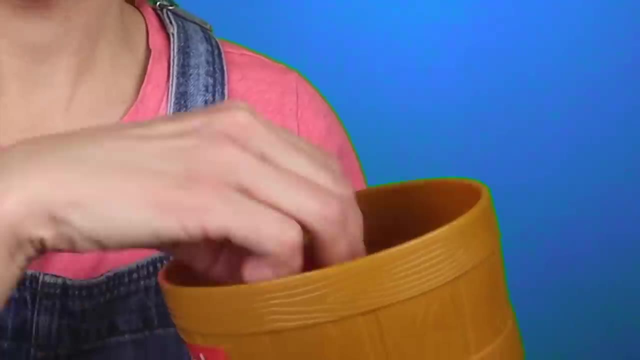 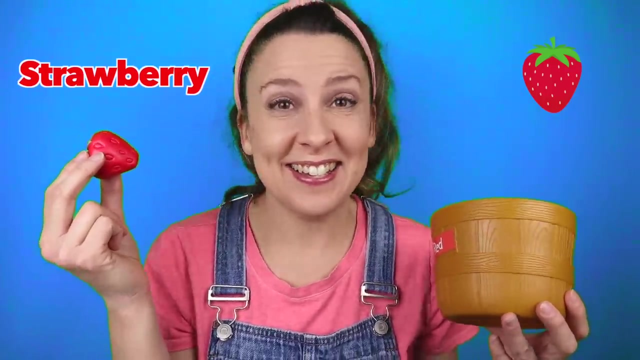 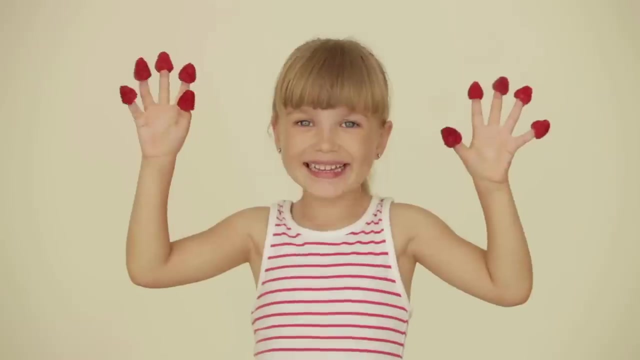 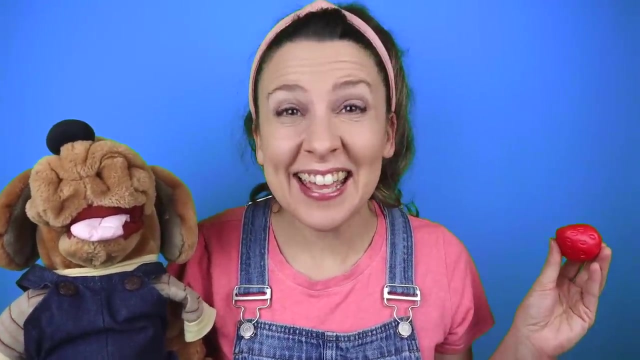 the apple. Good, Great job. Let's see what's inside: Some raspberries, A red tomato, A red strawberry, Mmm. so yummy, Yummy. Let's feed Doggie a strawberry You say eat, and he'll eat it. Eat, Nom, nom, nom, nom, nom, Nom. 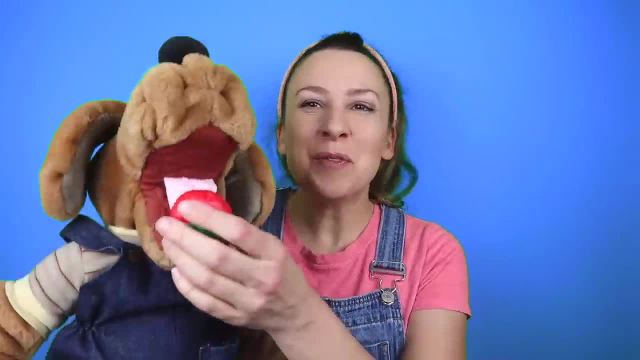 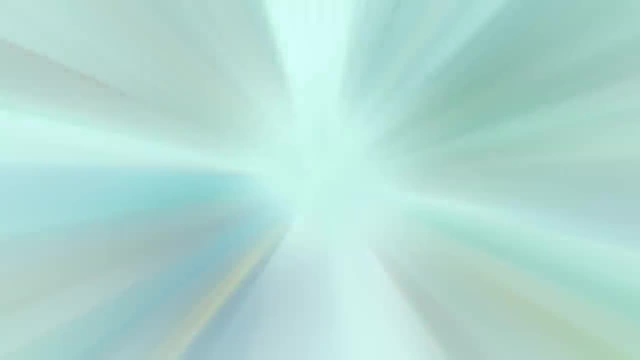 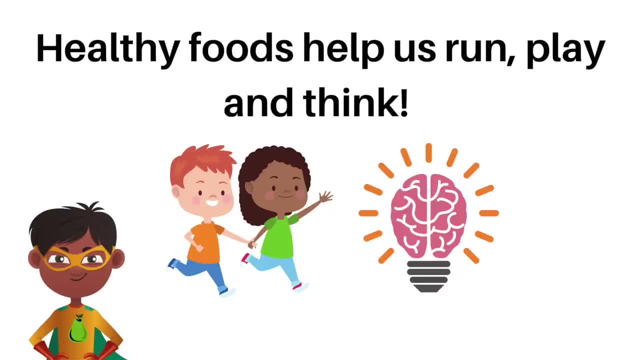 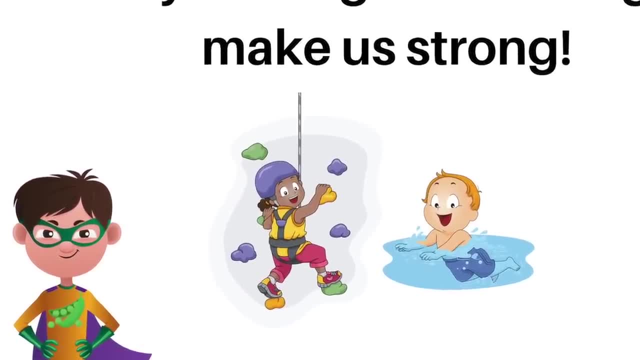 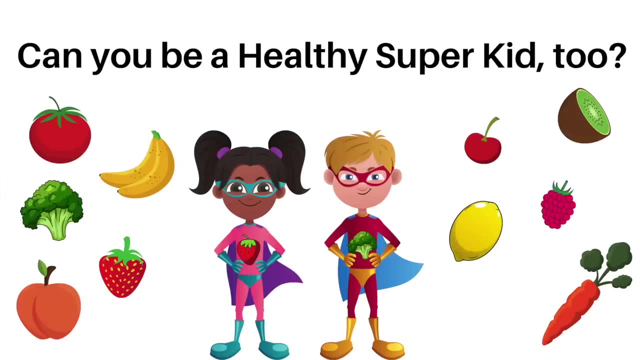 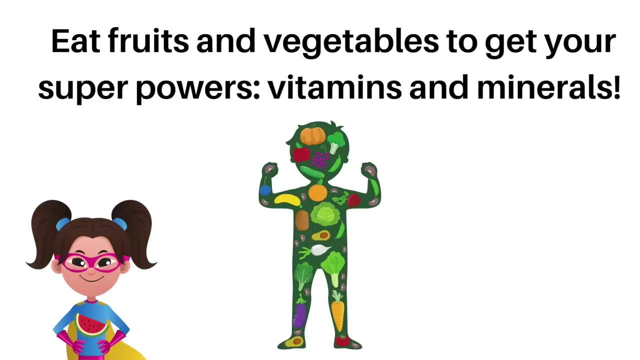 fruits. Healthy foods help us run, play and think. Healthy foods give us energy and make us strong. We eat fruits from the rainbow. Can you be a healthy superkid too? Eat fruits and vegetables to get your superpowers, vitamins and minerals. 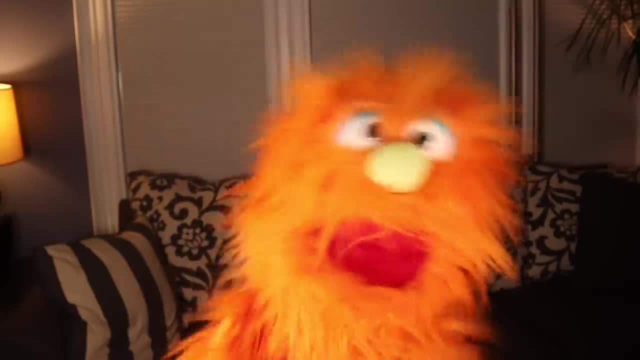 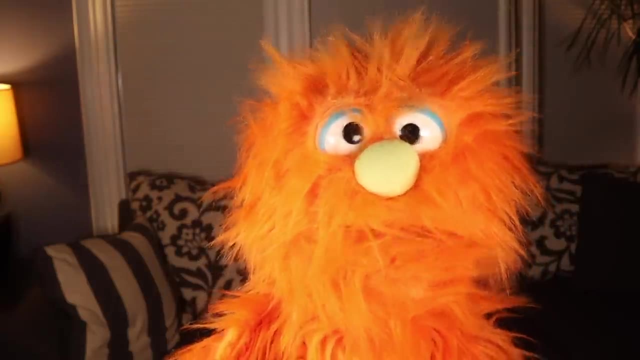 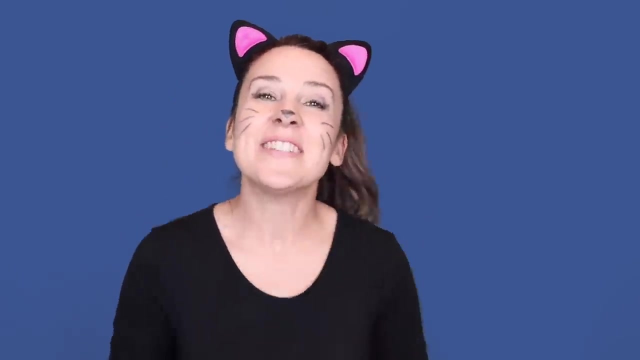 I like to oat, oat, oat, opals and bononos. Opals and bononos- That's funny. For this next song, let's pretend that we keep dropping our pumpkin. You can play along and use a stuffed animal. 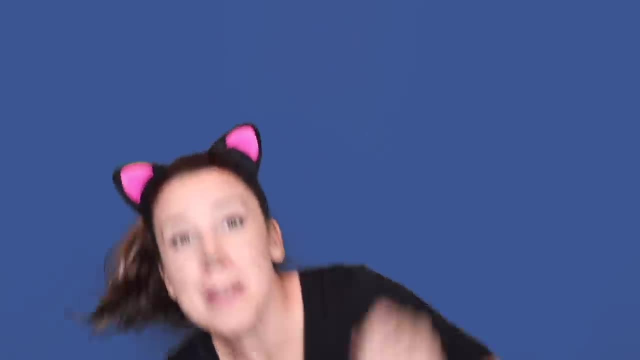 Are you ready? I drop my pumpkin, pick it up, pick it up. I drop my pumpkin, pick it up, pick it up. I drop my pumpkin, pick it up, pick it up And put it on my head. Can you balance it on your head? 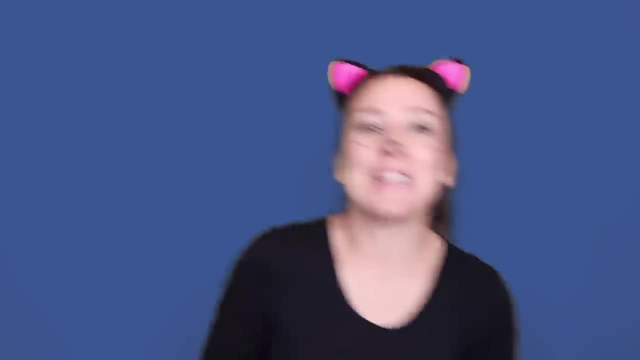 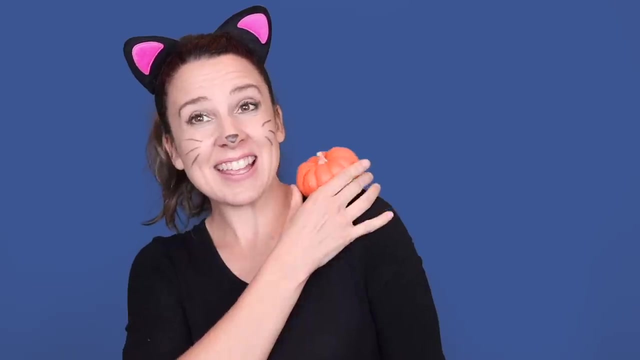 I drop my pumpkin, pick it up, pick it up. I drop my pumpkin, pick it up, pick it up. I drop my pumpkin, pick it up, pick it up And put it on my shoulder. Can you do that? 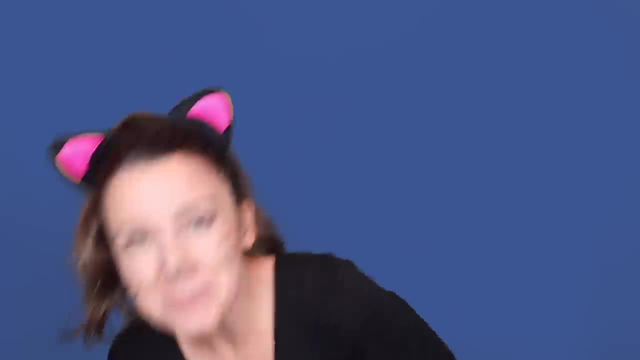 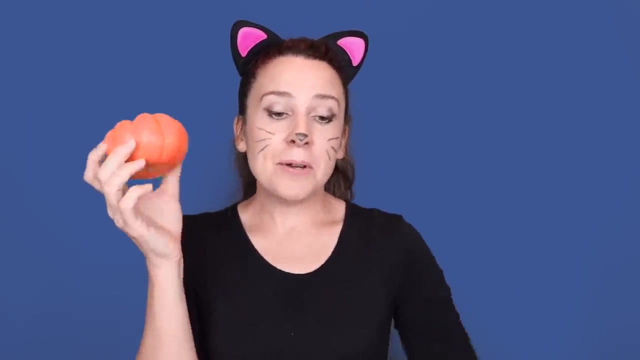 It's hard to balance. I drop my pumpkin, pick it up, pick it up. I drop my pumpkin, pick it up, pick it up. I drop my pumpkin, pick it up, pick it up And put it on my hand. 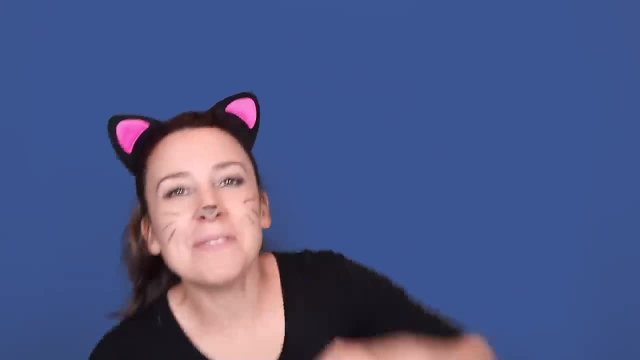 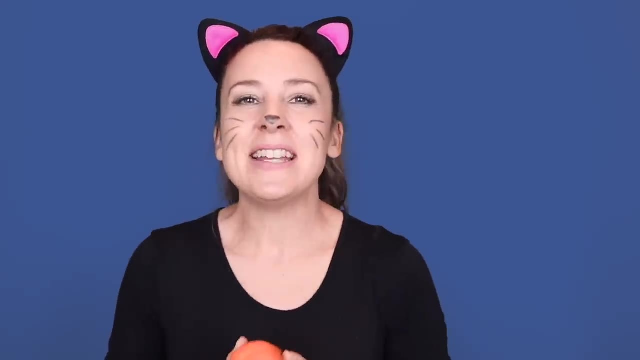 I drop my pumpkin again. I drop my pumpkin, pick it up, pick it up. I drop my pumpkin, pick it up, pick it up. I drop my pumpkin, pick it up, pick it up And put it on my back. 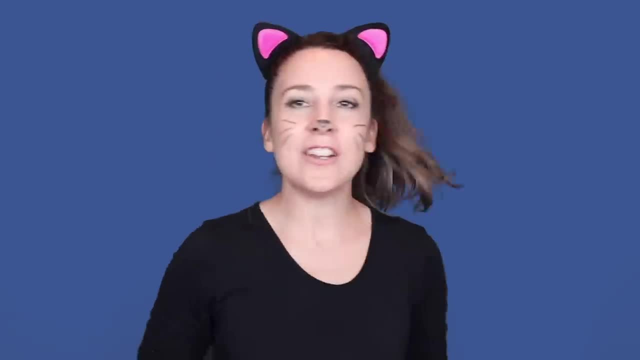 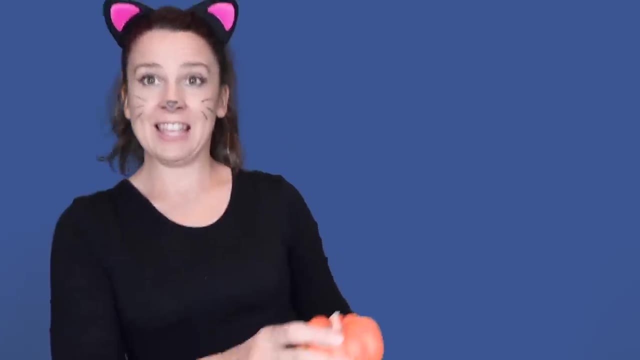 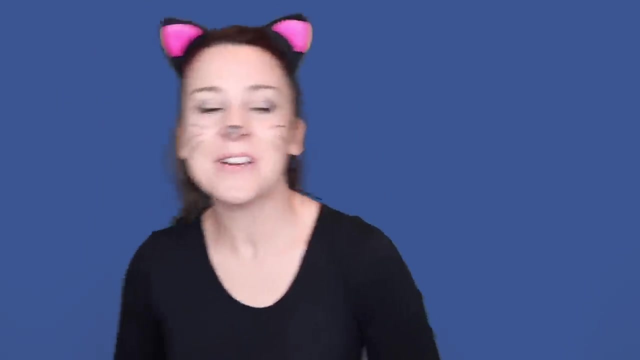 Can you do that So silly? Can you try it on your tummy? Whoa, Whoa. Can you try it on your knee? Can you balance it on your foot? Try that, Good job, Let's sing it one more time. 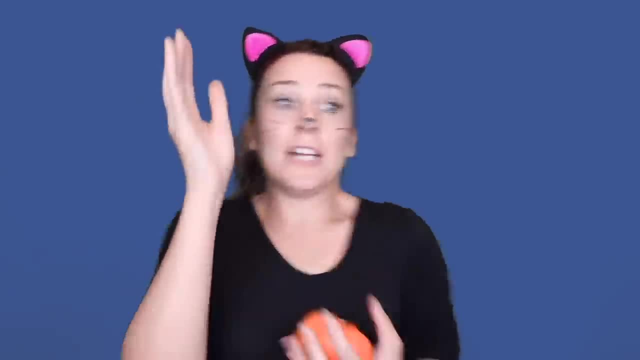 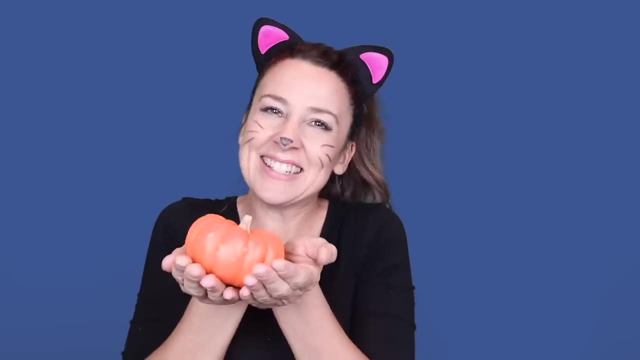 I drop my pumpkin, pick it up, pick it up. I drop my pumpkin, pick it up, pick it up. I drop my pumpkin, pick it up, pick it up And hold it with two hands. That was so much fun. 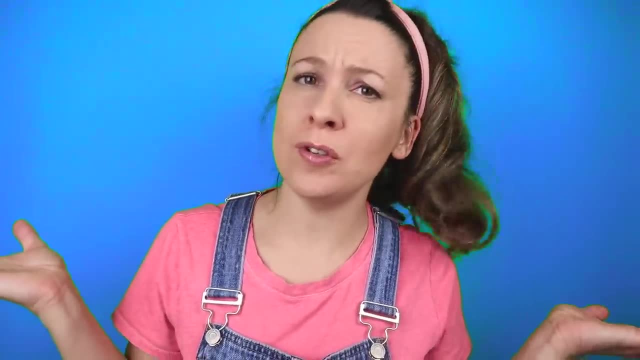 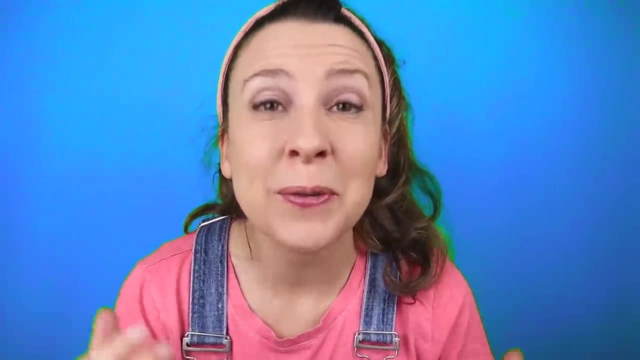 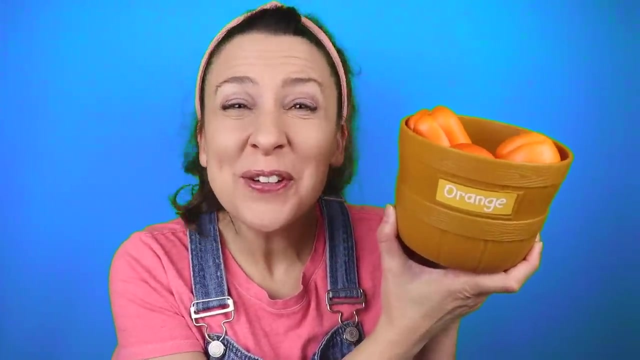 Good job. Can you think of any orange foods? Hmm, You say food and some orange foods will come in. I don't know. I don't know What's going to come out. Food, Food. A bucket of orange foods came out. 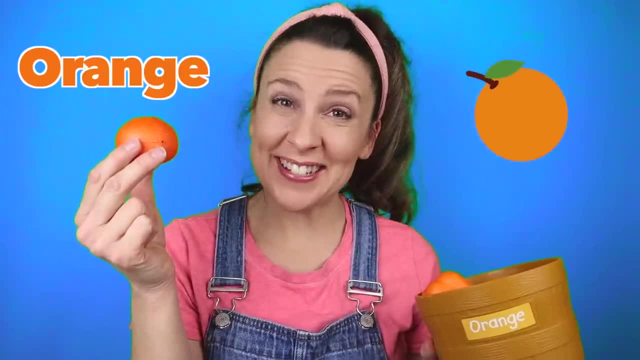 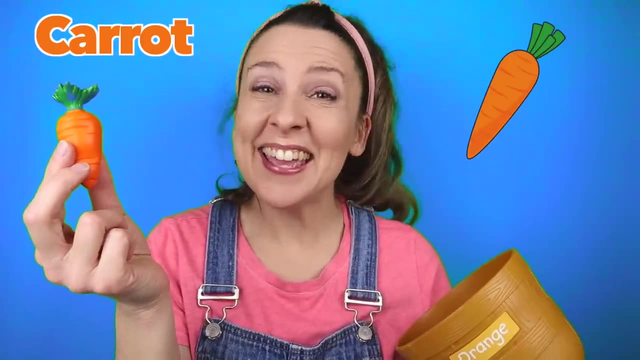 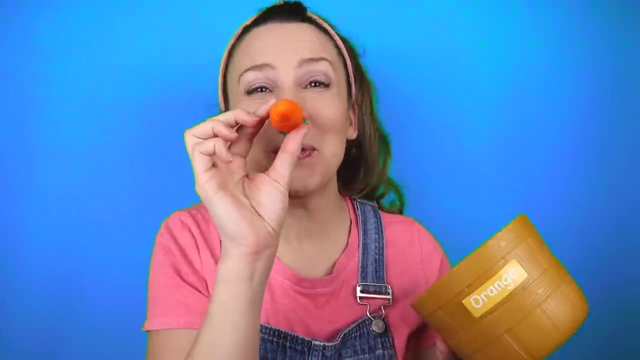 Yay, We have an orange, an orange pepper, an orange carrot. Good job, If you make a snowman, you can use a carrot as the nose. Doo doo, doo, doo, doo. So silly Carrot nose. 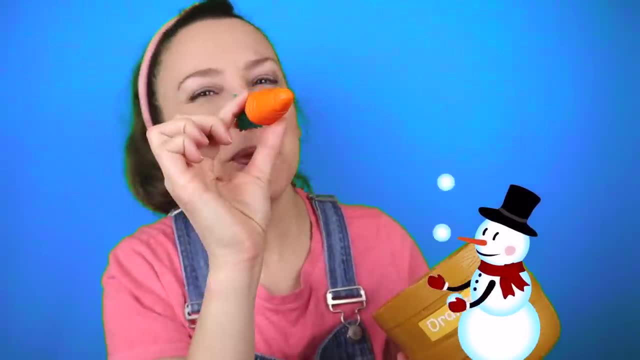 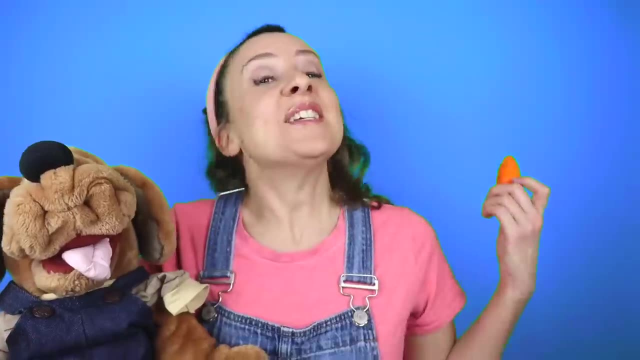 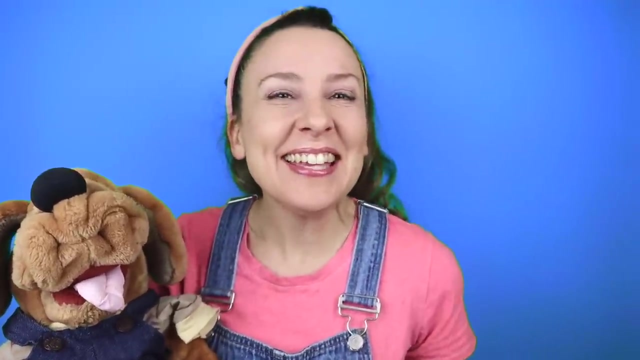 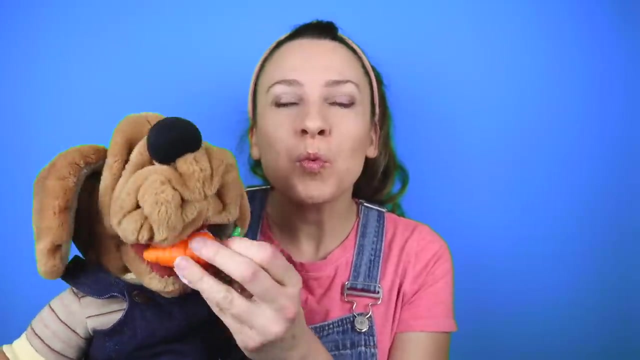 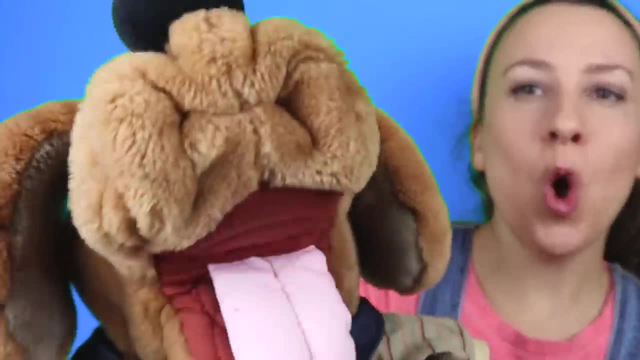 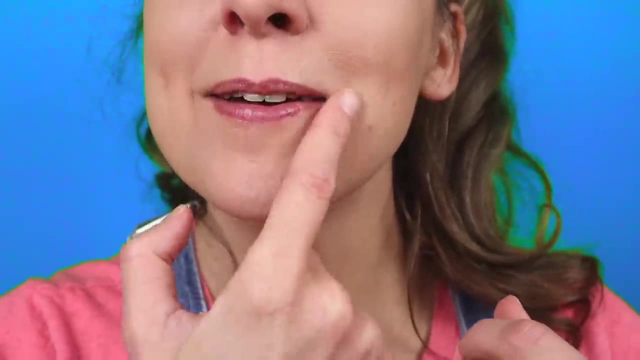 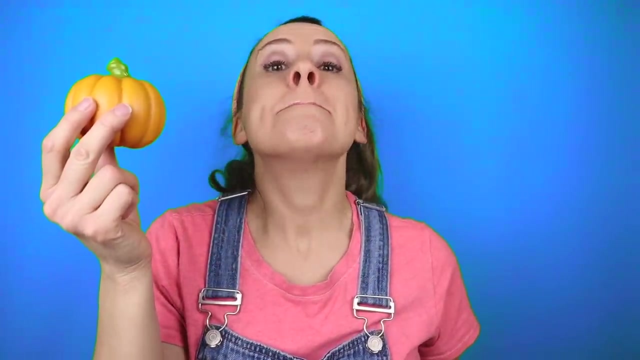 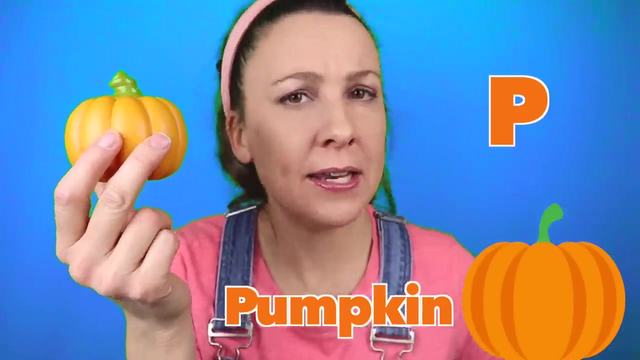 He loves it. om, nom, nom, nom, nom, nom. So yummy, Yummy, can you say that, Yummy, Yummy in my tummy? And an orange pumpkin- wow, Pumpkin begins with P. Can you do the P sound? 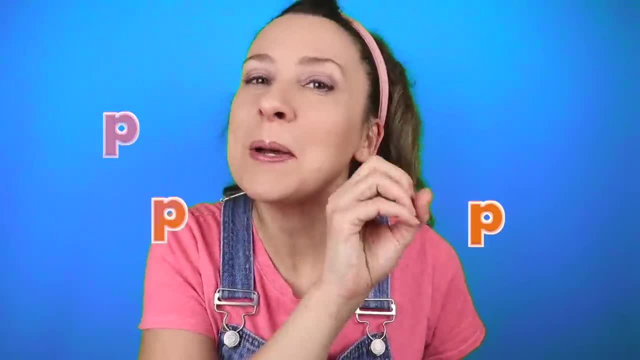 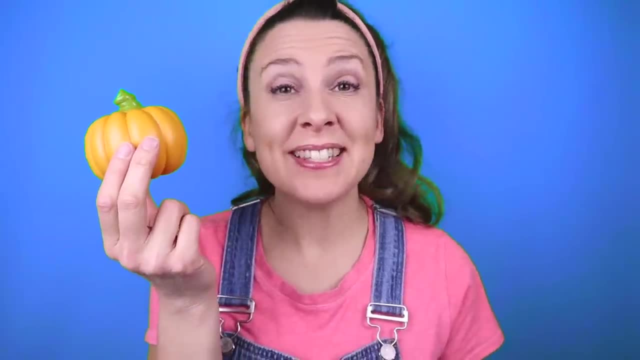 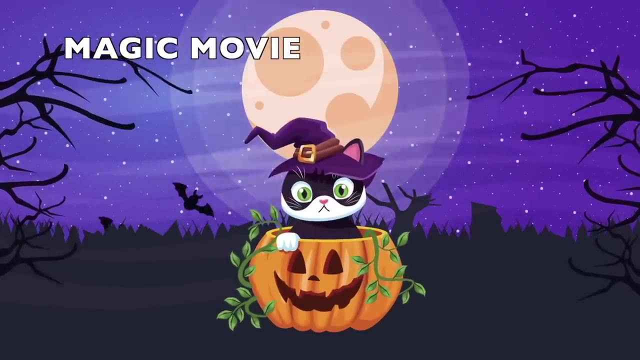 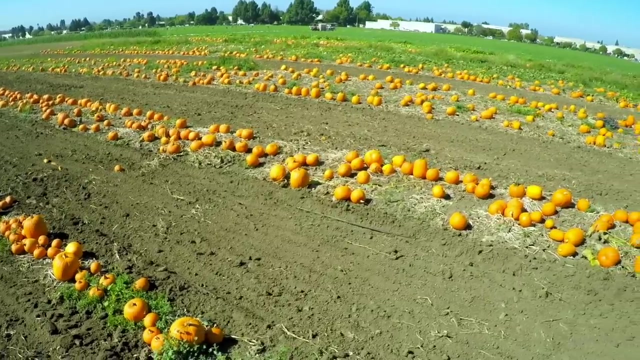 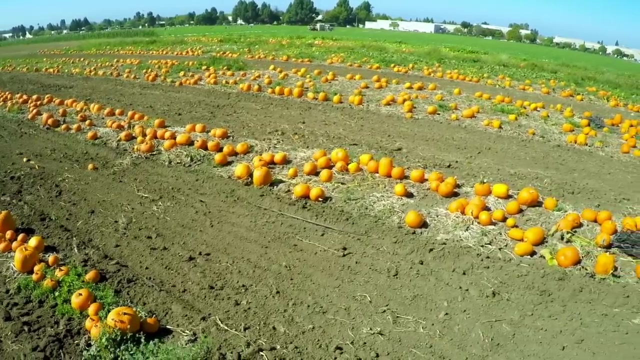 Sometimes on Halloween, we make pumpkins into jack-o'-lanterns. It's so much fun. It's time for a magic movie. Look, We're at the pumpkin patch. I see lots and lots of orange pumpkins, So many pumpkins. 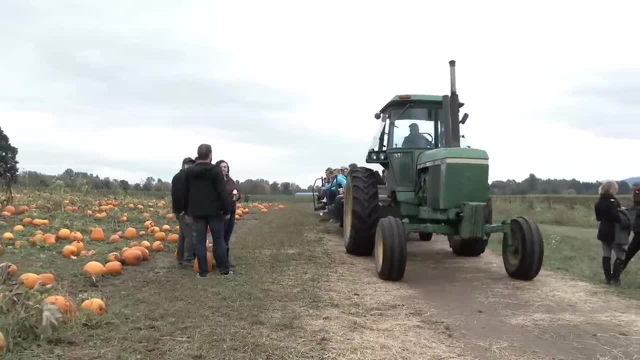 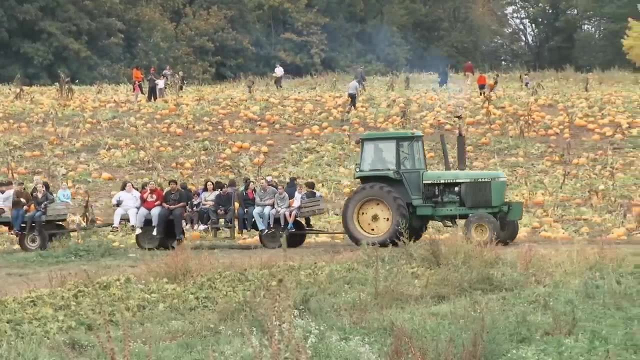 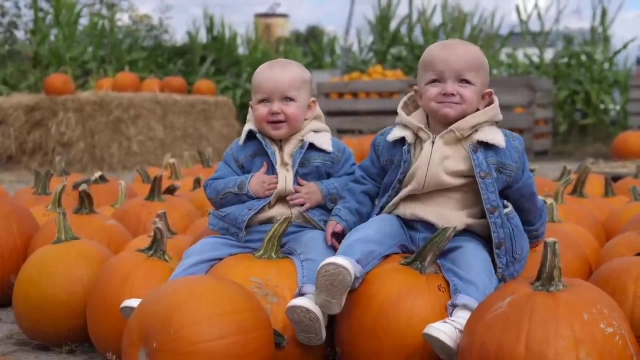 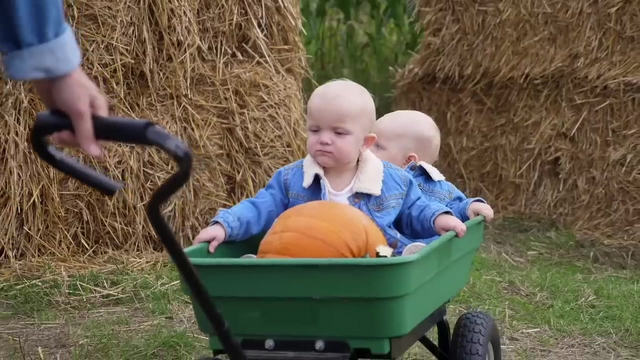 Hey look, a green tractor. There are people riding on the back of the green tractor. This is called a hay ride. Aw, I see two happy babies sitting on the pumpkins. Now the babies are riding in a green wagon. The babies found a pumpkin to take home. It's fun to go to the pumpkin patch and find a. 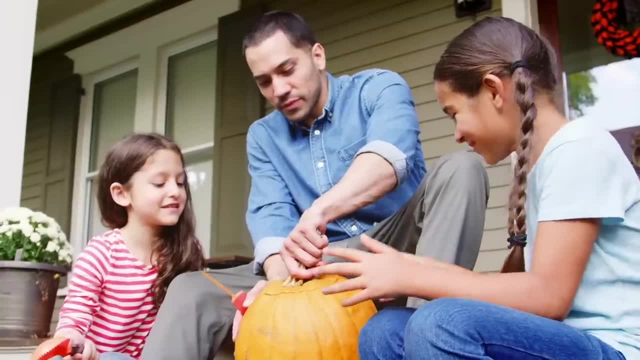 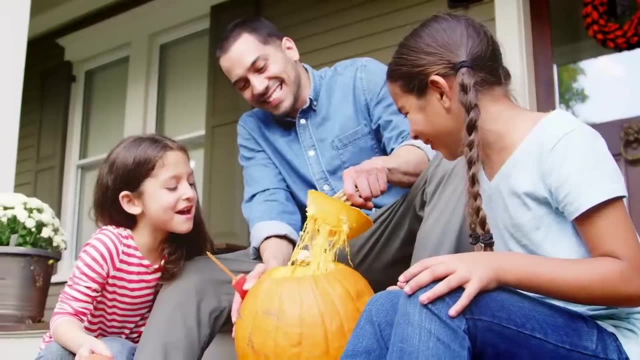 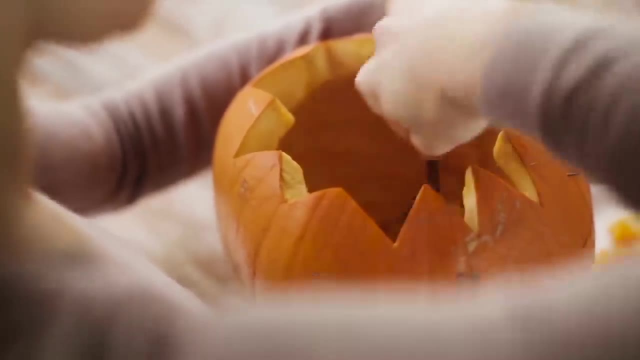 special pumpkin to take home. Now it's time to make the pumpkin into a jack-o'-lantern for Halloween. First you have to cut open the pumpkin- That's only for grown-ups. Then you scoop out the pulp and the seeds. Next you carve a face into the pumpkin. This little girl is carving a pumpkin. 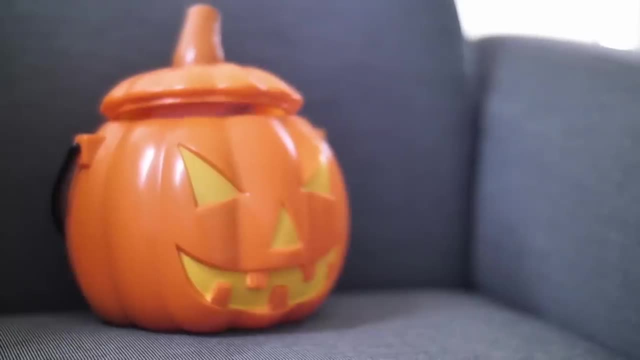 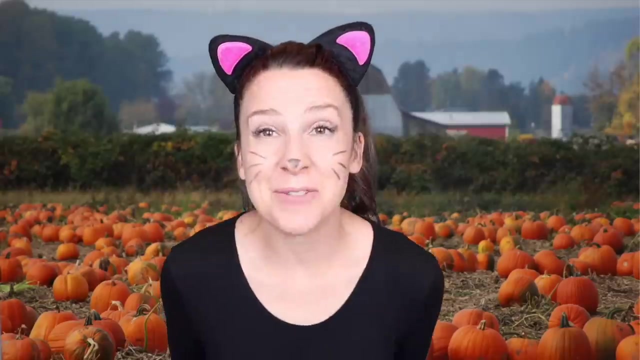 with her grandpa. Finally, we can make the jack-o'-lantern light up. It's so fun to make jack-o'-lanterns for Halloween. Let's pretend we're in a pumpkin patch looking for our pumpkin. Can you walk with me to the beat? 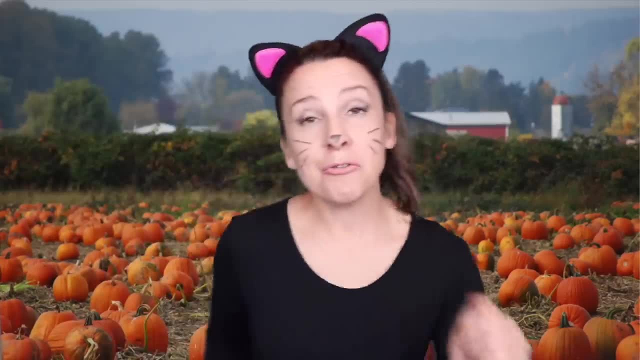 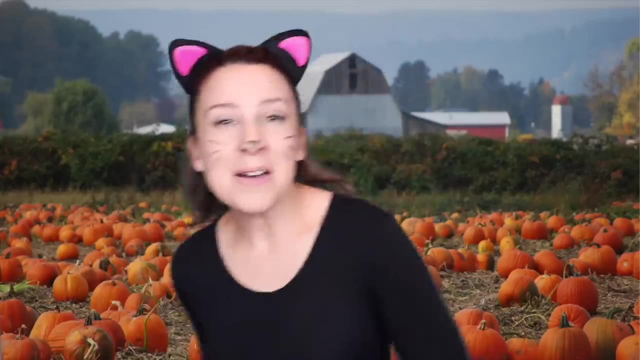 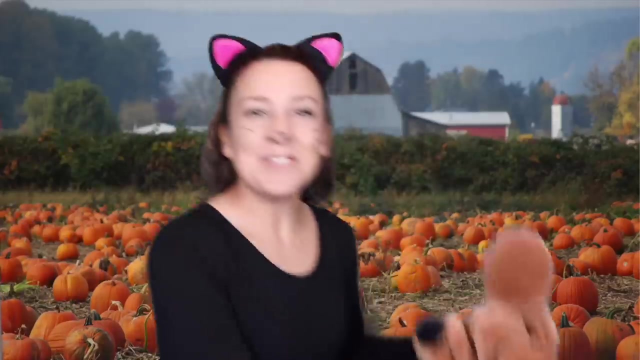 Good job. And when you find the pumpkin, you can dance with your grown-up or someone in your family or a stuffed animal. Are you ready? Pumpkin patch, pumpkin patch. I'm looking for a pumpkin in a pumpkin patch. Here is one one for me. 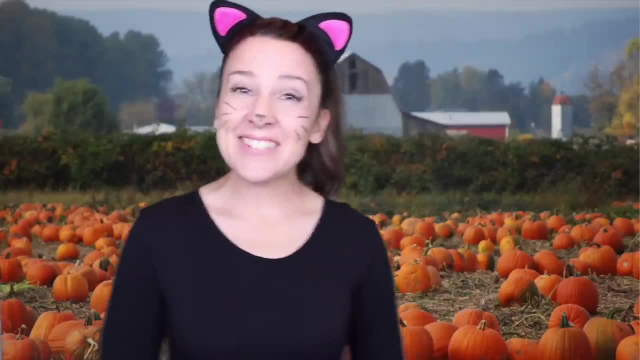 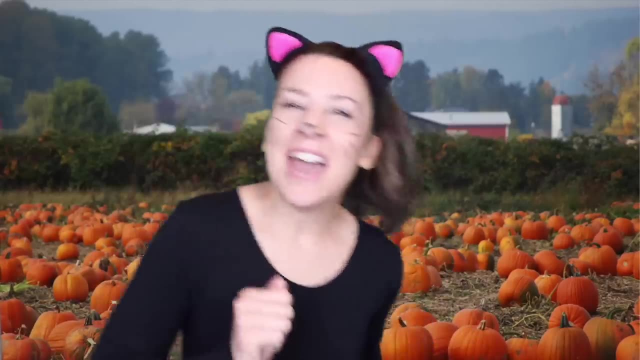 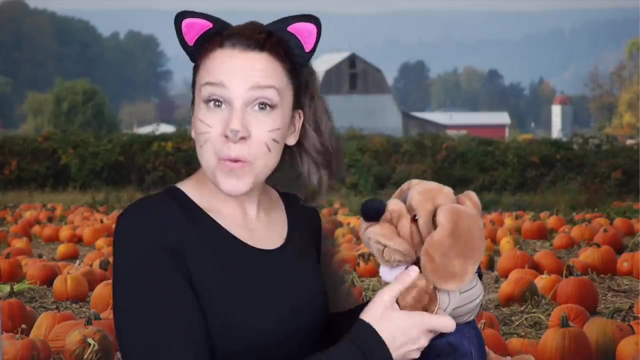 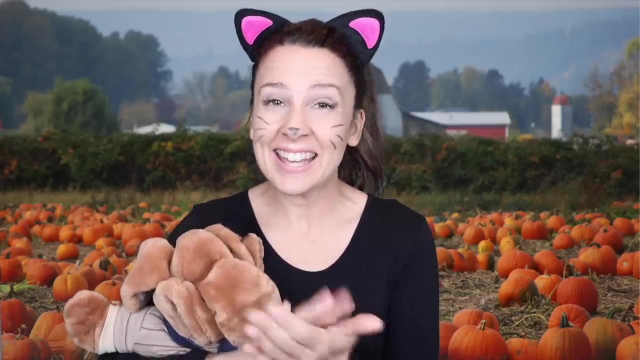 Turn into a jack-o'-lantern for Halloween. That was so much fun. Should we do it again? Should we do it again? Okay, Pumpkin patch, pumpkin patch. I'm looking for a pumpkin in a pumpkin patch. Here is one one for me. Turn into a jack-o'-lantern for Halloween. Yay. 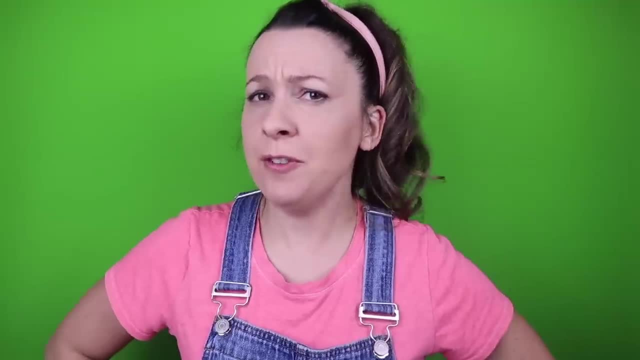 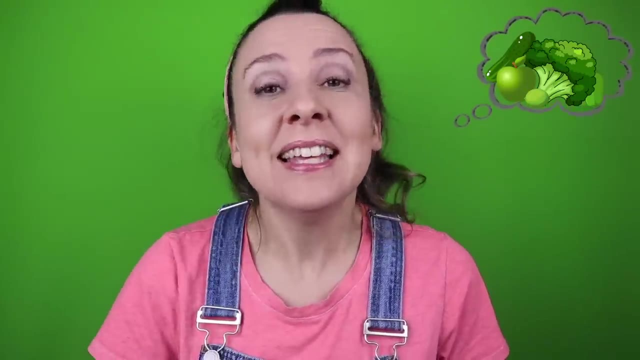 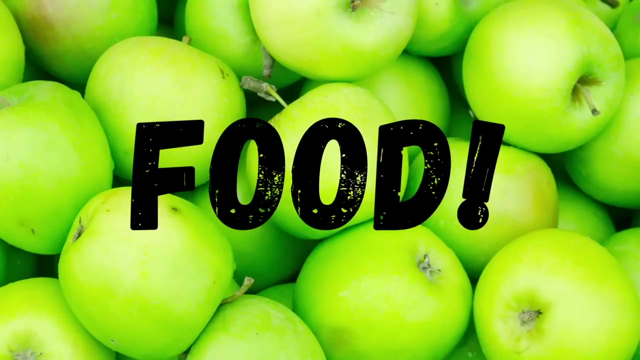 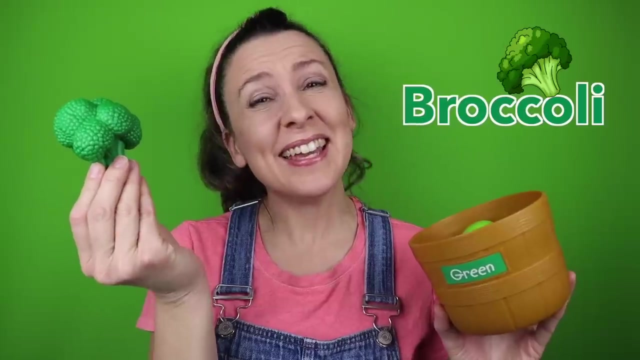 You did a great job. Can you think of any green foods? No, Green foods are so yummy. Hmm, let's say food, and maybe some green foods will come out. Food- Look, It's green broccoli. Yay, I love broccoli, It's one of my favorite foods. 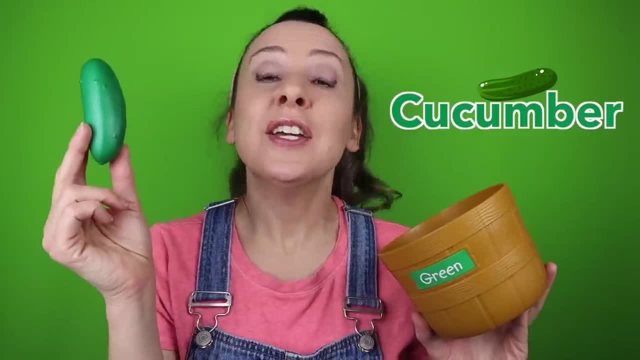 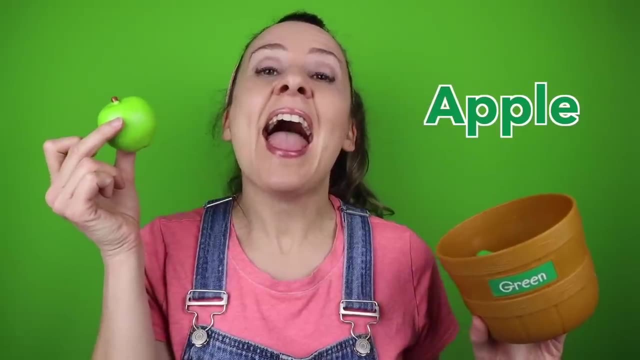 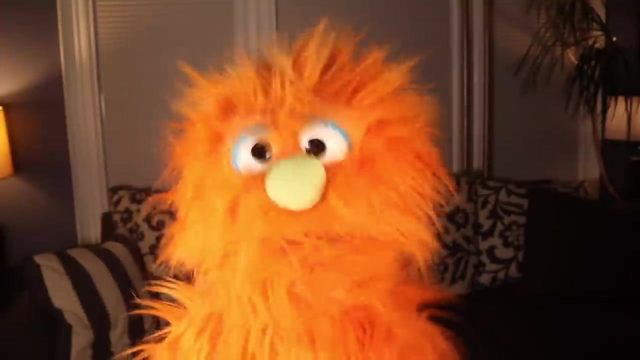 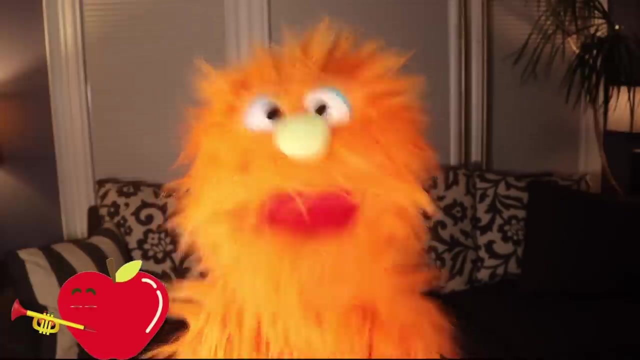 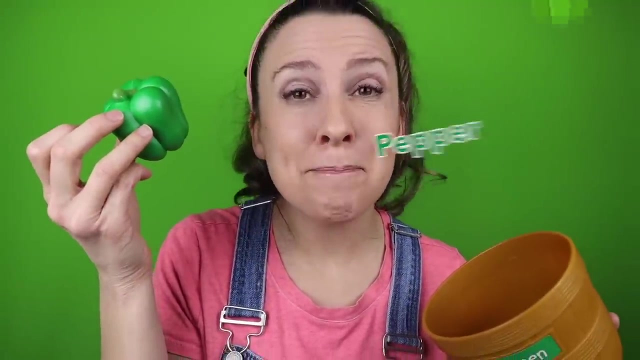 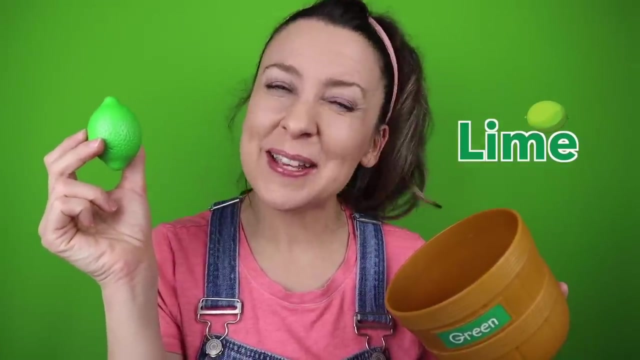 A green cucumber? A green apple? Yeah, Apples can be green too. What do you call an apple that plays the trumpet? A tutti-frutti, Wow, Look. A green pepper, Wow. And a green lime- Awesome. Limes are sour too. 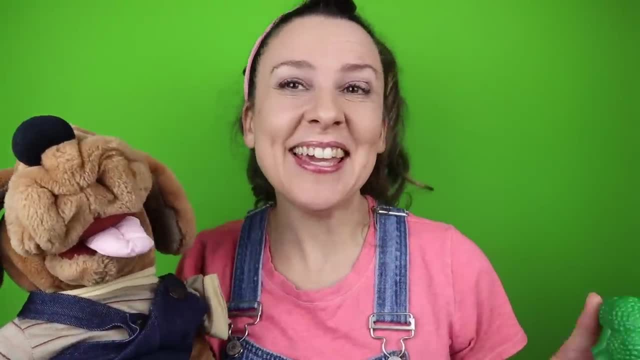 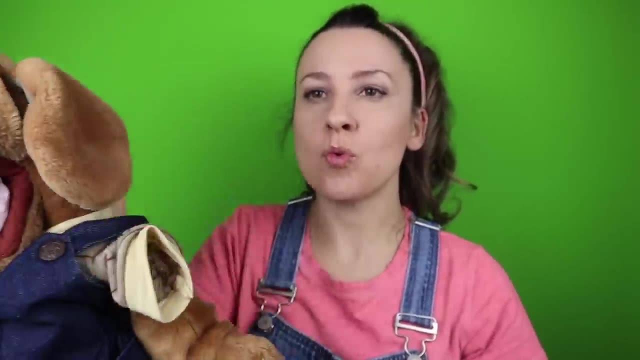 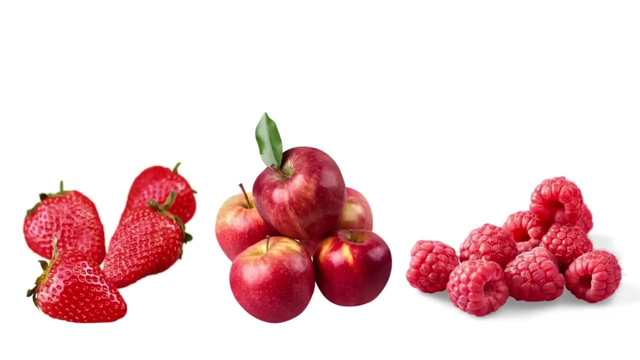 Let's feed doggy some broccoli. Say: eat, Eat, Om nom, nom, nom, nom nom. So yummy, He loved it, Good job. Which group of fruit are the strawberries? Yeah, those are strawberries. What color are all of these fruits? 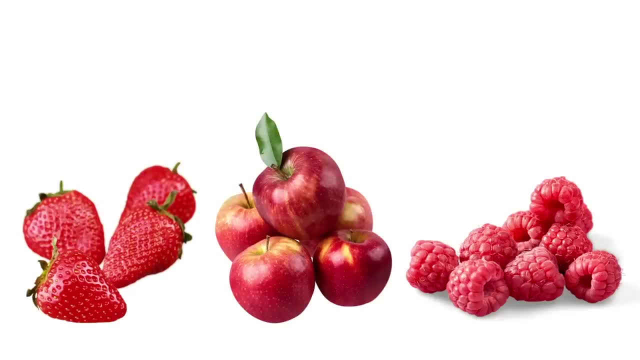 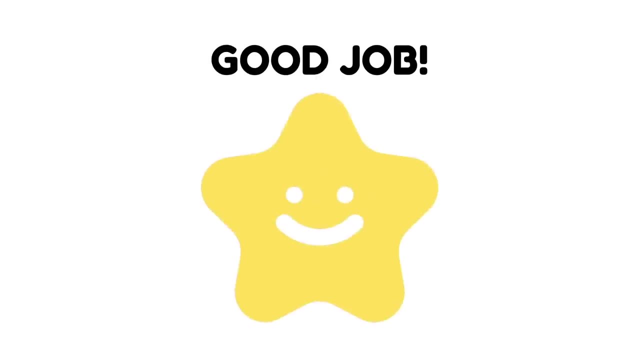 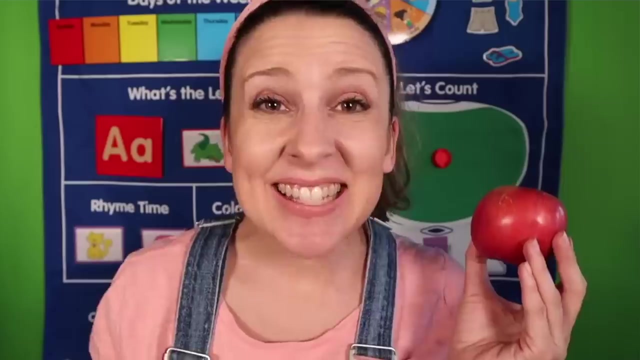 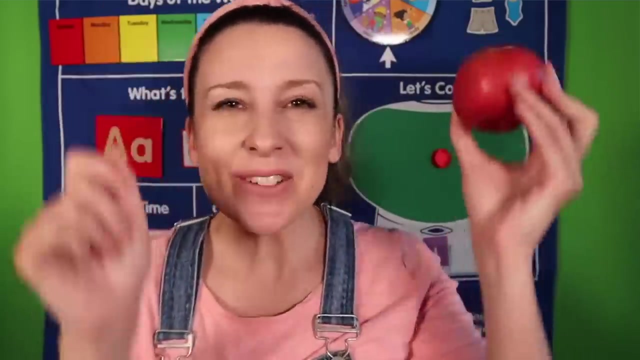 Yeah, they're red Red fruit, Good job. Do you know where apples come from? Trees? That's right. They grow on trees called apple trees And we have to pick them. Pick the apples. Can you pretend to pick an apple off a tree? 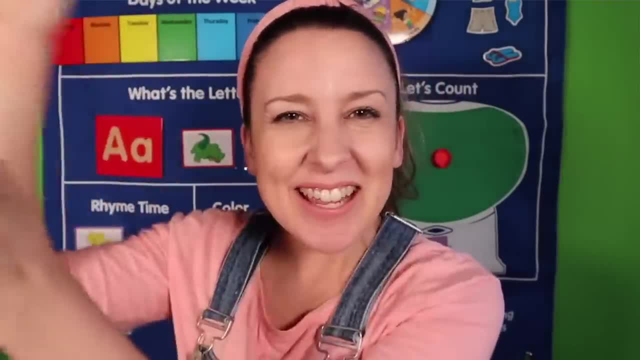 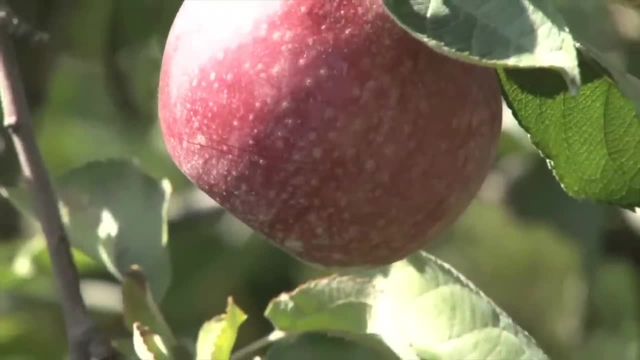 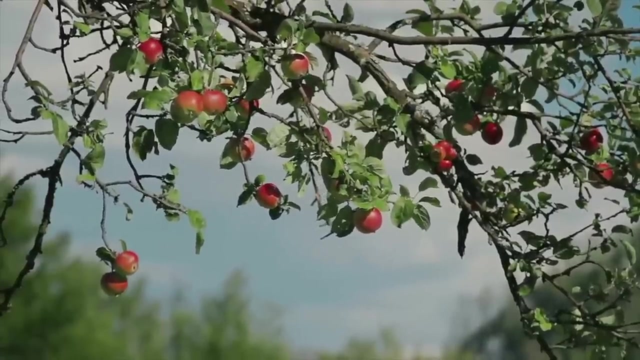 Pick the apple. Pick the apples off trees. Good job pretending. Let's learn more about apples from our magic movie. Here is an apple growing on a tree. Wow, There are many apples on this tree. The man is picking apples. Pick the apple. 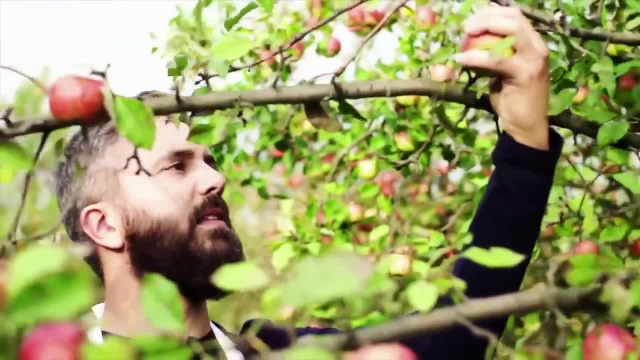 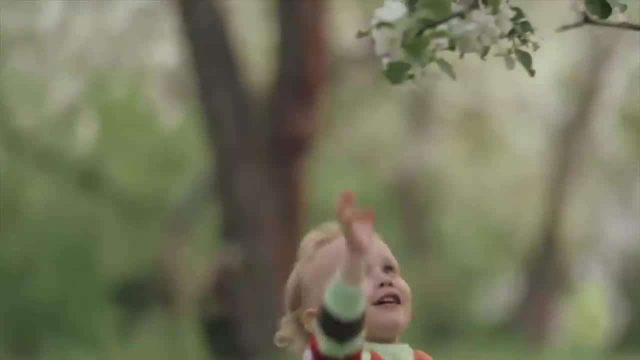 Reach for the apple tree. She is reaching for the apple tree. Look at all the apple trees. A place with many apple trees is called an apple orchard. Can you say orchard, Orchard? The little tree is growing. The apple is growing. 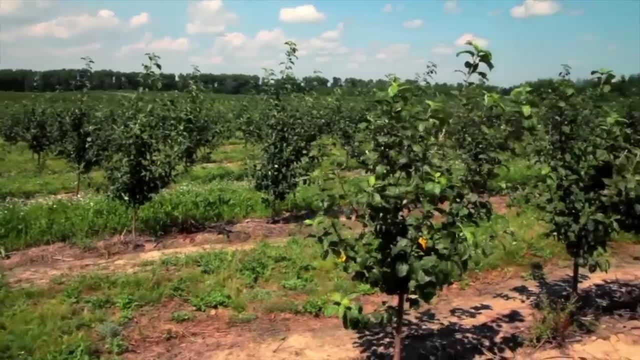 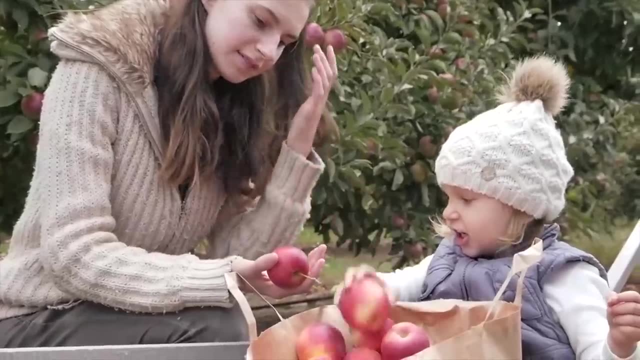 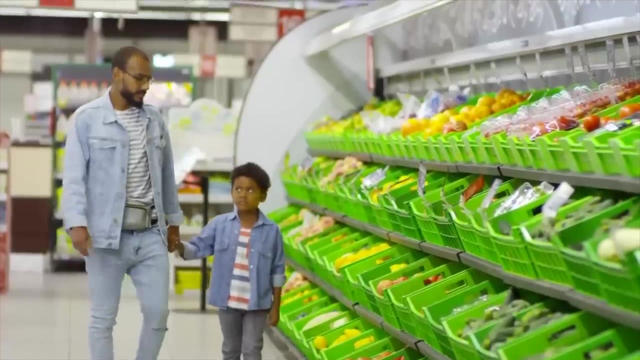 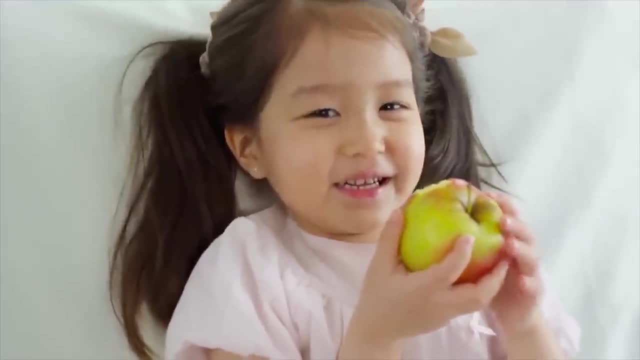 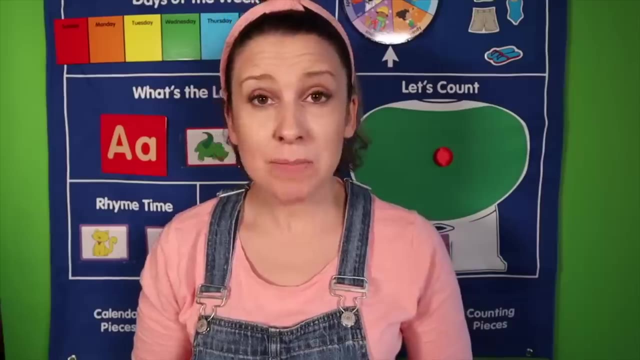 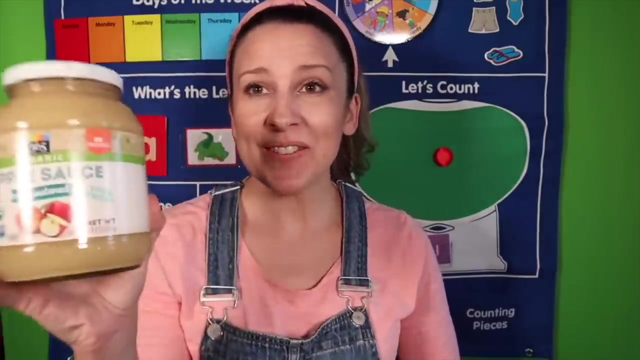 Apples are a fruit that we can eat. Yum, eating the apple. We can eat apples plain. they're so yummy. There's other things we can make out of apples too. Do you know any of them? There's apple. what is this? 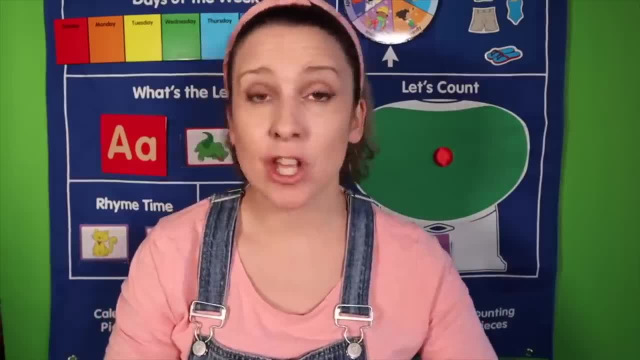 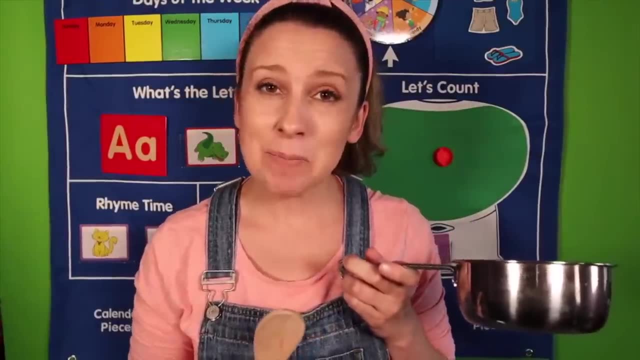 Applesauce: yeah, you can make applesauce. You have to smush the apples to make applesauce and cook them too. Let's pretend we're cooking some apples and making applesauce. Stir the applesauce. can you stir the applesauce? 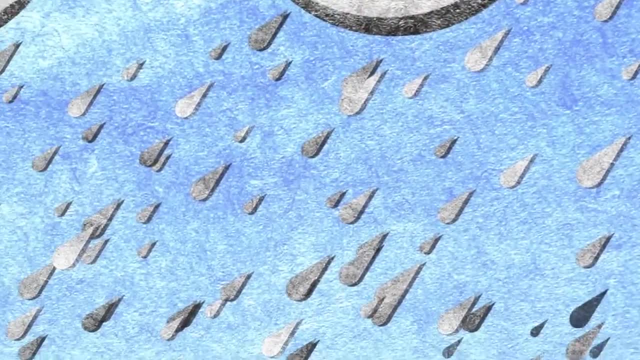 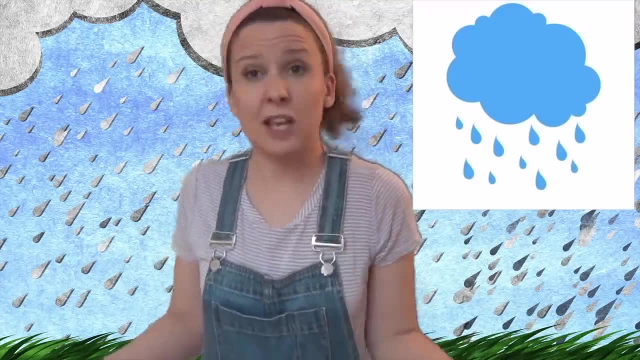 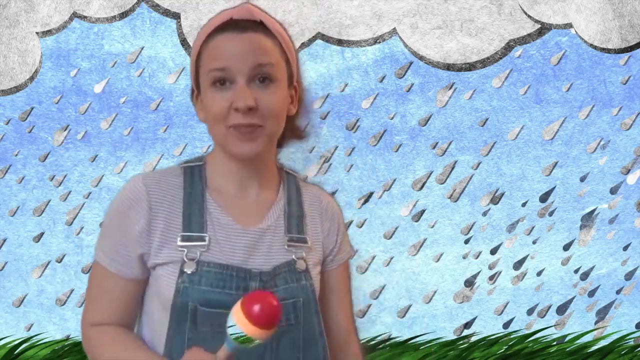 Stir the applesauce- good job. It's starting to rain. Can you help me sing Mr Golden Sun, so the sun will come back out. If you have a shaker at home, it's time to get out your shaker. Oh, Mr Sun. 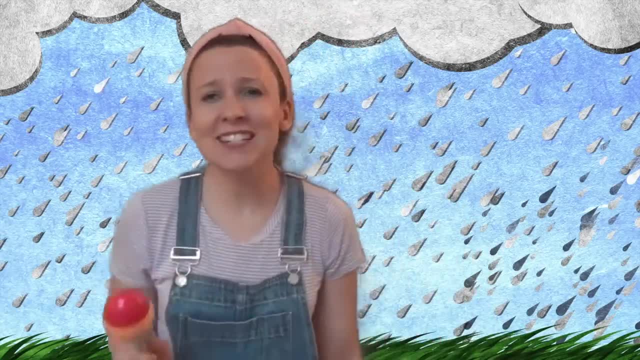 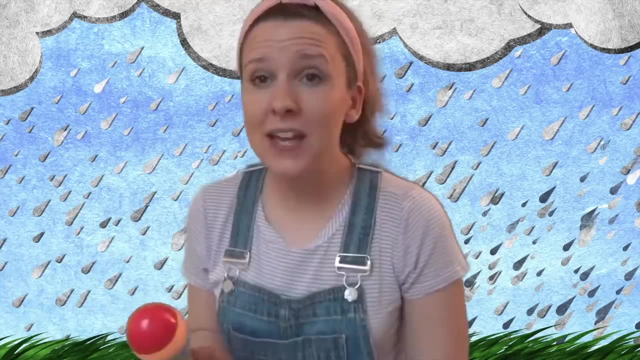 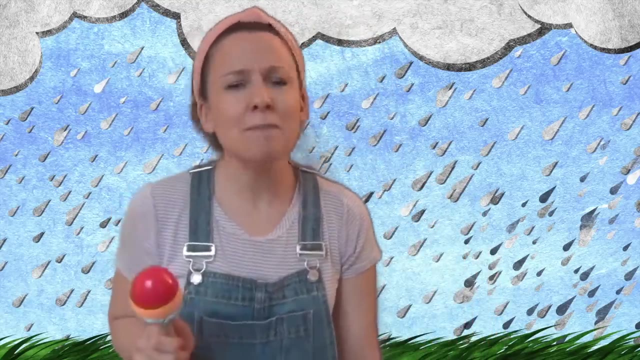 Sun, Mr Golden Sun, Please shine down on me. Oh, Mr Sun Sun, Mr Golden Sun, Hiding behind a tree. These little children are asking you to please come out so we can play with you. Oh, Mr Sun. 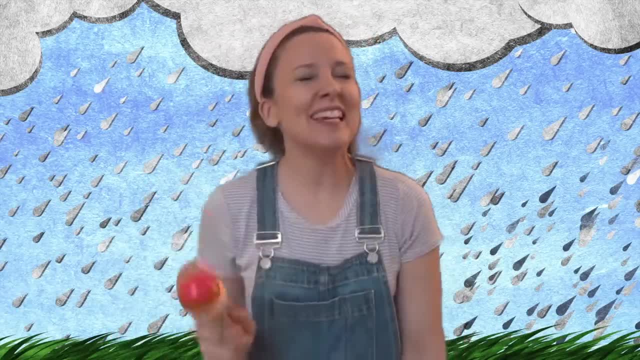 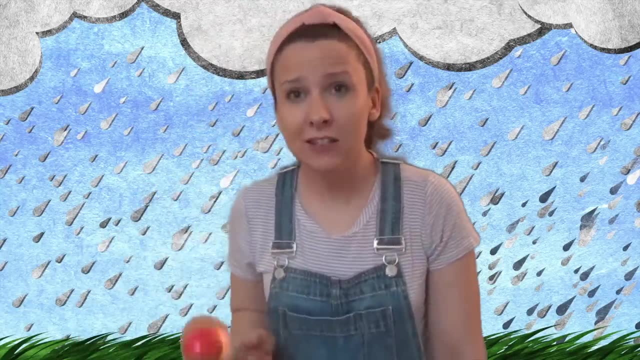 Sun, Mr Golden Sun, please shine down on me. Wow, The sun is coming out, but it's still a little cloudy. Let's sing it again and see if the sun comes out. Are you ready? Okay, get your shaker. 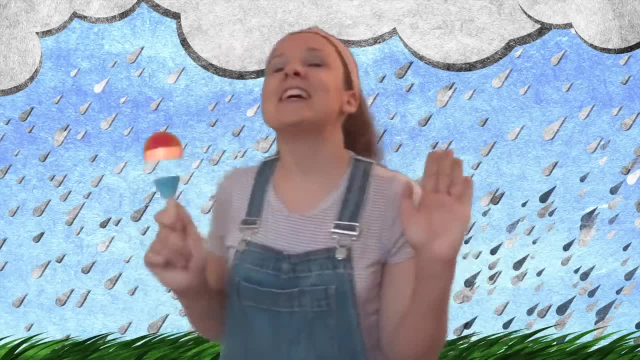 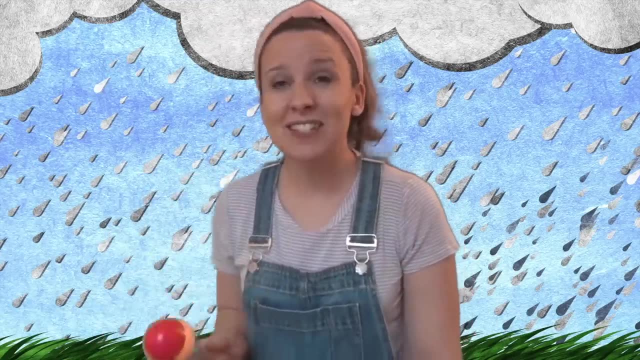 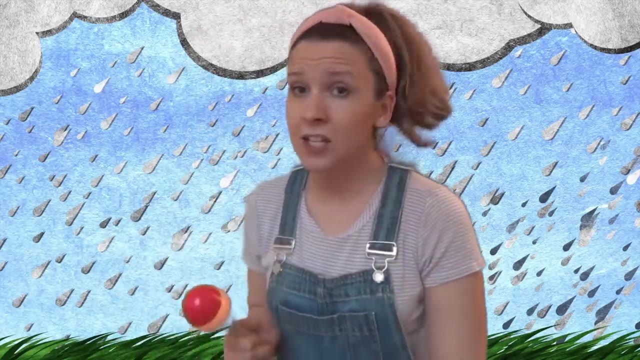 Oh, Mr Sun Sun, Mr Golden Sun, please shine down on me. Oh, Mr Sun Sun, Mr Golden Sun, hiding behind a tree, These little children are asking you to please come out so we can play with you. 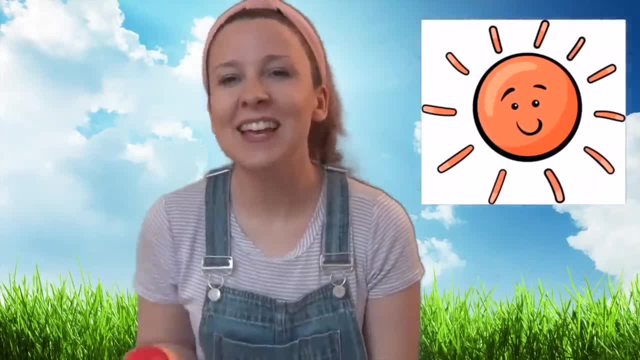 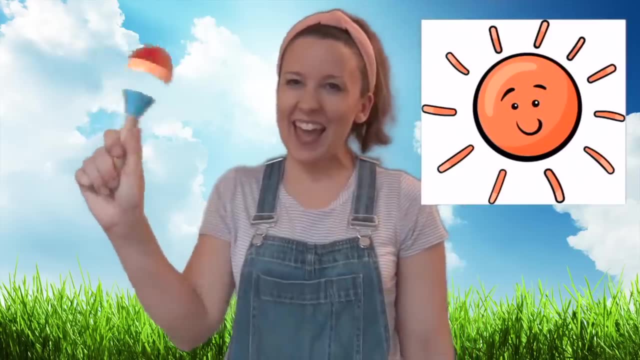 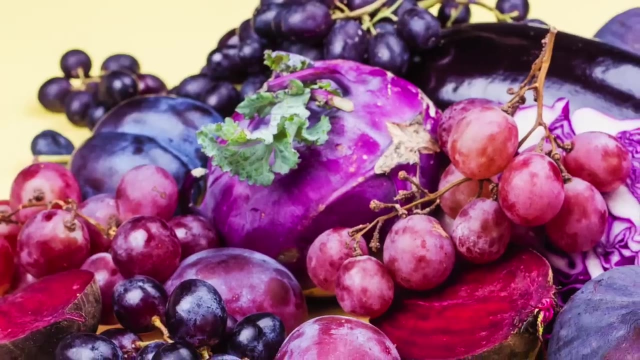 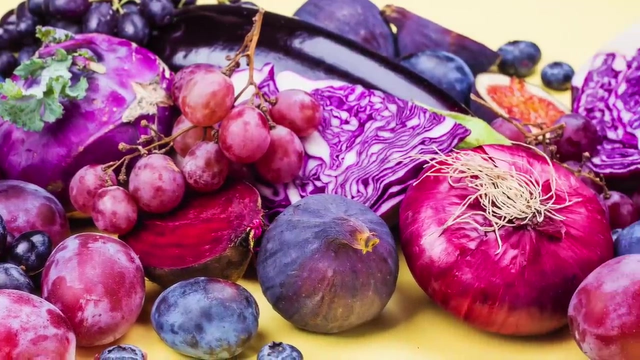 Oh, Mr Sun Sun, Mr Golden Sun, please shine down on me. Yay, The sun came out. Oh, it's so warm now. Thank you so much. Can you think of any purple foods? Hmm, let's say food, and maybe some purple foods will come out. 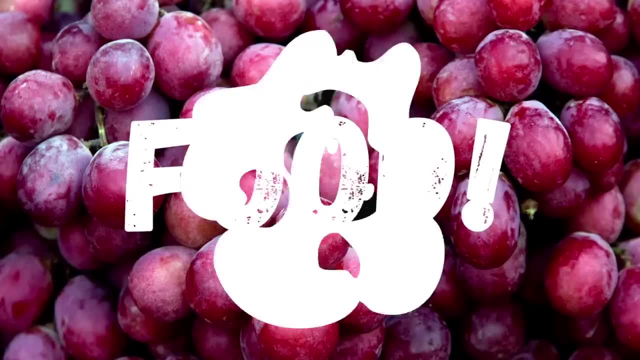 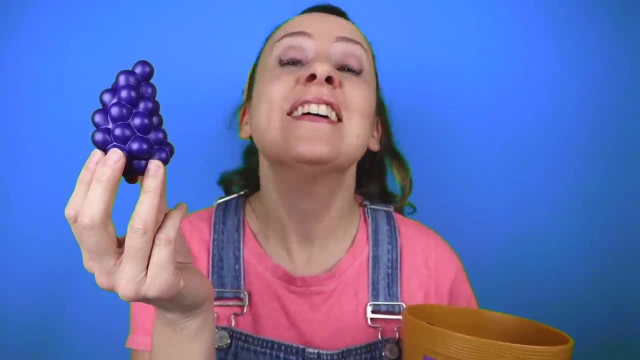 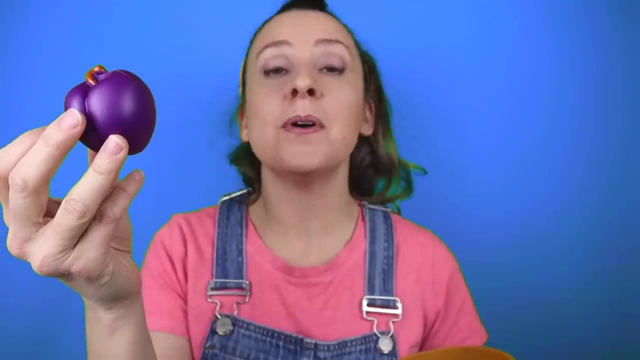 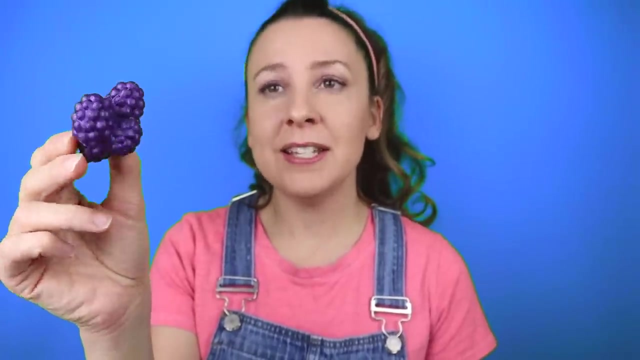 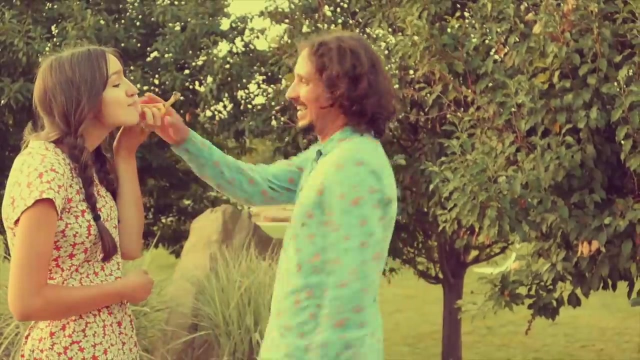 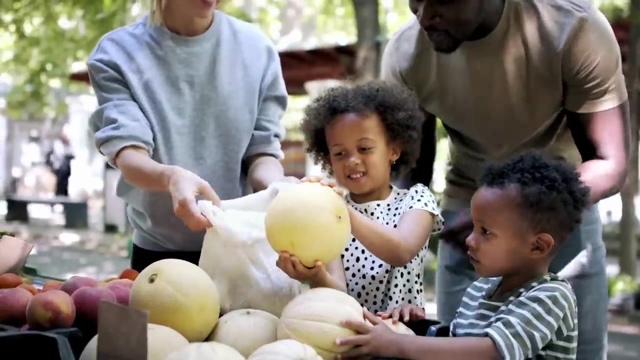 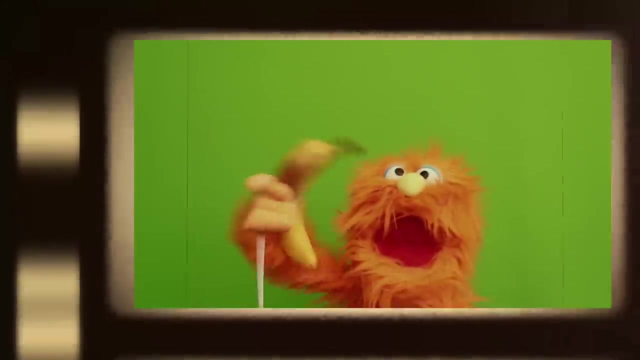 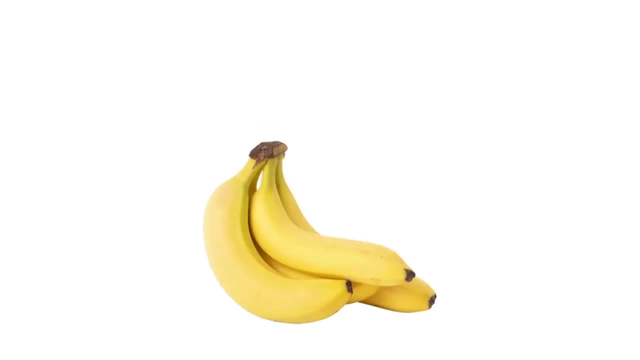 Food. You said food and the purple food came out. Wow, It's purple grapes. Wow, This is a purple eggplant, A purple apple, A purple plum, A purple onion And some blackberries that are purple. What color are these bananas? 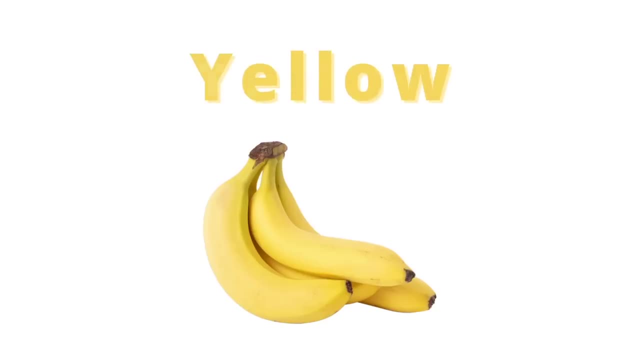 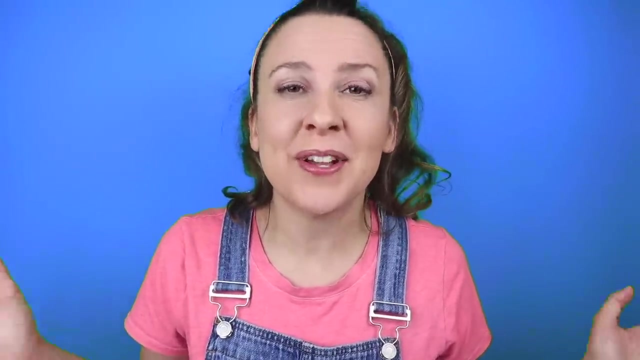 Yeah, they're yellow. Which fruit shares a name with a color? I'll give you a clue: Yeah, It's an orange orange, Good job. One of my favorite foods is blue. Can you guess what it is? Hmm, Can you guess? 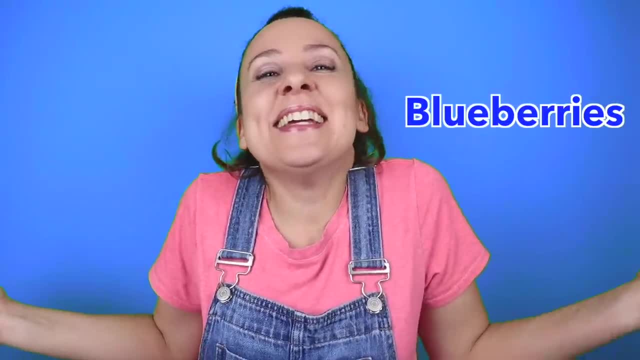 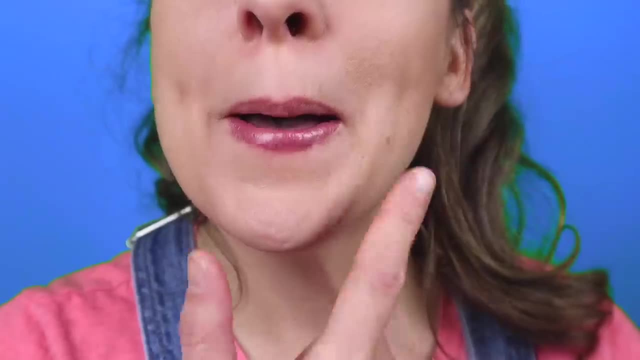 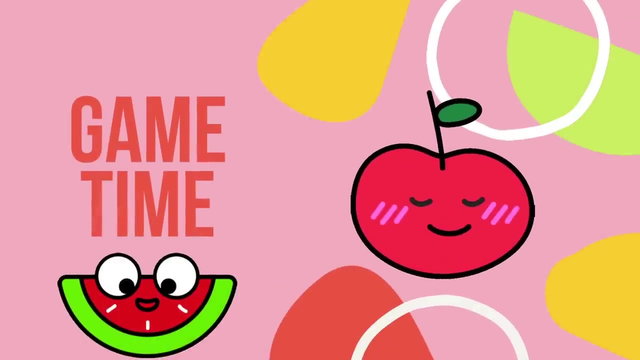 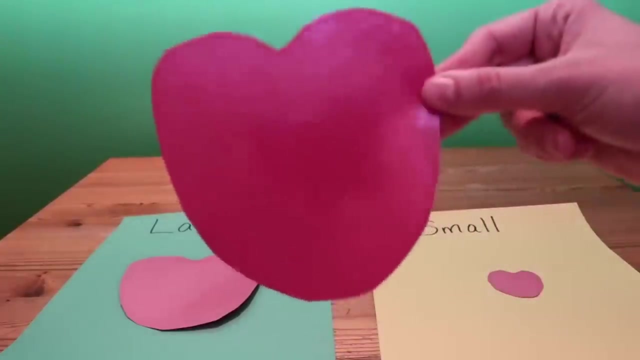 Yeah, Blueberries, Yummy in my tummy, Mmm Yummy. It's time for a super fun game. Let's sort these apples by size. Okay, Does this apple go with large or small? Large, Good job. 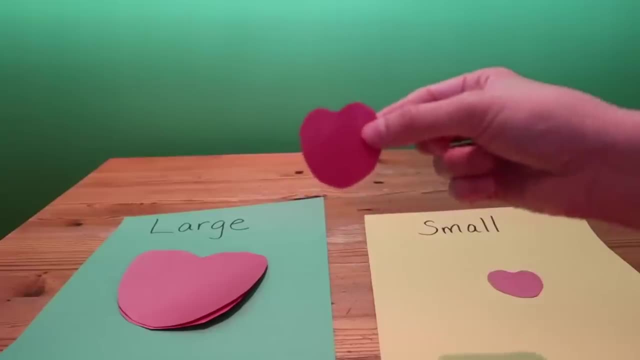 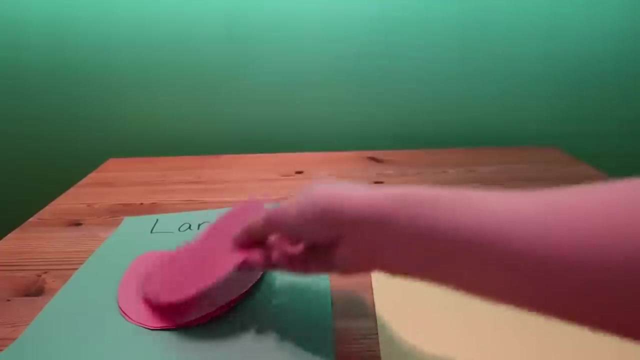 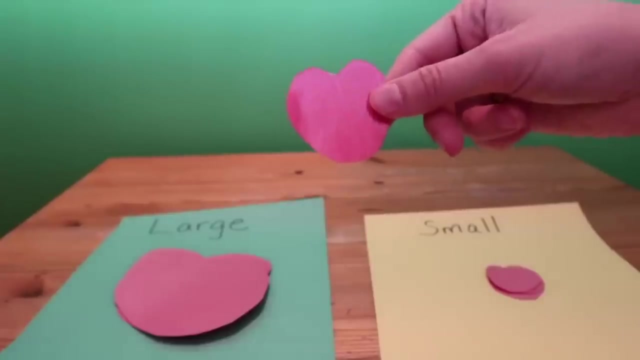 How about this one? Large or small, Small, Good job, Large or small. Large, Good, Large or small, Small. Uh-oh, I'm not sure where this goes. Large or small, Small, Good job, Large or small. 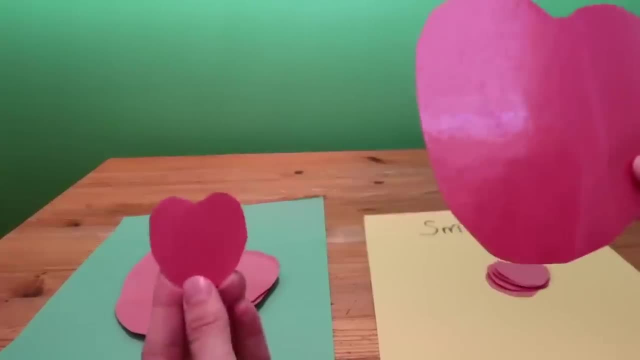 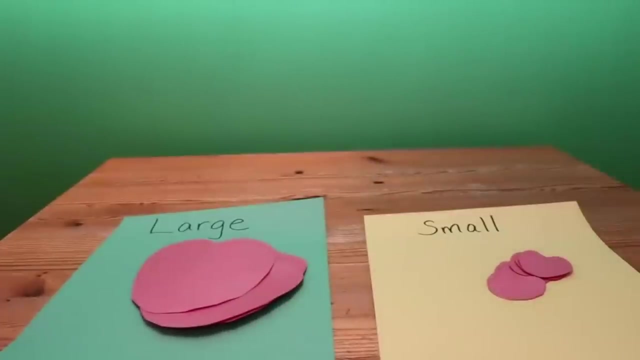 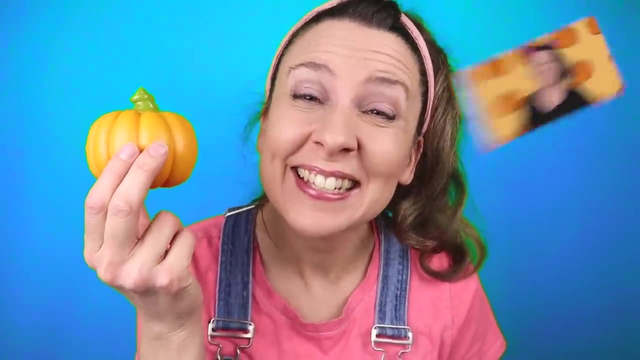 Large, Great work. What about the last two? Yeah, This is large and this is small. Yay, We did it. I'm so proud of you. Let's do five little pumpkins. Get out your arm and we'll pretend it's a gate. 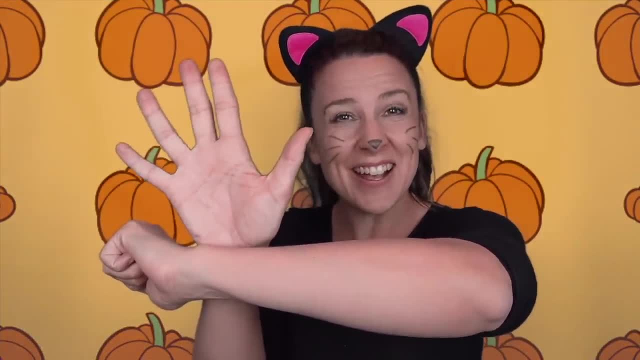 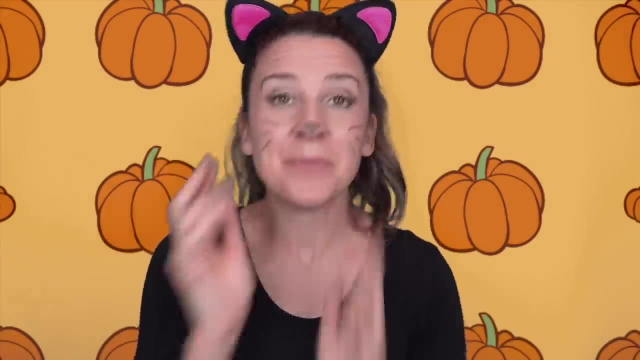 And then get out five little pumpkins. Good job, Five little pumpkins sitting on a gate. The first one said: oh my, it's getting late. The second one said: there are witches in the air. The third one said: but we don't care. 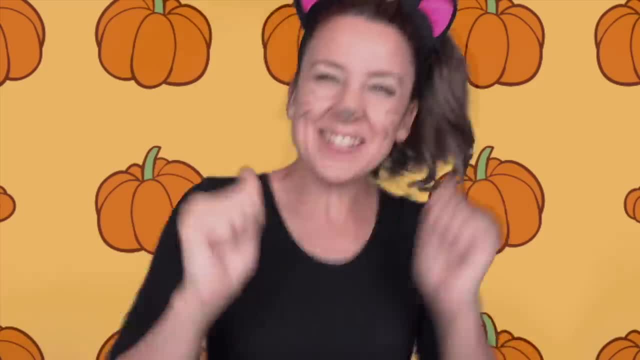 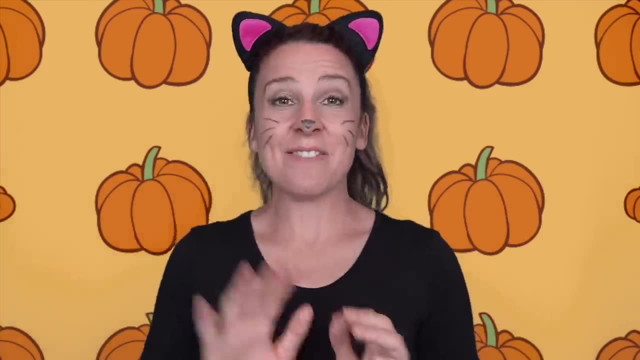 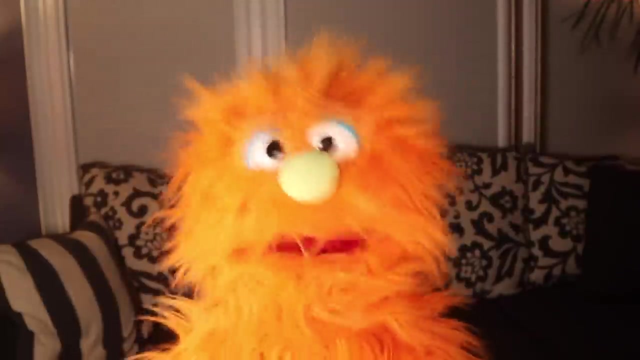 The fourth one said: let's run and run and run. The fifth one said: I'm ready for some fun. Ooh went the wind and out went the light, And the five little pumpkins rolled out of sight. Good job. What do you call a bunch of strawberries in a band together? 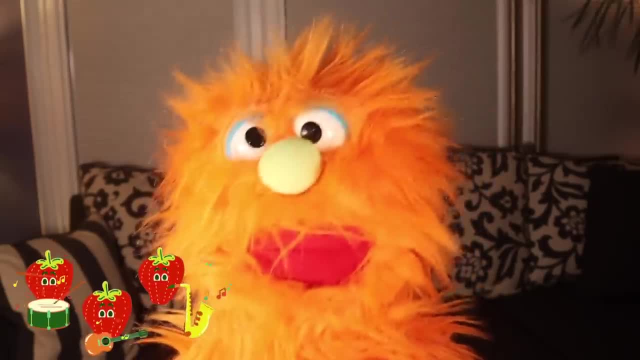 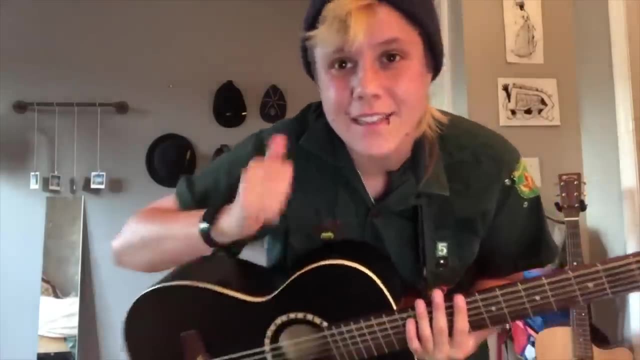 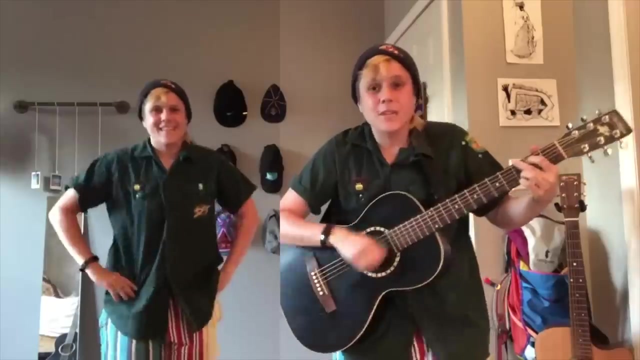 A jam session. This song's called the Hokey Pokey. I bet you already know it. Are you all ready? Okay, let's go. You can follow along with me right here. You put your left foot in. you put your left foot out. 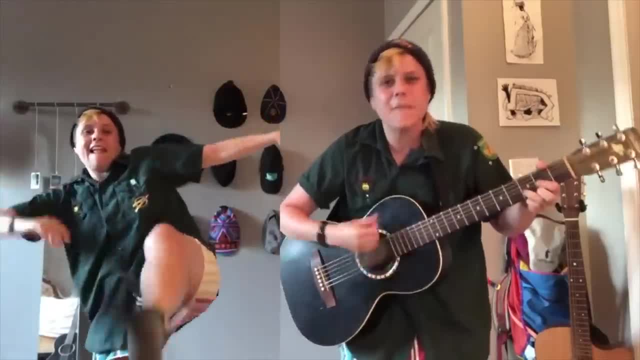 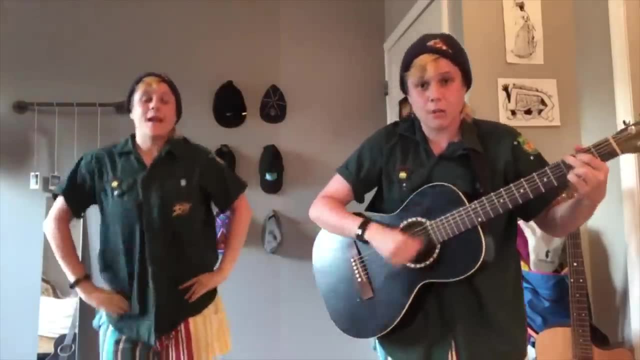 You put your left foot in and you shake it all about. You do the hokey pokey and you turn yourself around. That's what it's all about. You put your right foot in, you put your right foot out, You put your right foot in and you shake it all about. 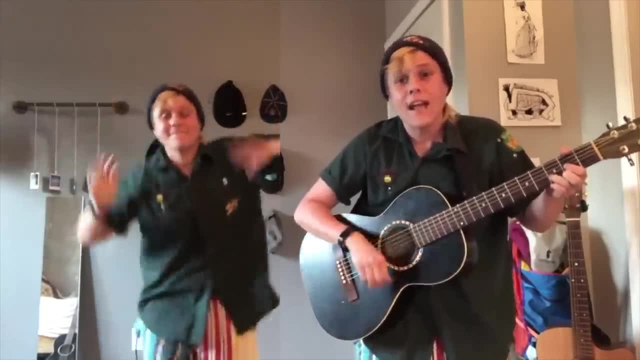 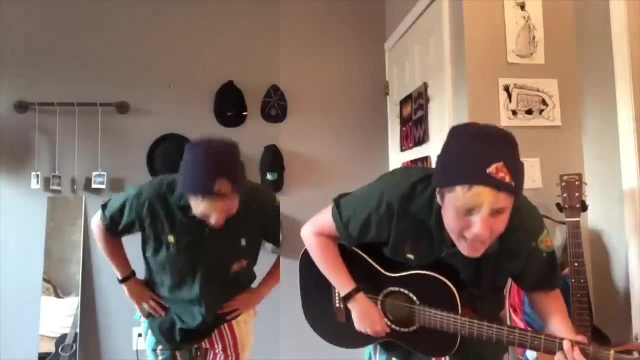 You do the hokey pokey and you turn yourself around. That's what it's all about. You put your head in, you put your head in, You put your head out, you put your head in And you shake it all about. 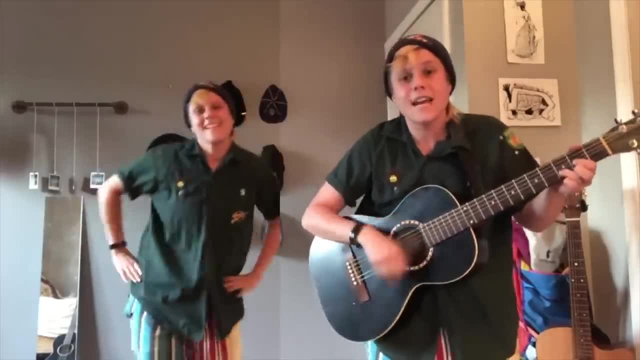 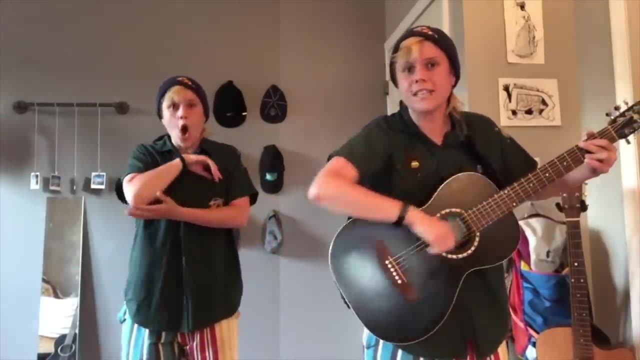 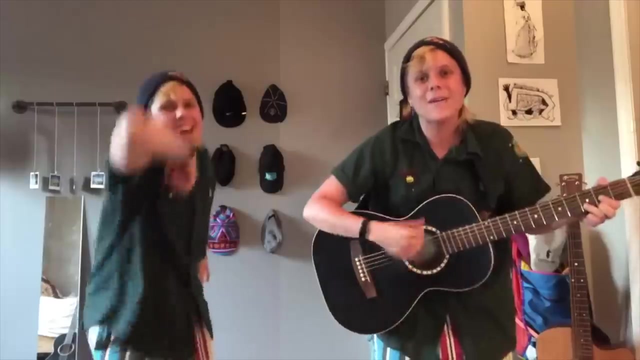 You do the hokey pokey and you turn yourself around. That's what it's all about. What else should we put in this circle? How about our elbows? You put your right elbow in, you put your right elbow out, You put your right elbow in and you shake it all about. 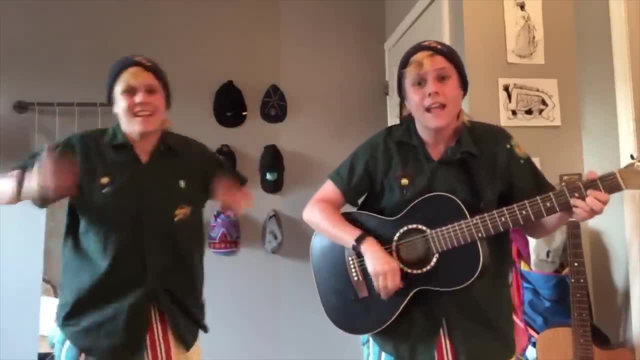 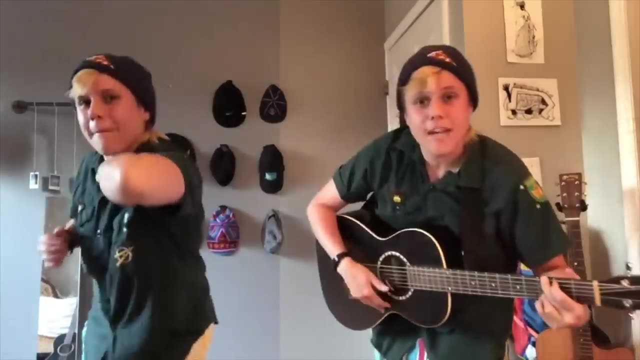 You do the hokey pokey and you turn yourself around. That's what it's all about. Let's do the left elbow ready. You put your left elbow in, you put your left elbow out, You put your left elbow in and you shake it all about. 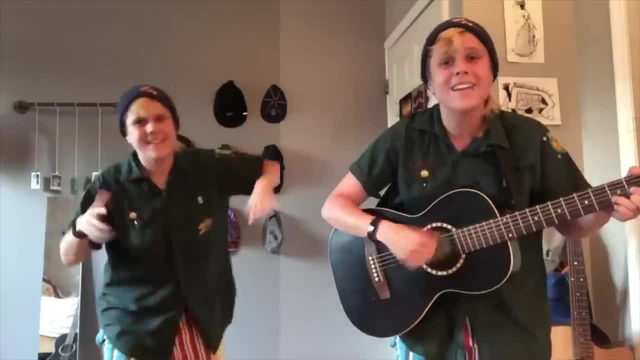 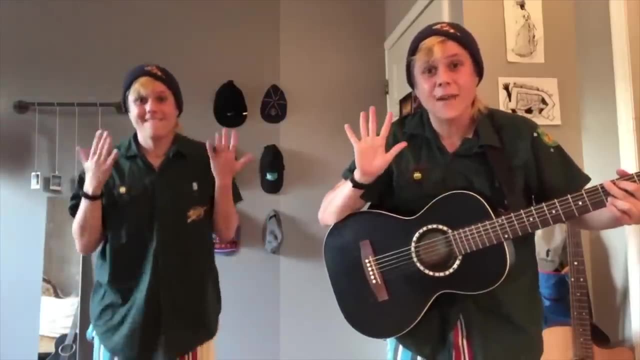 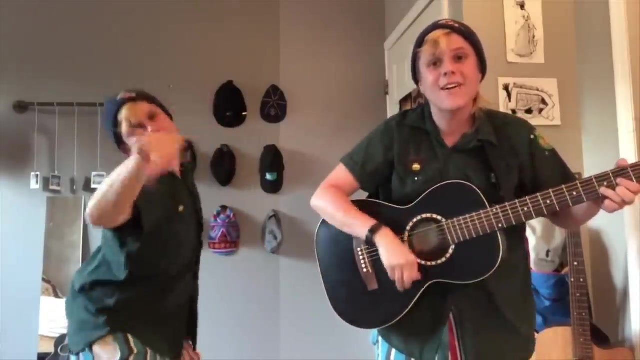 You do the hokey pokey and you turn yourself around. That's what it's all about. Alright, let's do our hands Ready. We put our right hand in, we put our right hand out, We put our right hand in and we shake it all about. 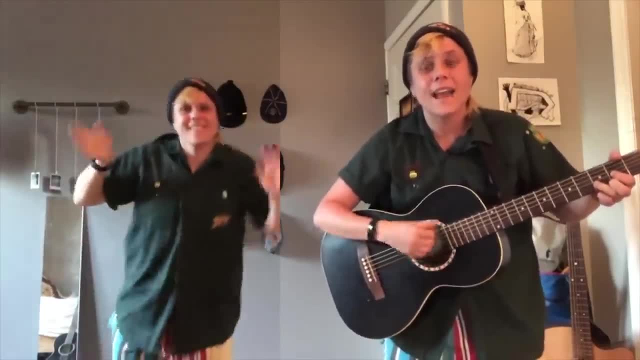 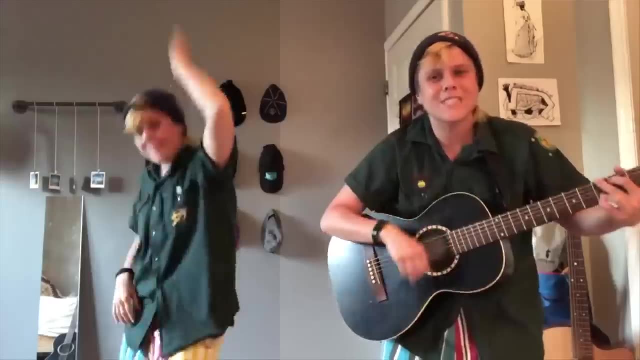 You do the hokey pokey and you turn yourself around. That's what it's all about. You put your left hand in, you put your left hand out, You put your left hand in and you shake it all about. You do the hokey pokey and you turn yourself around. 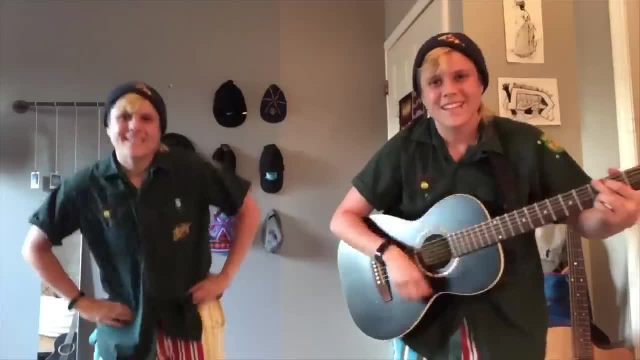 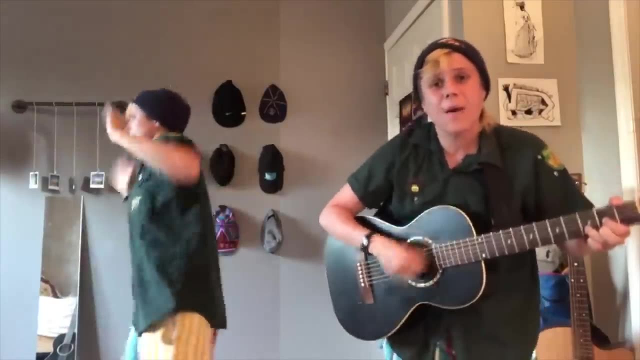 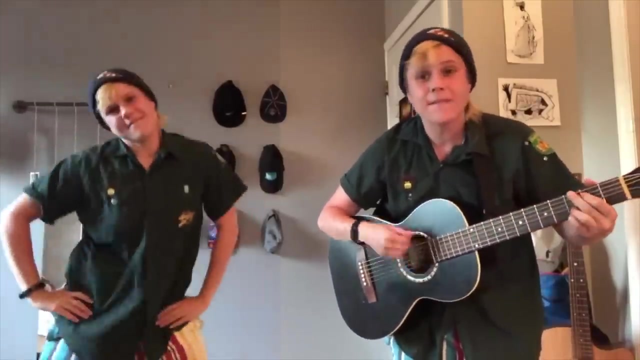 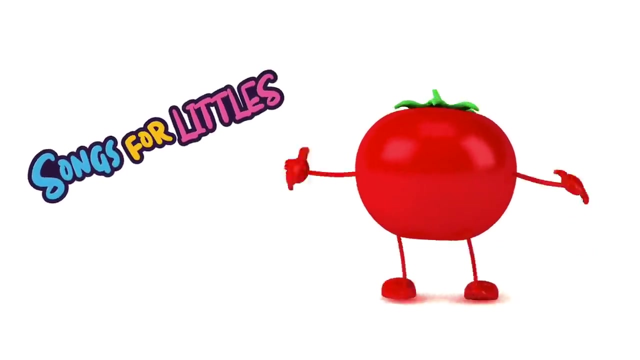 That's what it's all about. Free dance: You do the hokey pokey, You do the hokey pokey, You do the hokey pokey. That's what it's all about. Yay, Let's pretend to cut some fruit together. 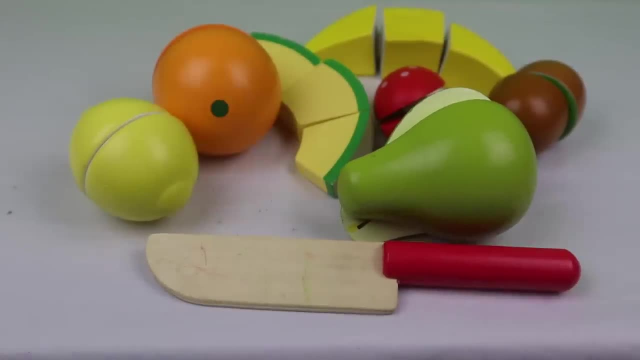 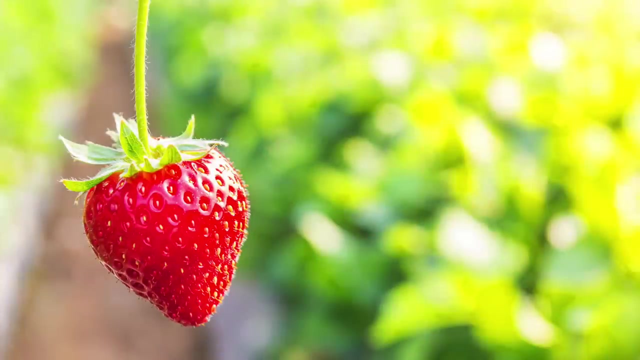 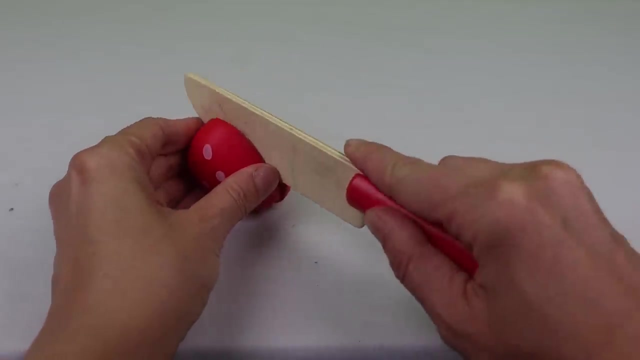 This is a pretend knife. Remember, real knives are only for grown-ups. Do you remember what this fruit is called? Yeah, it's a strawberry, A red strawberry. You say: cut and we'll cut the strawberry. Cut, We did it. 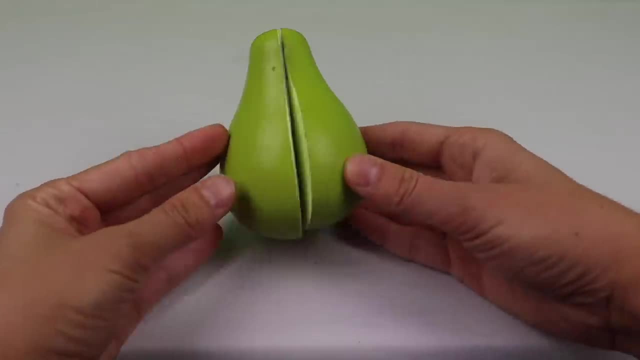 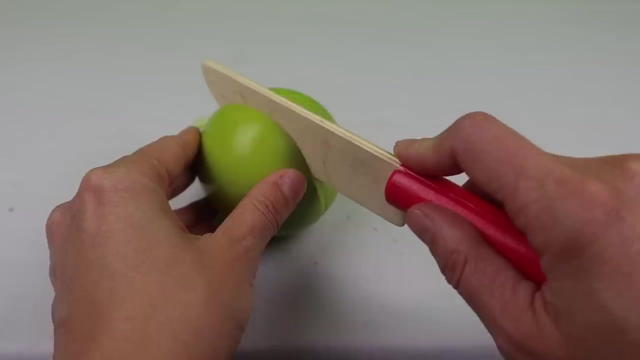 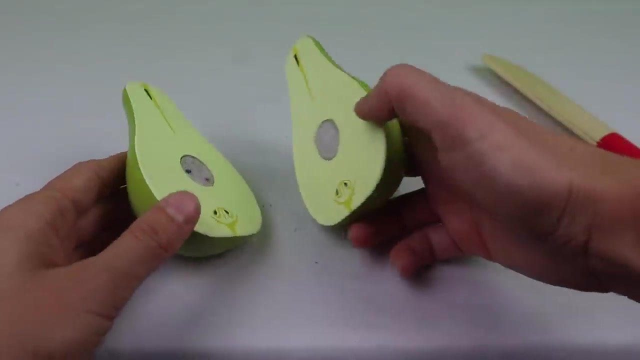 We cut the strawberry into two halves. Do you know what this fruit is called? Yeah, it's a pear, A green pear. You say, cut and we'll cut it. Ready set, cut. We did it. We cut the whole pear into two halves. 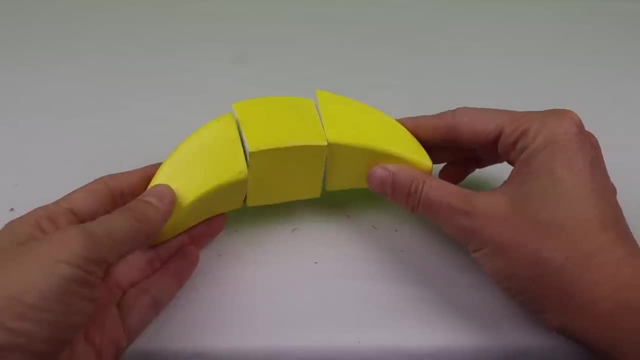 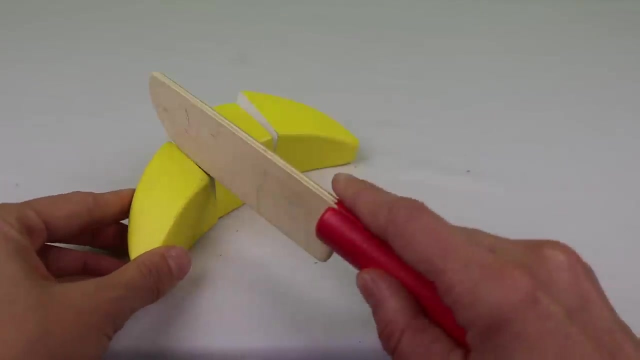 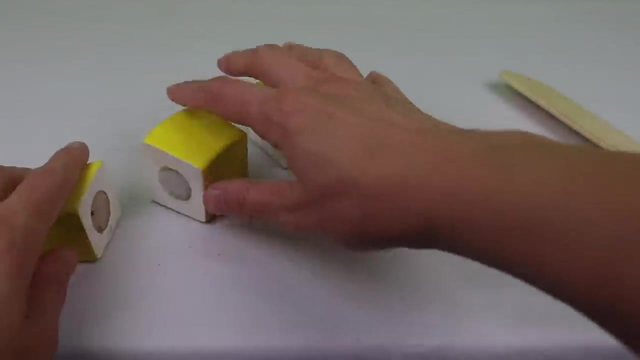 Do you remember what this is called? Yeah, it's a banana, A yellow banana. You say, cut and we'll cut it. Ready, set, cut, Cut. Oh wow. Let's see how many pieces we cut it into: One, two, three. 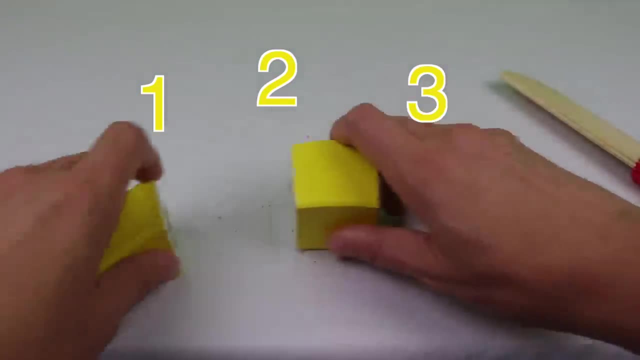 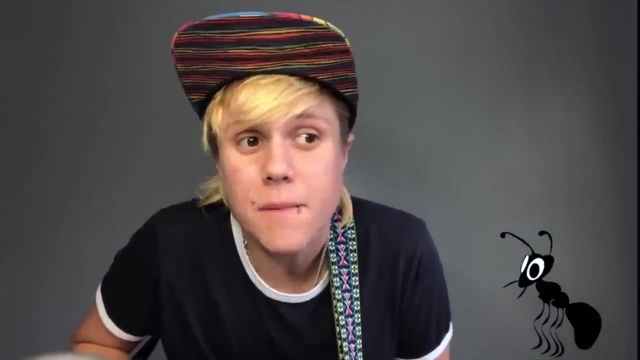 Three pieces of banana. Great job. The next song we're going to sing is about a tiny little bug called an ant. We're going to sing a song about them marching And we're going to count them as they march. Can you march with me? 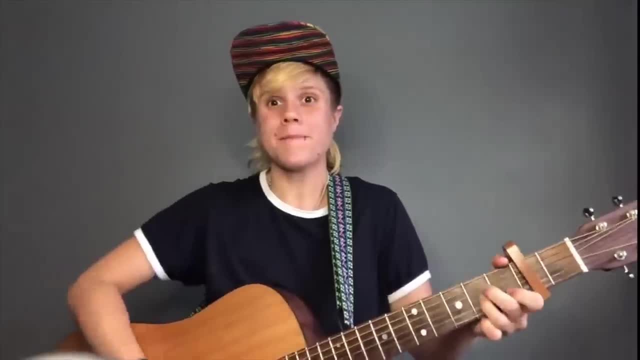 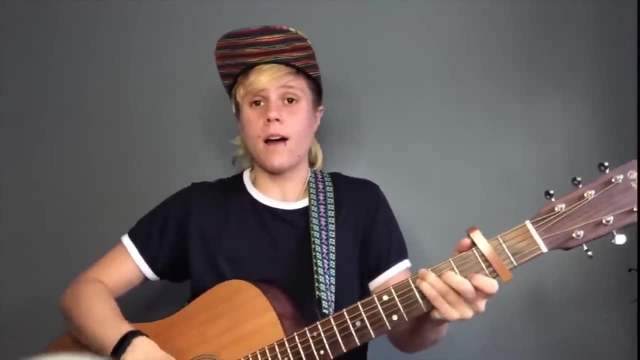 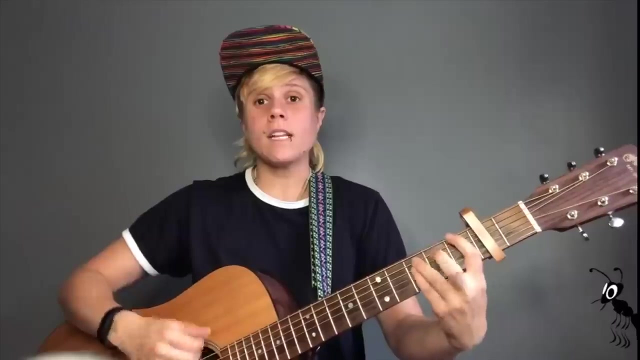 Let's go. Here we go. The ants go marching one by one. Hurrah, Hurrah. The ants go marching one by one. Hurrah, Hurrah. The ants go marching one by one. The little one stopped to suck his thumb. 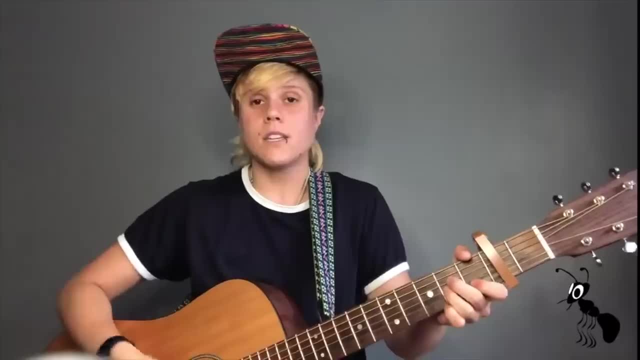 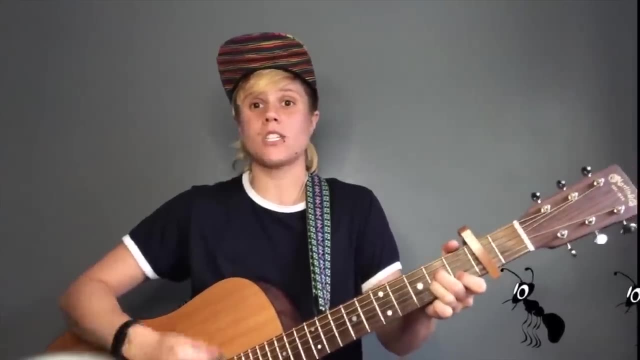 and they all go marching down to the ground to get out of the rain. Boom, boom, boom, boom, boom, boom, boom. The ants go marching two by two. Hurrah, Hurrah. The ants go marching two by two. 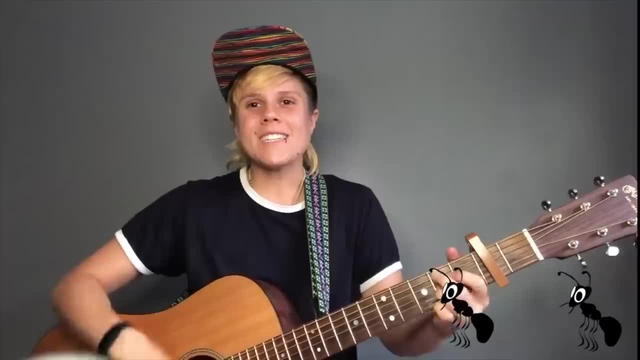 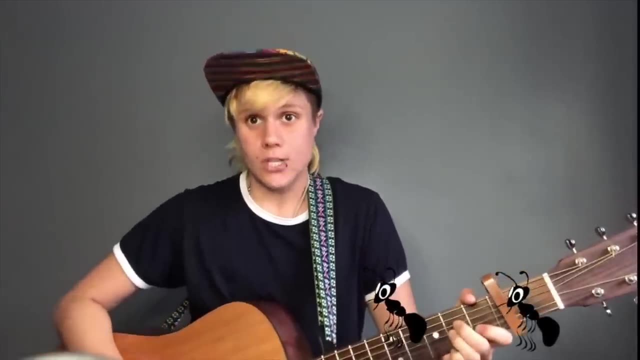 Hurrah, Hurrah, The ants go marching two by two. The little one stopped to tie his shoe and they all go marching down to the ground to get out of the rain. Boom, boom, boom, boom, boom, boom boom. The ants go marching three by three. Hurrah, Hurrah. The ants go marching three by three. Hurrah, Hurrah. The ants go marching three by three, Hurrah, Hurrah. The ants go marching three by three. The little one stopped to climb a tree. 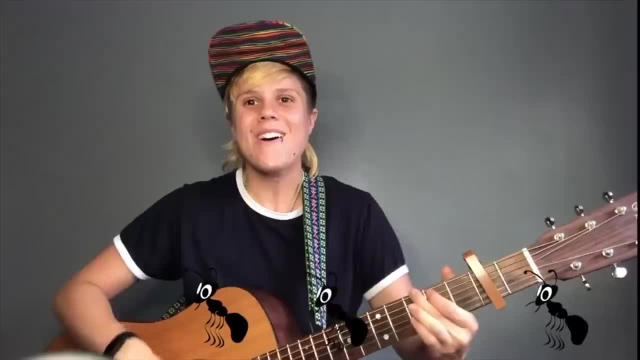 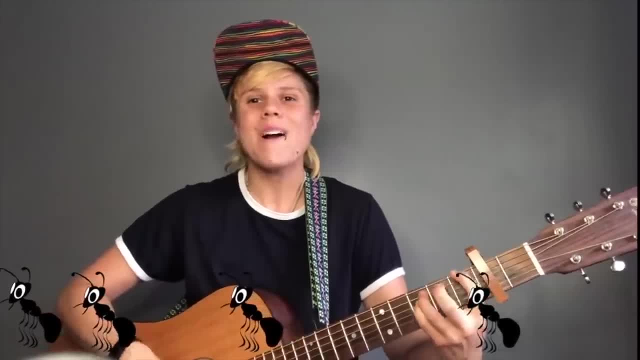 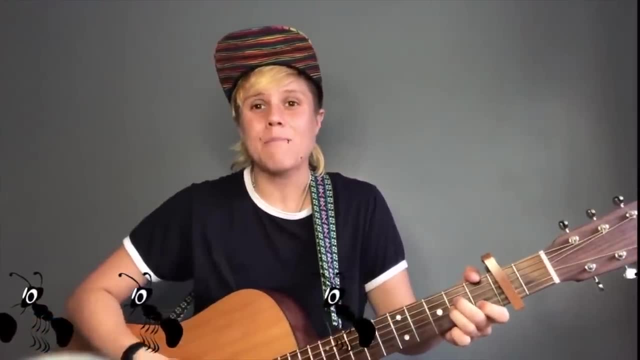 The little ones stop to shut the door and they all go marching down to the ground to get out of the rain. Boom, boom, boom, boom, boom, boom, boom. The ants go marching five by five. Hurrah, hurrah, the ants go marching five by five. 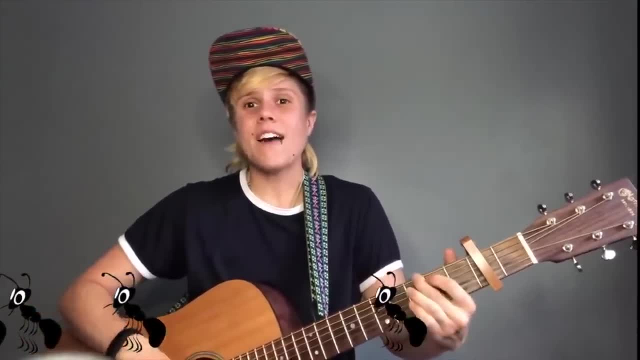 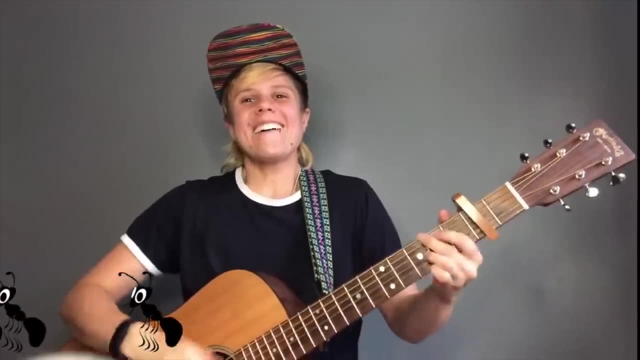 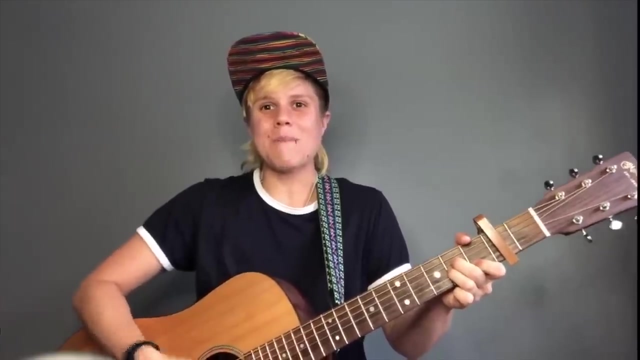 Hurrah, hurrah. the ants go marching five by five. the little ones stop to give a high five And they all go marching down to the ground to get out of the rain. Boom, boom, boom, boom, boom, boom boom. 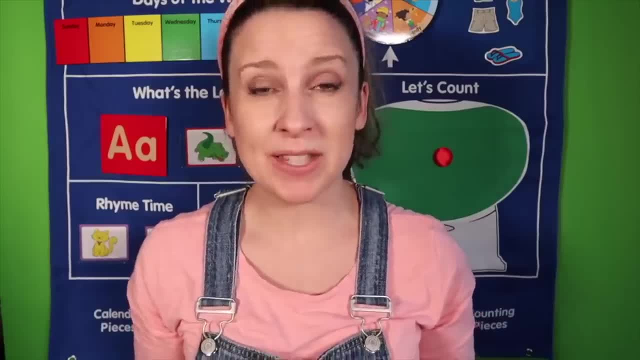 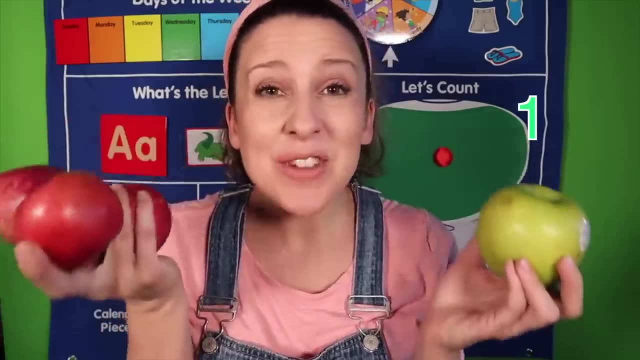 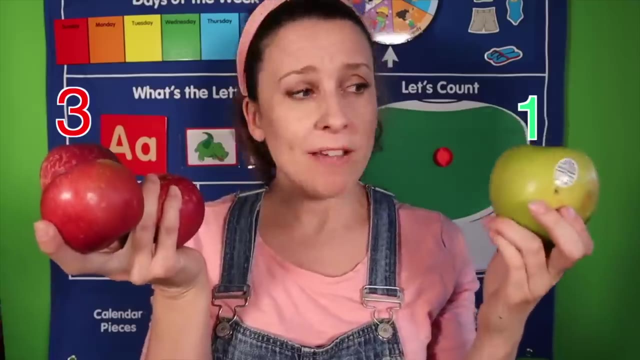 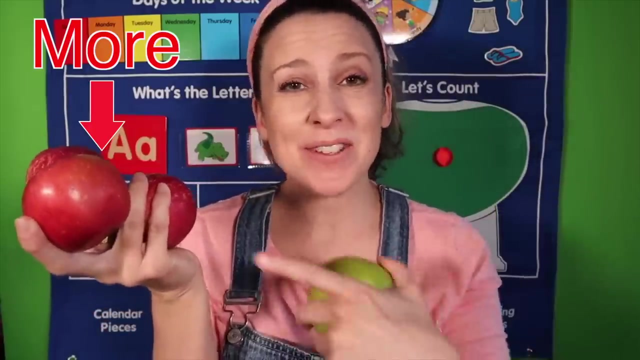 Now I'm going to put the apples in my refrigerator into two groups: Green apples- I have one green apple- And red apples. I have three red apples: One, two, three- Good counting. Do I have more green apples or more red apples? There's more red apples, More red apples. 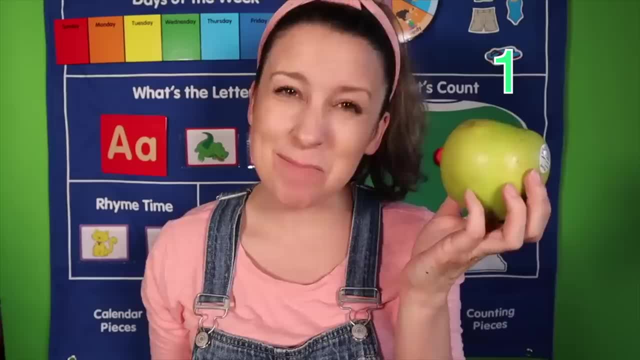 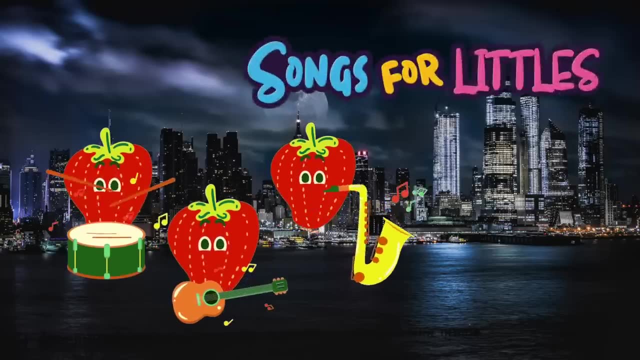 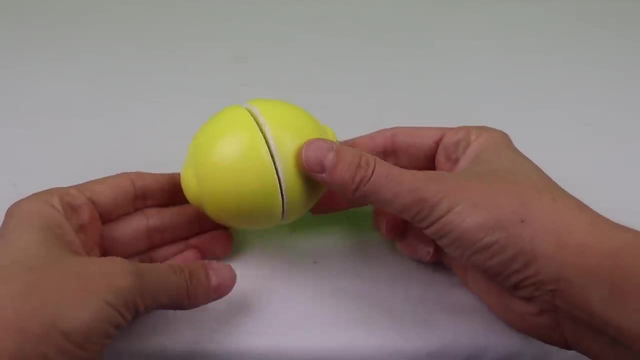 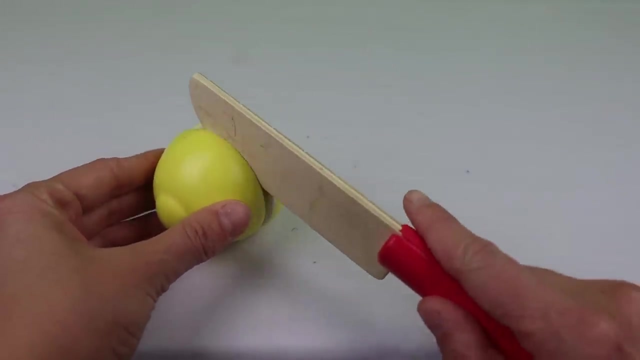 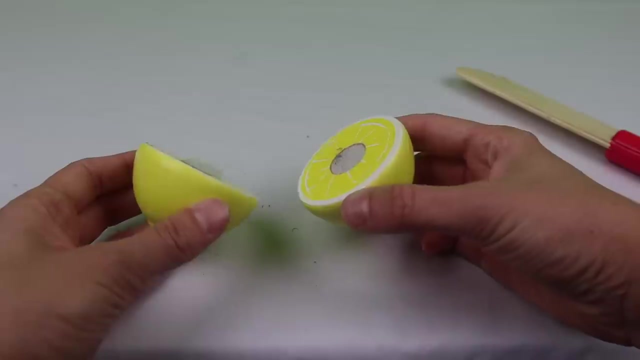 Less green apples, Only one green apple, Three red apples. Wow, Good job. Do you know what this fruit is called? It's very sour. Yeah, it's a lemon, Let's cut it. You say: cut Ready, set, cut, Push down. We did it. We cut the whole lemon into two halves. 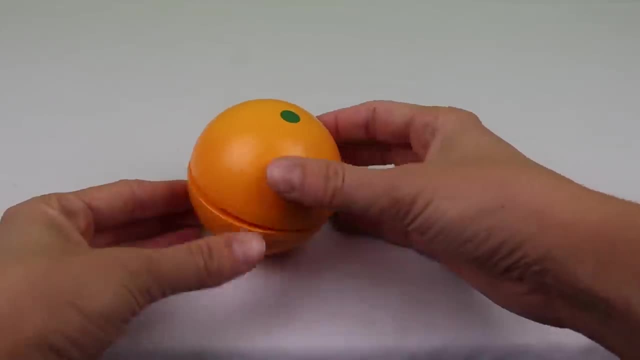 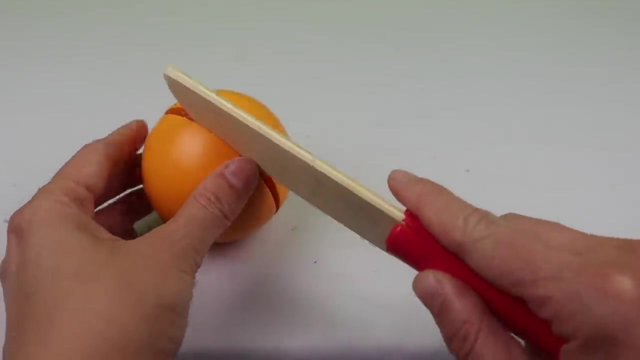 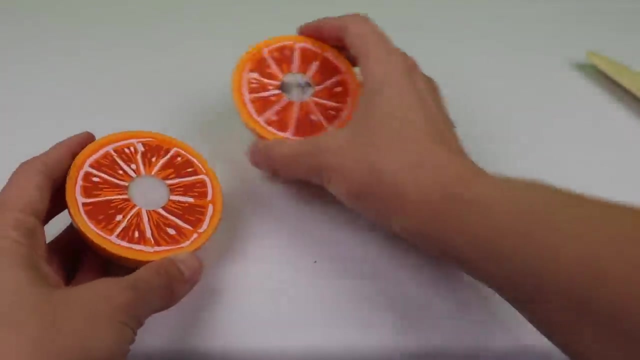 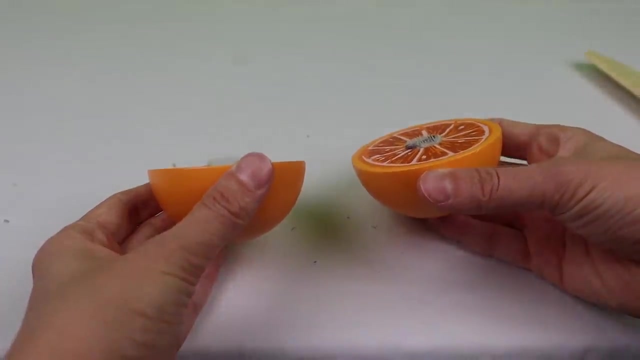 Do you know what this fruit is called? Yeah, it's an orange, An orange orange. That's so silly. You say, cut and we'll cut it. Cut, We pretended to cut it. Yay, Look inside. Wow, We cut the whole orange into two halves. Good job Have. 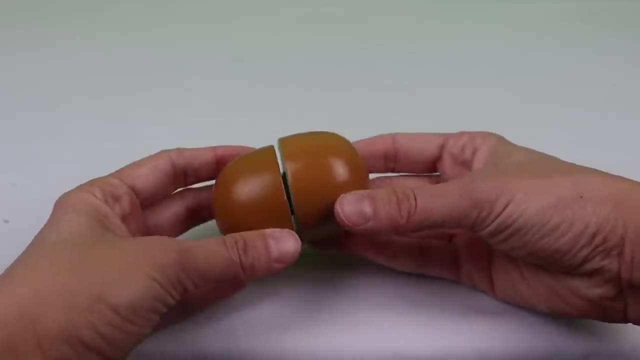 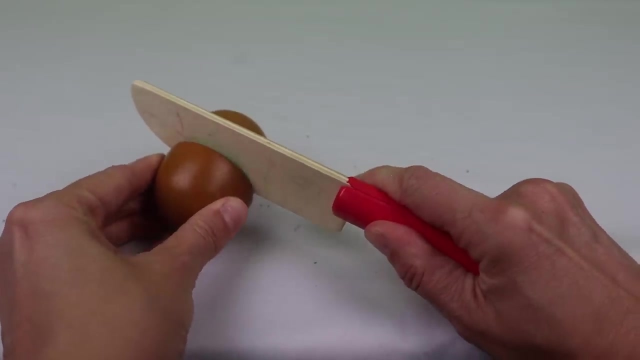 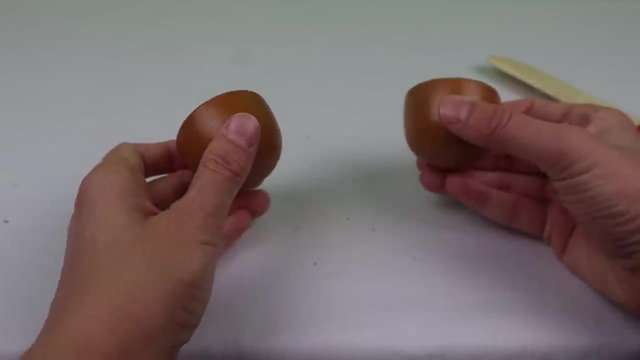 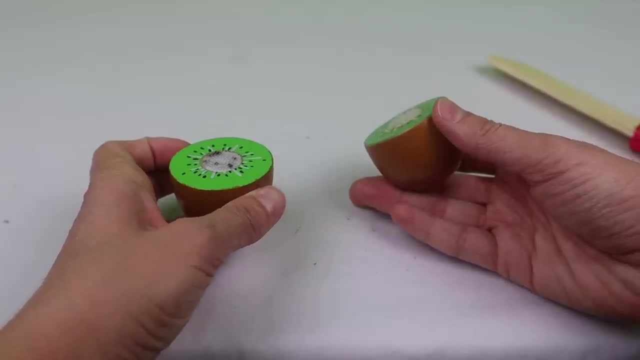 you ever seen this fruit? It's really fuzzy. It's called a kiwi. Let's cut it open and see what's inside. Ready, set, cut, Cut, You did it. Oh, the inside is green. Wow Say kiwi. Kiwi One whole, kiwi two halves. 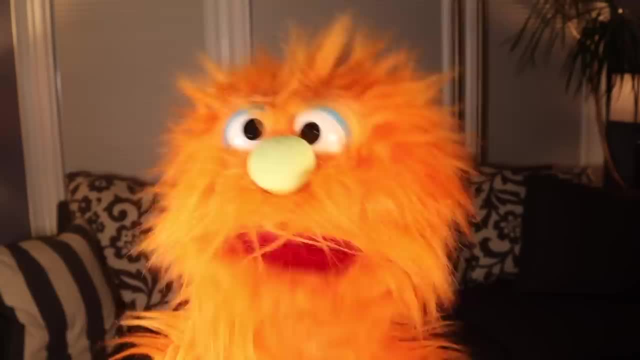 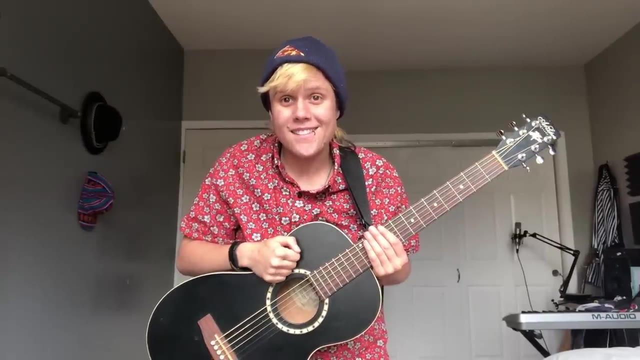 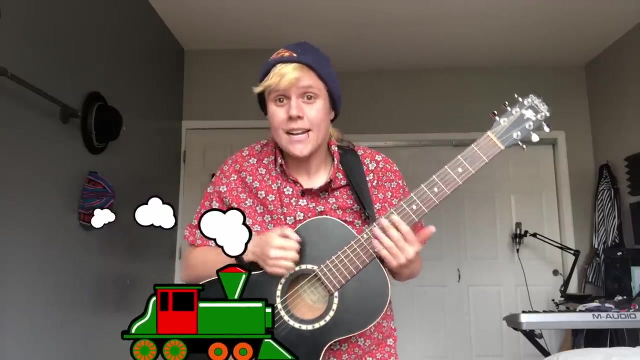 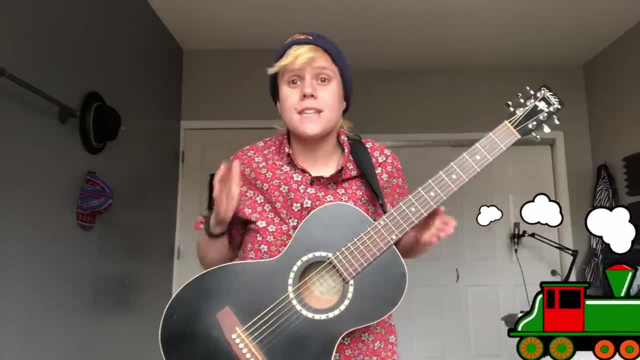 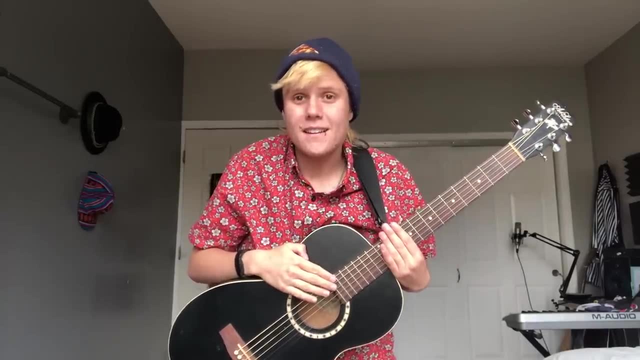 So we're going to pretend to be trains. We're going to walk in a circle with our arms like this, And whenever I say the word stop, we're going to freeze and wait for the train to start back up again. You can just follow along right up here. Are you ready, All aboard? 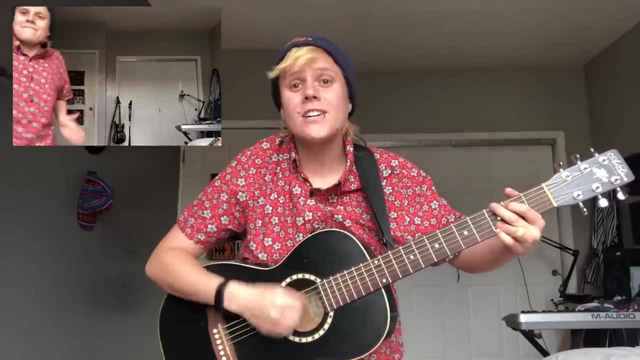 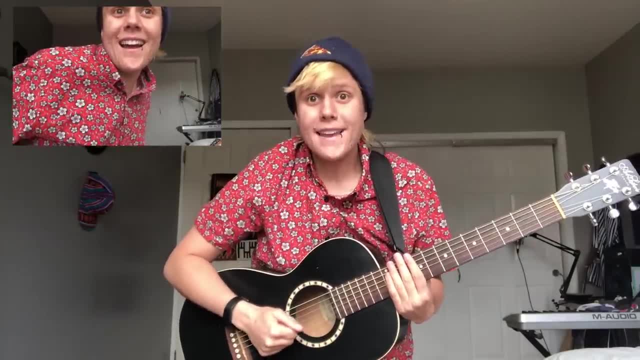 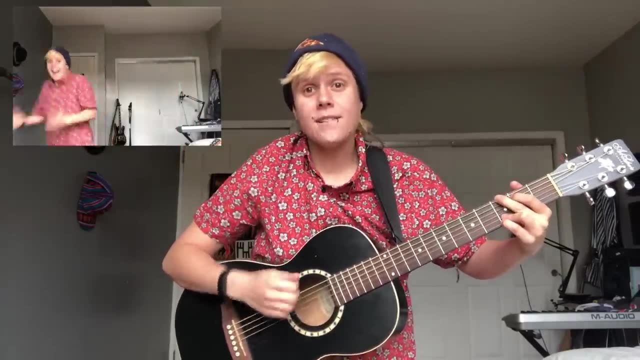 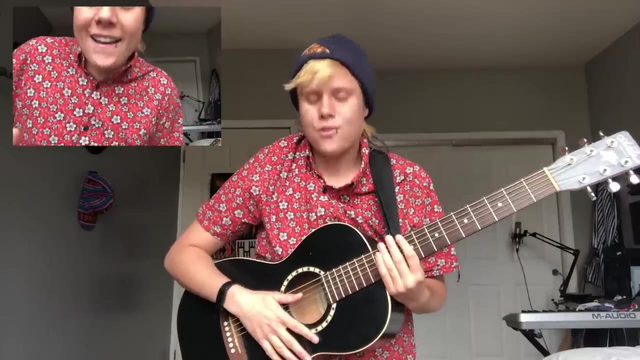 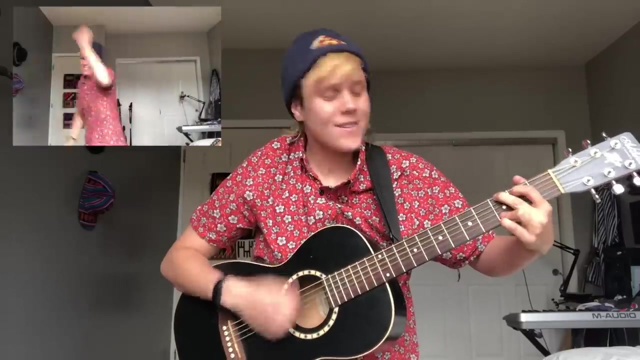 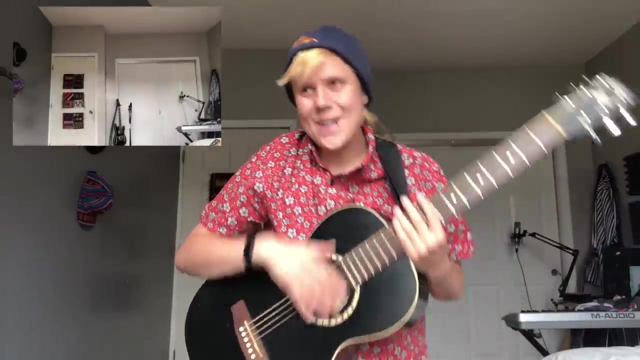 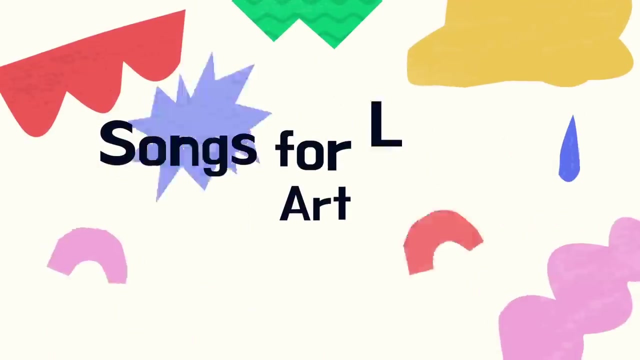 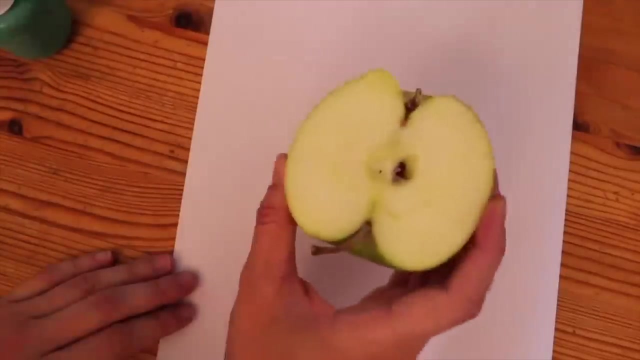 All right, we're going to go really, really fast this time. Are you ready? I think we can go faster. Woo, That was fun. Thanks for pretending to be a train with me. Apple prints. So we take an apple and you have a grown-up help you cut it in half. 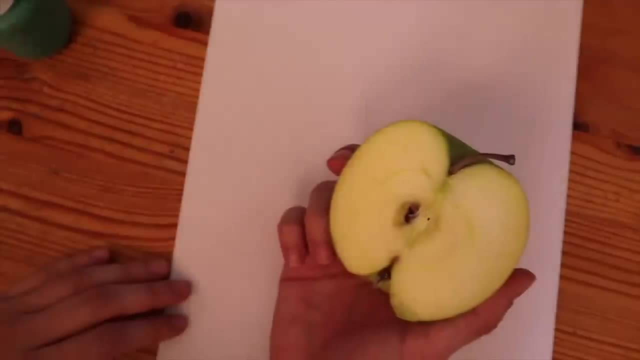 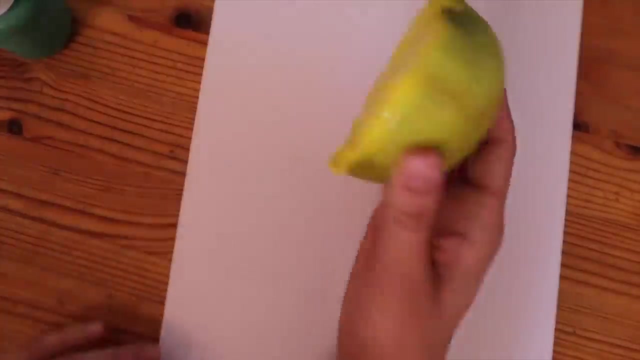 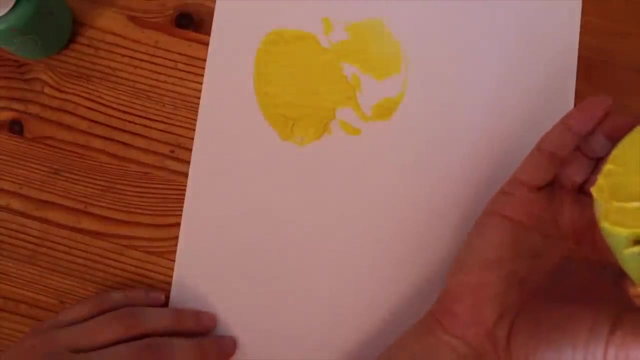 and then we're going to make a print, So we're going to dip it in paint. Did you know? some apples are yellow, So I dip this in yellow paint. Now I'm going to stamp it on. Can you say stamp, Stamp. Let's see how it looks. I'm so excited. Oh, it looks pretty. I like it. Maybe I should hold. 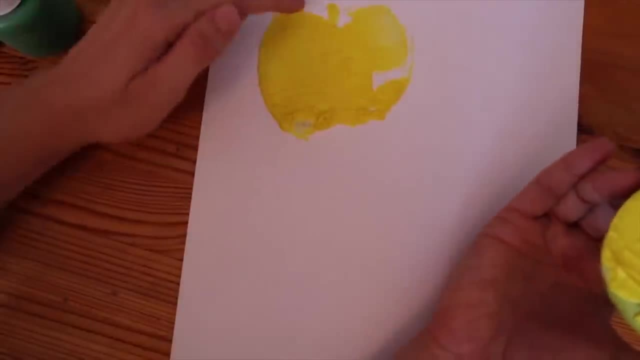 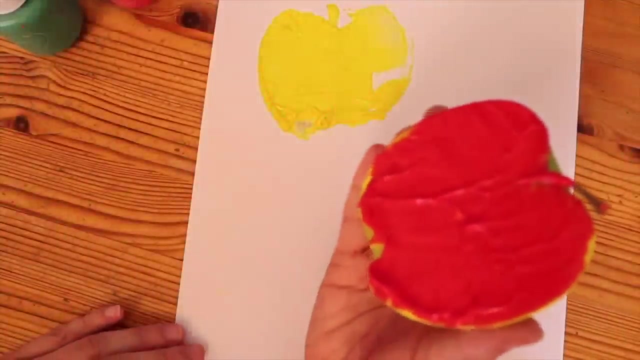 it down a little longer and push. Wow, that looks good. I even see the stem. Next, I'm going to dip it in red paint. Wow, I dipped it in red paint. Now let's stamp it, Say stamp, Stamp, Let's see. 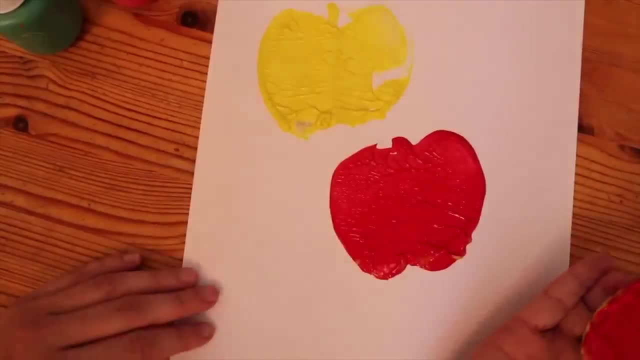 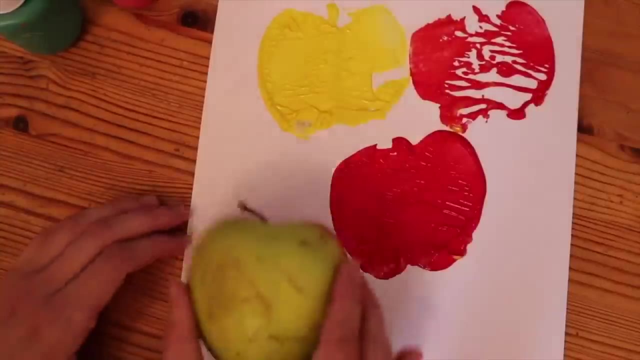 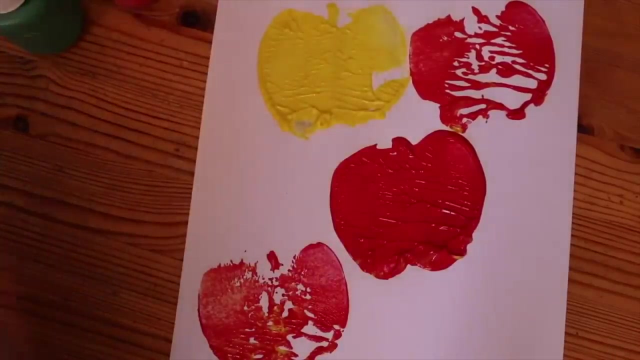 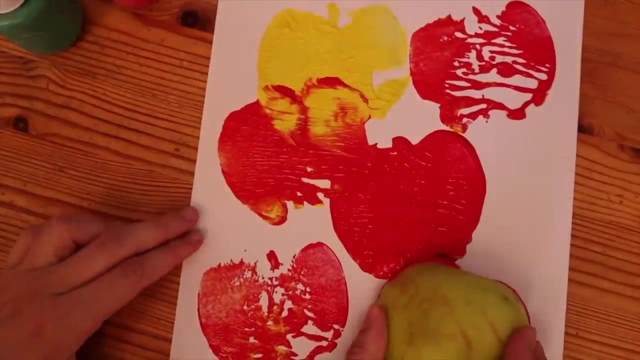 what happens? Push Pretty. Oh, my goodness, I love it. Do another one. Ooh, that one has a lot of spaces, but I like how it looks. Wow, I'm going to mix the yellow and the red together a little bit. Wow, I like printing them on top of each other. It looks nice. 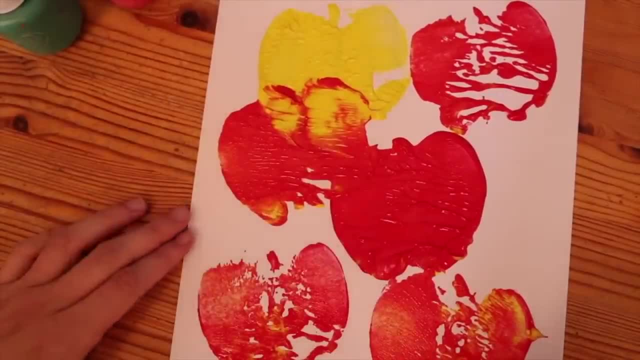 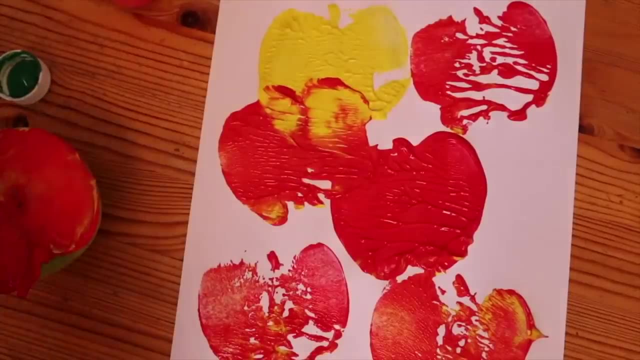 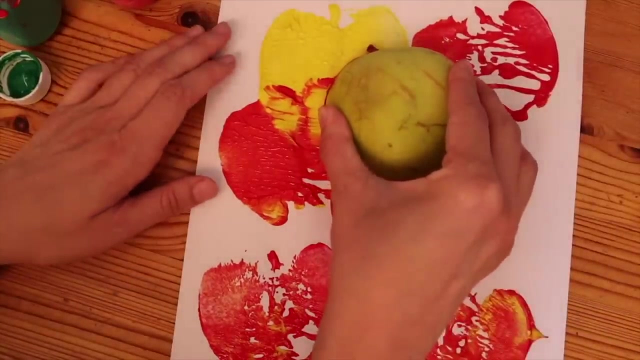 I even see the seed prints a little bit. That's so cool. I really like my picture. You know, we learned also that apples can be green, so I'm going to try green and see how that looks. Let's see how the green looks. I dipped it in green paint. Push Printing with apples. Whoa, Whoa. 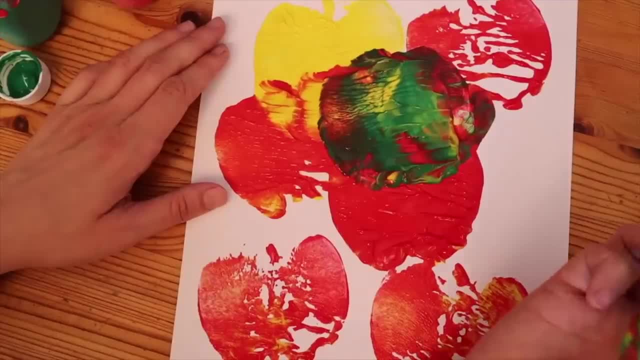 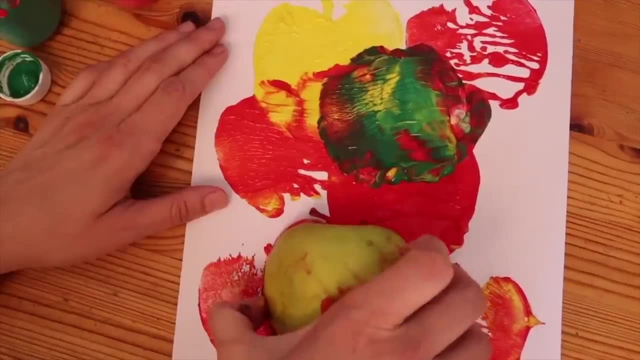 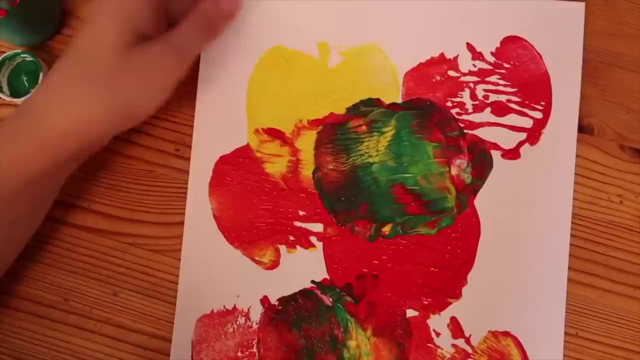 It's pretty messy, That's okay. I can wash my hands after That. one looks like a lot of colors. I like it. Push again. Oh, it's slippery. We did it. We made the apple print picture. I'm proud of myself and I'm proud of you. 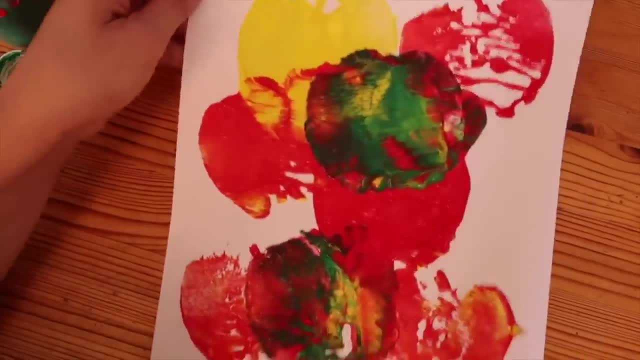 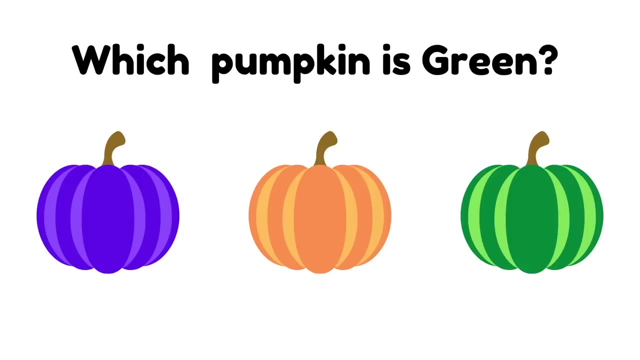 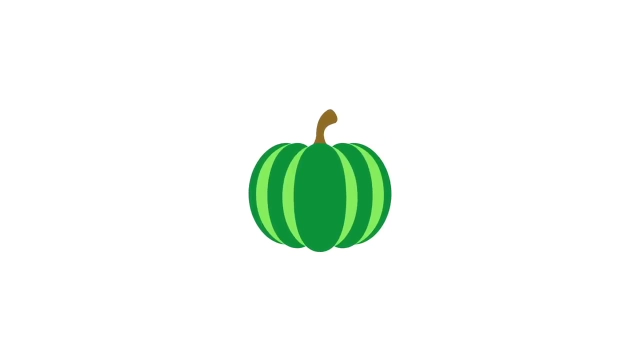 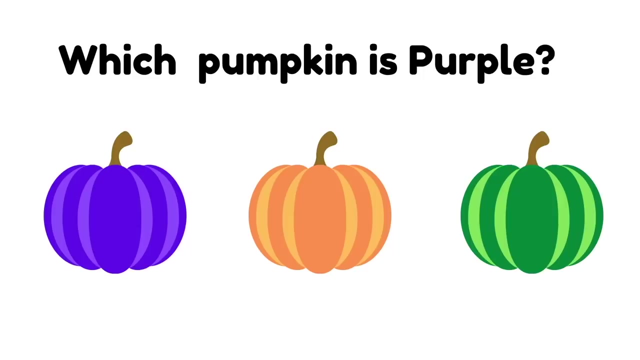 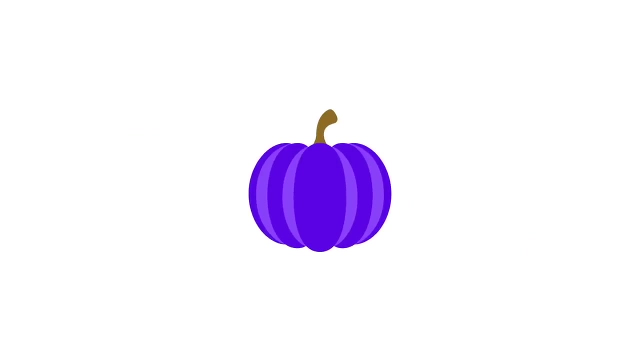 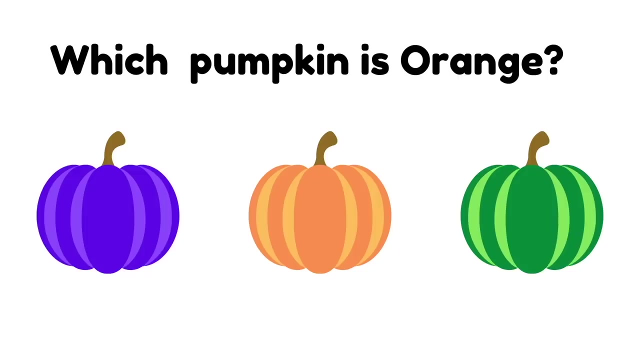 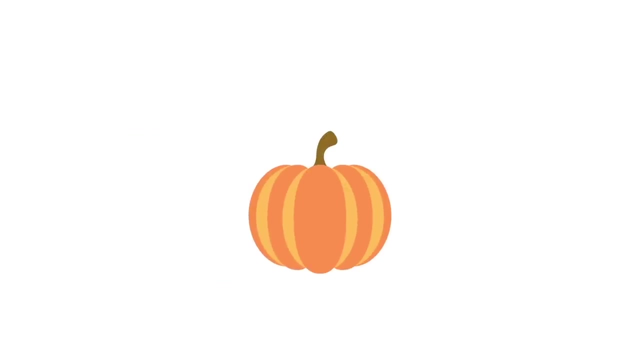 It always feels good to make something, doesn't it? Which pumpkin is green? That's right. This is the green pumpkin. Which pumpkin is purple? Yeah, that's the purple pumpkin. That's right. This is the orange pumpkin. Good job. 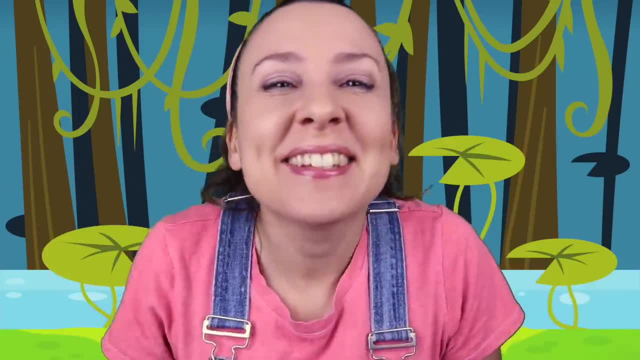 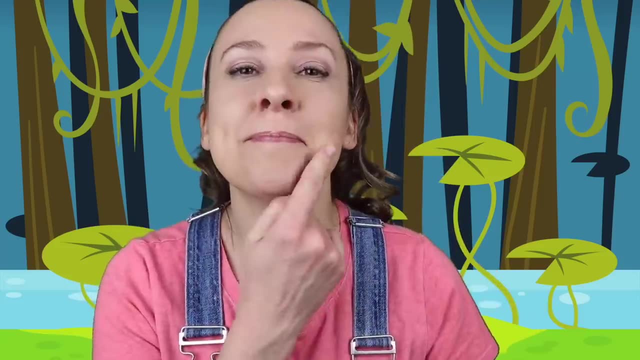 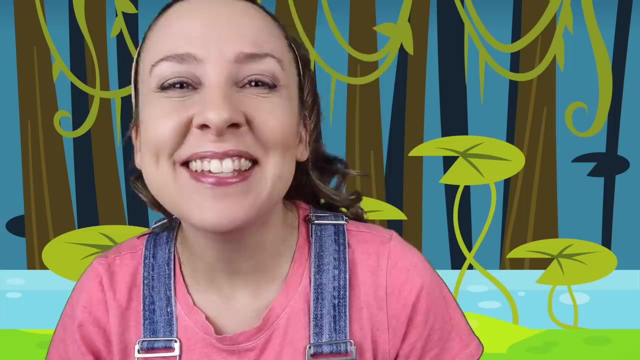 What does a frog say? Ribbit, ribbit, ribbit, ribbit, ribbit. In this song they say something else. It's so silly. Mmm-ah went the little green frog one day. Mmm-ah went the little green frog. 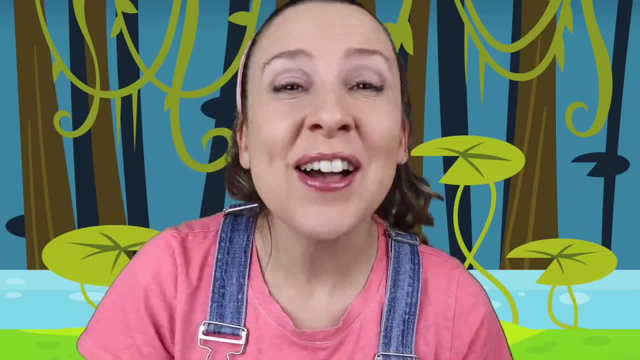 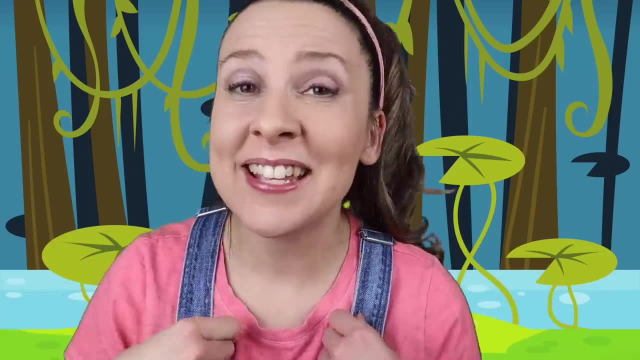 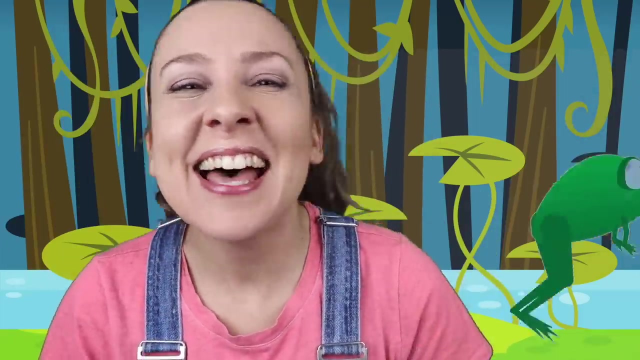 Mmm-ah went the little green frog one day, And they all went mmm-mm-ah. But we know, frogs go La-dee-da-dee-da, La-dee-da-dee-da, La-dee-da-dee-da, We know, frogs go la-dee-da-dee-da. 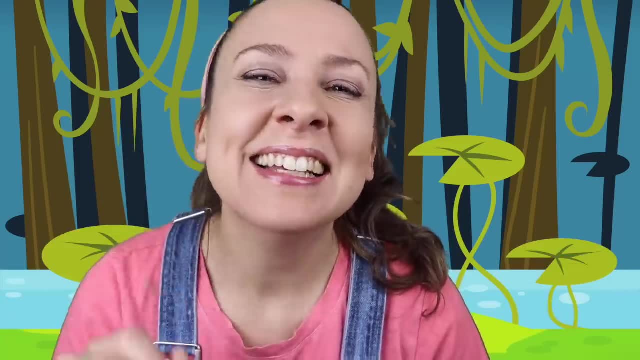 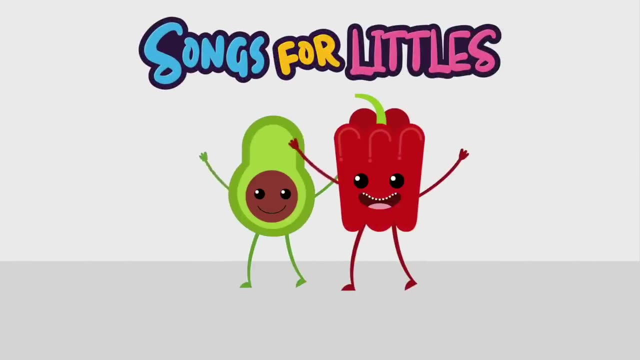 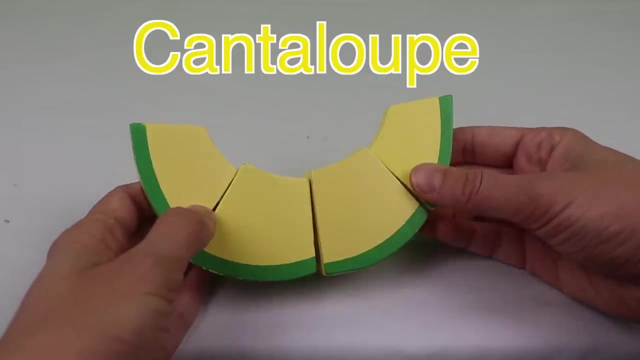 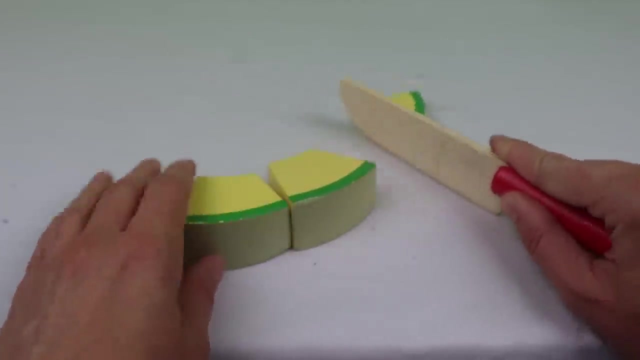 They don't go. mm-mm-ah, That was so silly, Good job. Do you know what this fruit is called? It's called cantaloupe. Let's cut the cantaloupe. Say cut, Cut. You did it. 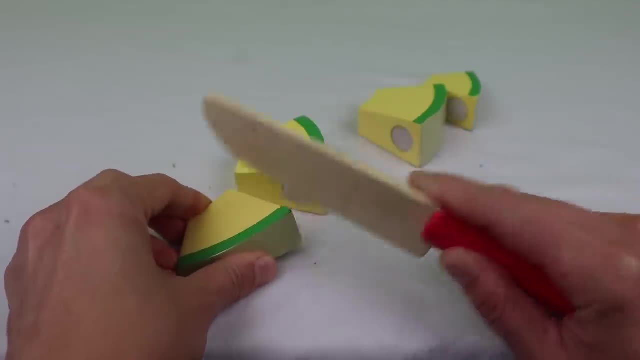 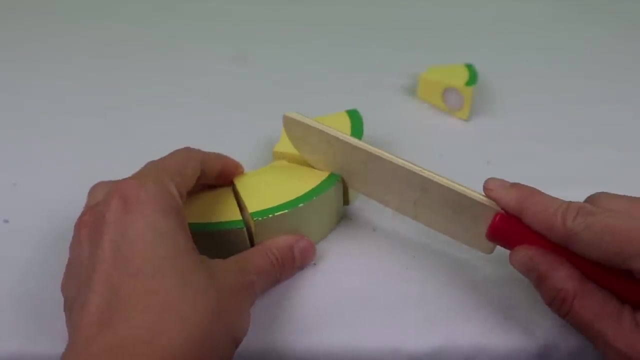 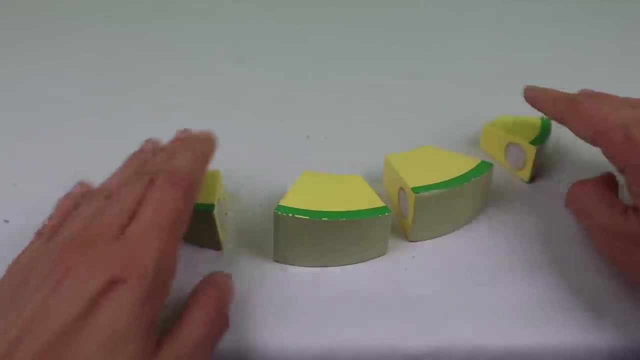 Cut. You did it, Cut. Let's do it again for fun. Cut, Cut, Cut. Let's see how many pieces of cantaloupe we have. We touch each piece and say a number when we touch the piece One. 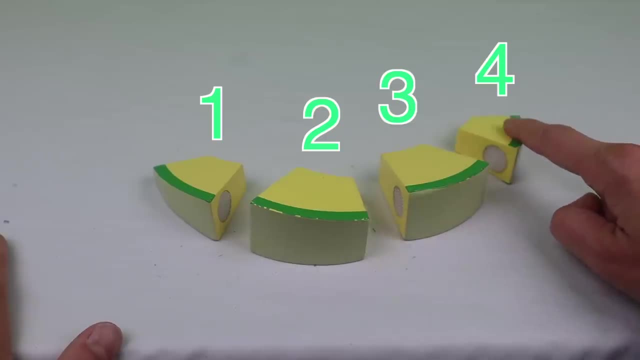 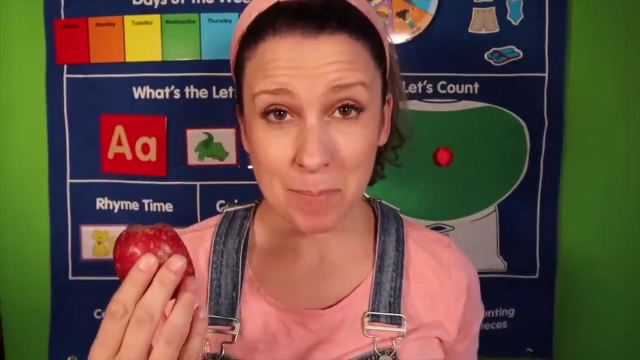 Two, Three, Four, Four pieces of cantaloupe. Four is the last number we said, so we know we have four pieces. We cut all the fruit. Great job, You did it. Next, let's talk about the parts of an apple. 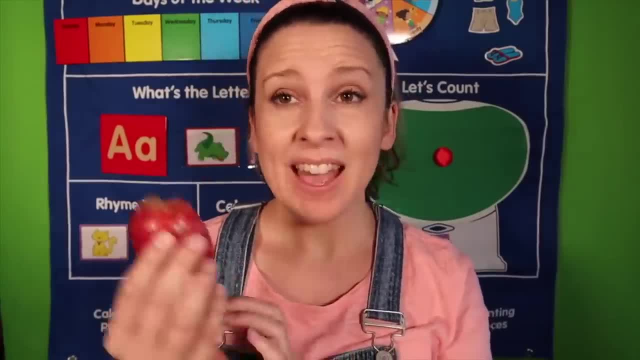 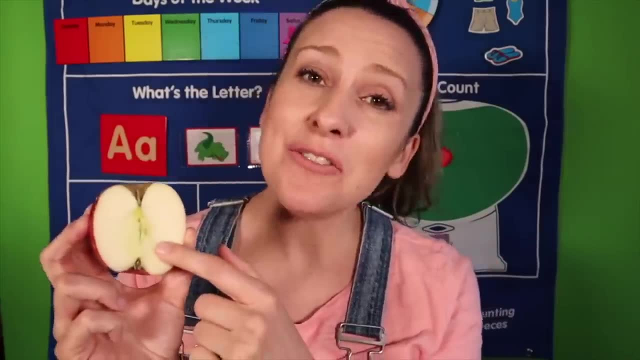 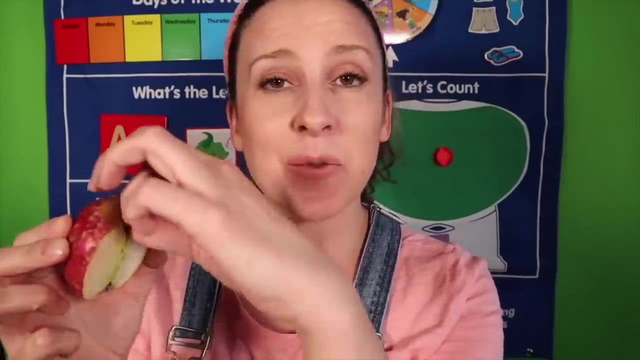 If you have a grown-up to help you, you can cut open an apple. I cut open this apple. This part's the skin of the apple. This part is called the flesh of the apple. This little part is called the stem. The stem is where the apple was hanging from the tree. 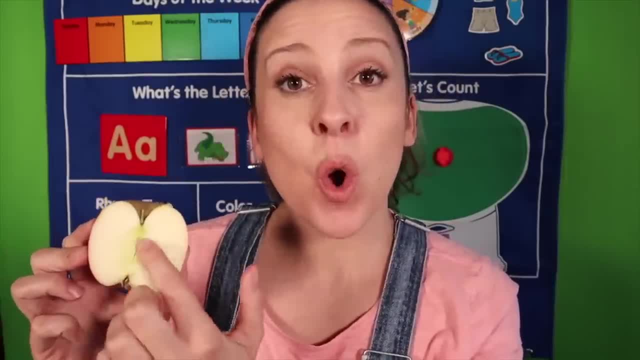 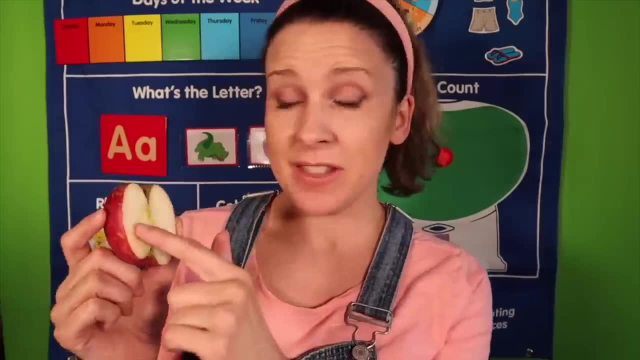 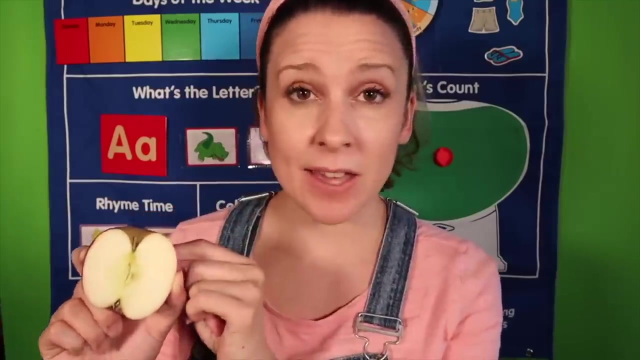 Wow, This part is called the core of the apple. Good listening. yeah, So we have the skin, the flesh, the white part, the core, the stem. Sometimes there's a leaf hanging off. This apple does not have a leaf hanging off. 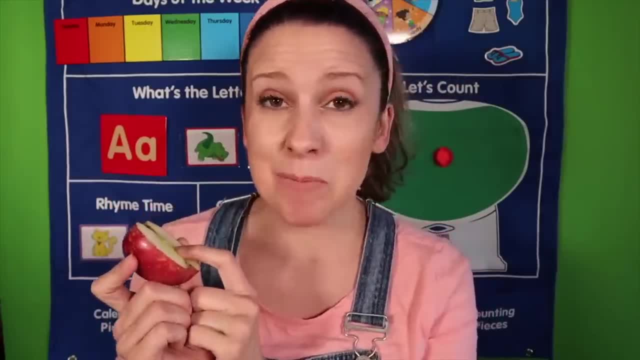 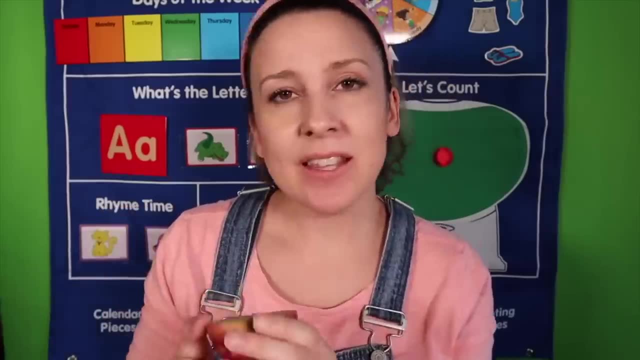 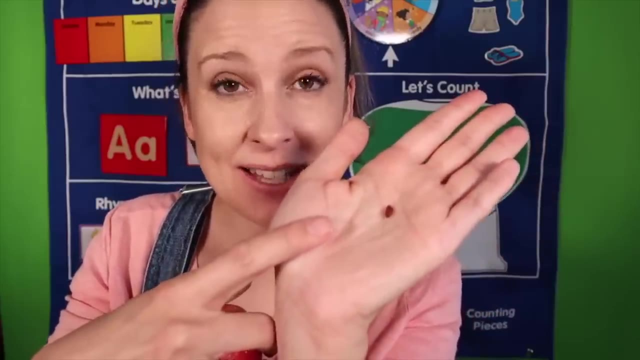 And then I almost forgot: inside the apple- this is really special- there's apple seeds. Wow, yeah, let's see if we can get one out. Wow, here's one of the apple seeds that was inside the apple. It's a brown tiny seed. 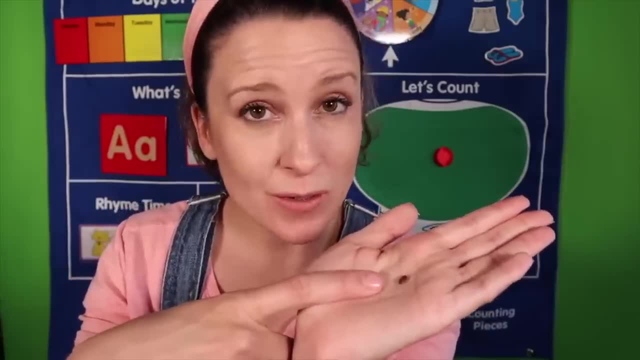 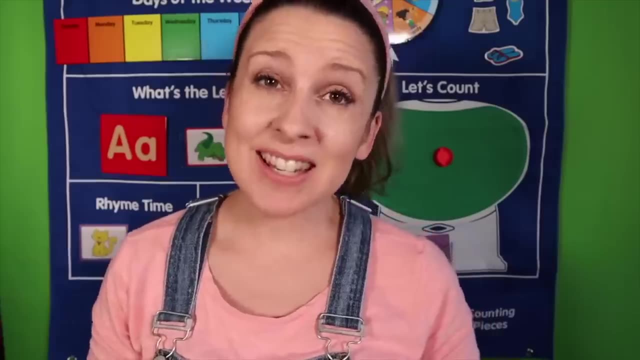 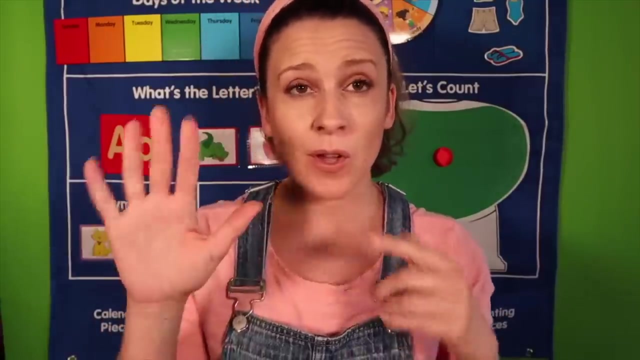 Do you know what would happen if we planted this seed in the ground and gave it sunlight and water and soil? When I was a little girl, we planted an apple tree in my front yard. It was so fun. Guess how many seeds were in my apple. 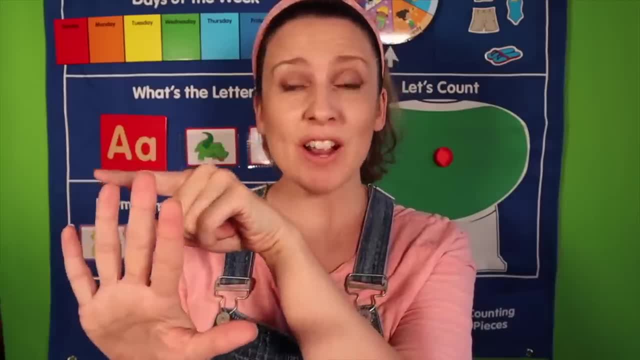 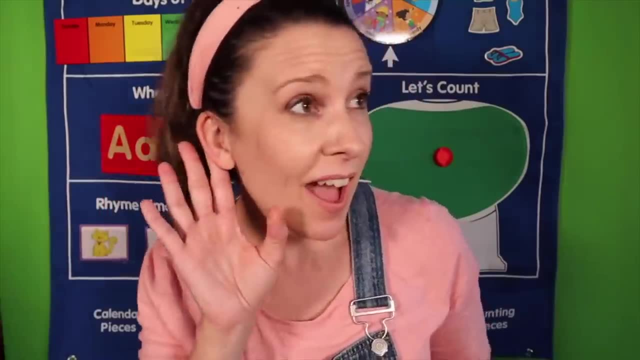 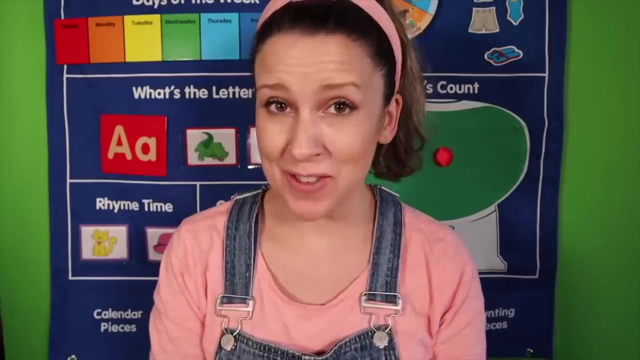 One, two, three, four, five, Five seeds were in the apple. How many seeds were in your apple if you looked inside? Wow, it's so fun learning about the parts of an apple. Great job, I'm so proud of you. 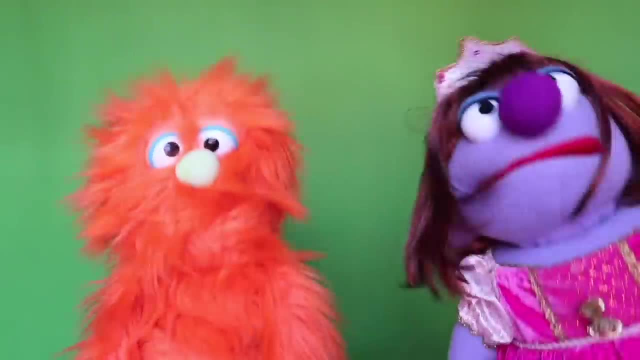 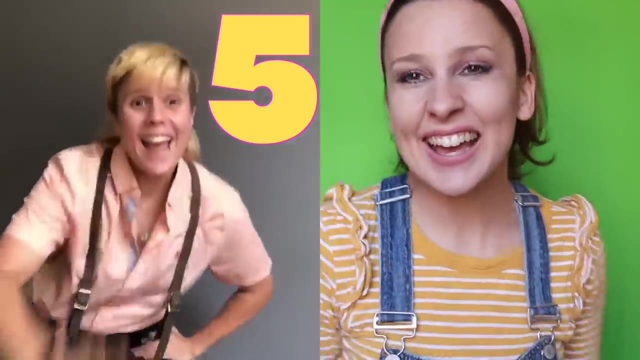 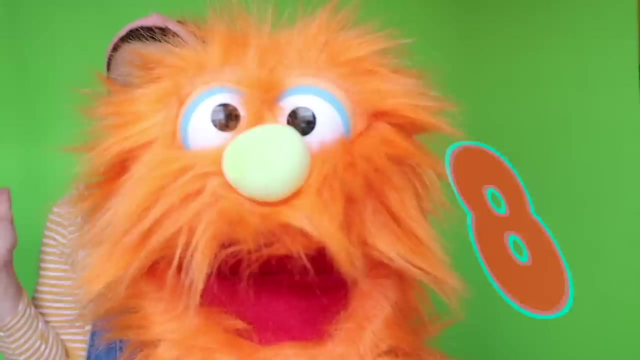 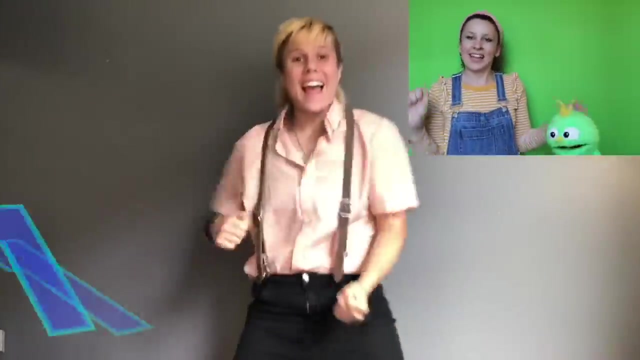 One, two, three, four, five, six, seven, eight, nine, 10.. Oh my good, Everything worked out super well. ��자 14,, 15,, 16,, 17.. What a incredible evolution. 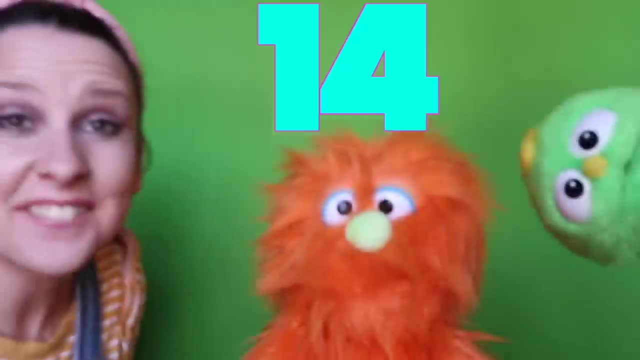 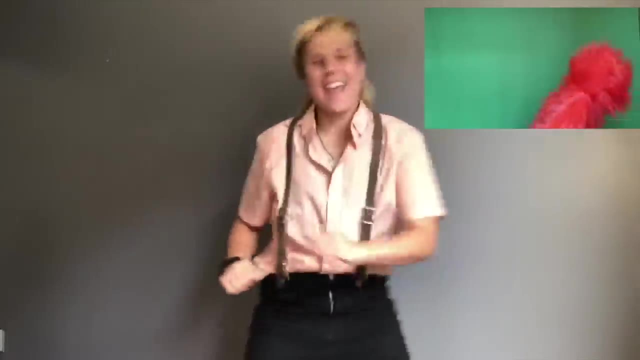 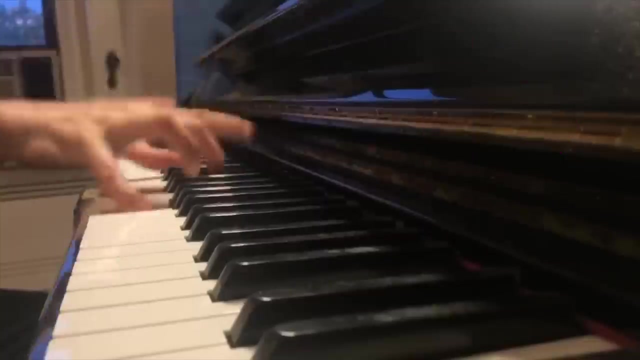 What did we learn? Where have we been? Is there anyして here? Where are you going? Let me see 15,, 16,, 17,, 18,, 19, 20.. You like Play-Doh. I love Play-Doh. 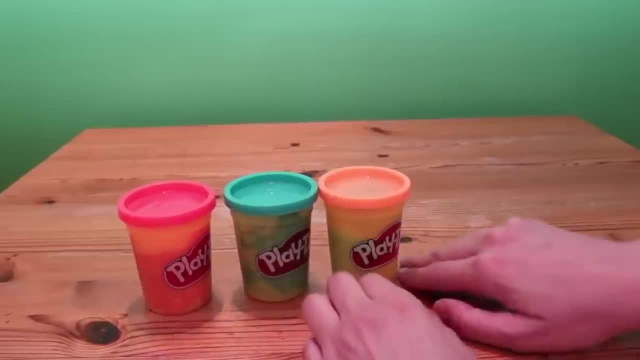 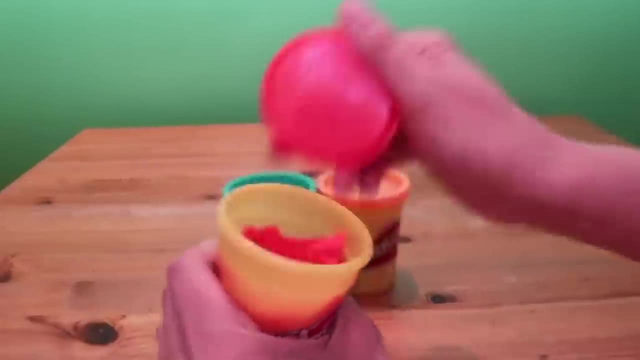 Do you have Play-Doh at home? Cool, you can even make Play-Doh. Hey, since we're learning about apples, let's make an apple out of Play-Doh Open. Okay, we gotta take some out. Pull it out. Oh, good job. 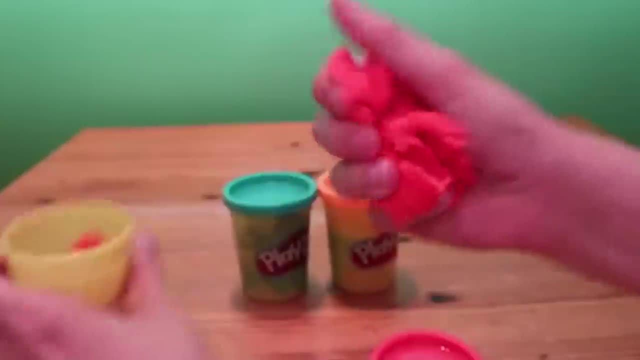 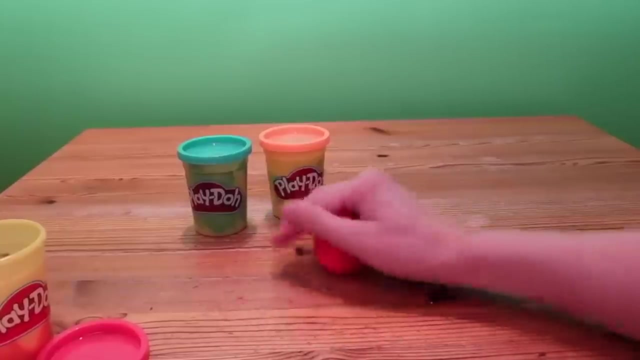 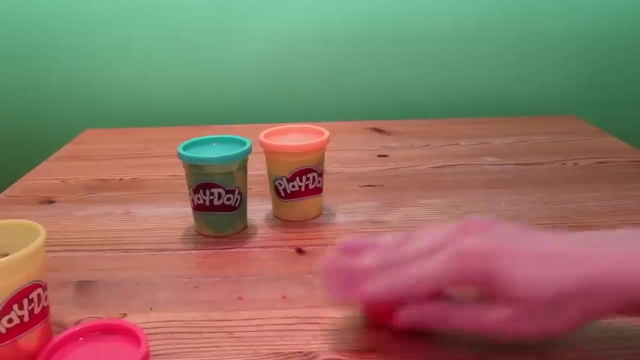 I'm gonna take a lot of Play-Doh out. Okay, now I'm gonna roll it into a ball. Roll, roll, roll the Play-Doh, Roll, roll, roll the Play-Doh, Roll, roll, roll the Play-Doh. We are rolling Play-Doh. 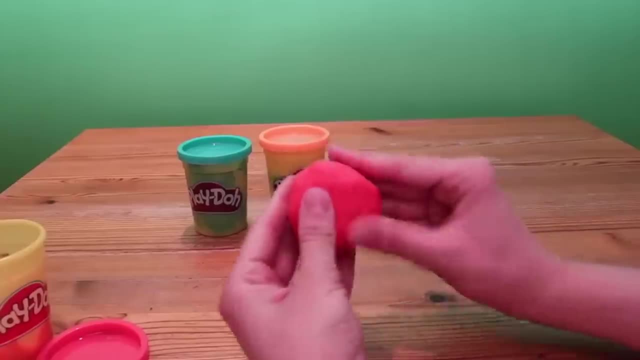 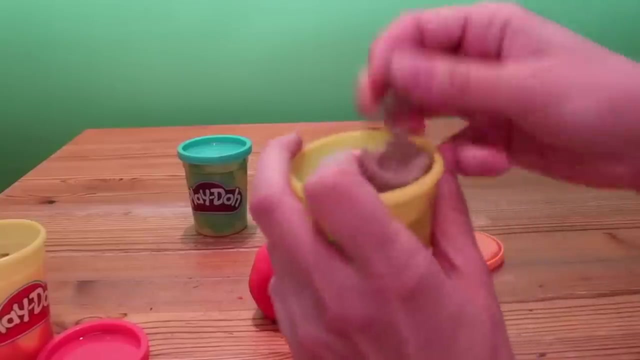 Oh, it's kind of starting to roll. It's starting to look like an apple Hooray. Okay, let's see what color this is. Oh, I made some brown Play-Doh here so I can do a stem. Remember, we learned about the stem. 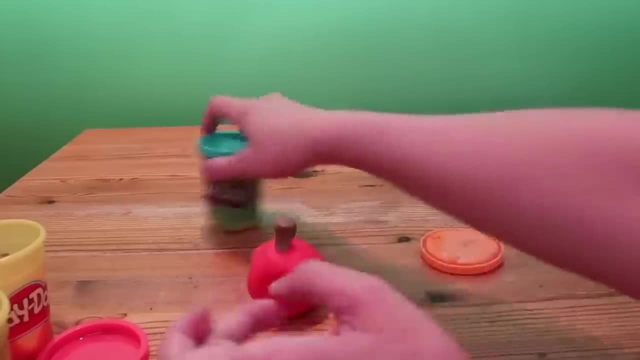 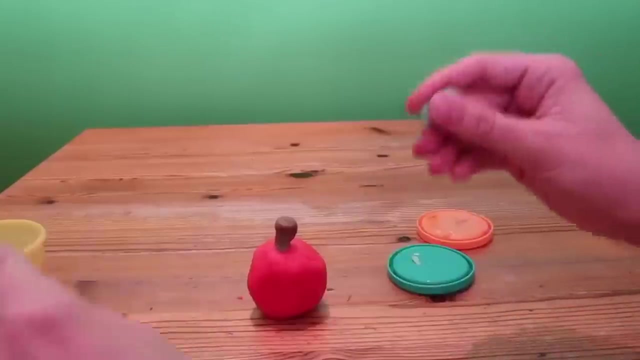 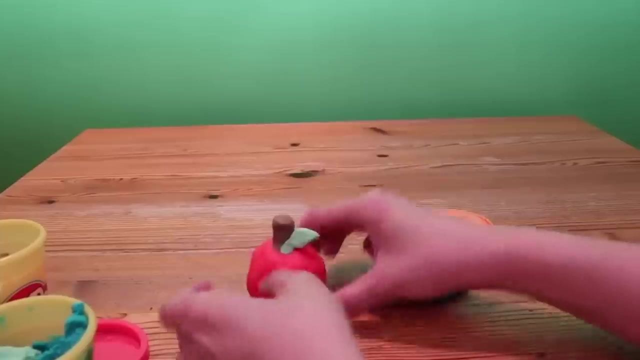 Put on the stem. Wow, it's starting to look like an apple. That is cool. Oh, yay, Here's some green for the leaf. Sometimes a leaf comes off the tree when you pick the apple, so put the leaf right by the stem. We made an apple. That was so much fun. 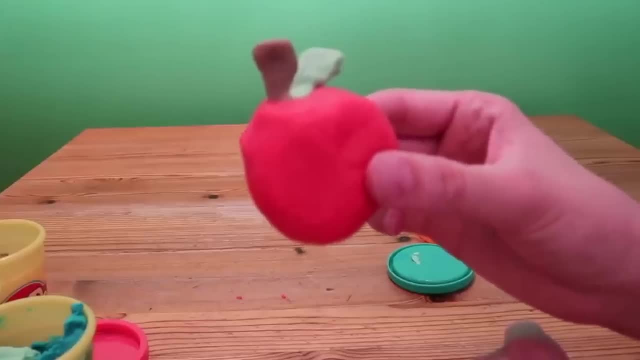 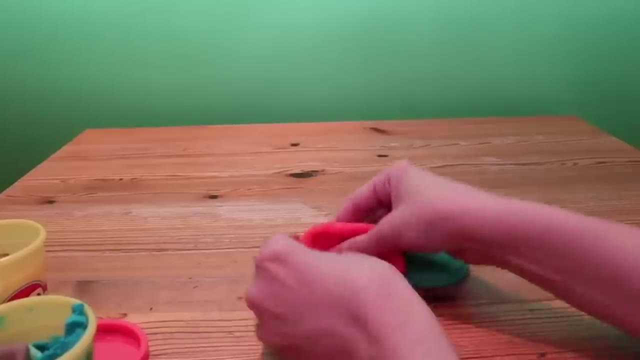 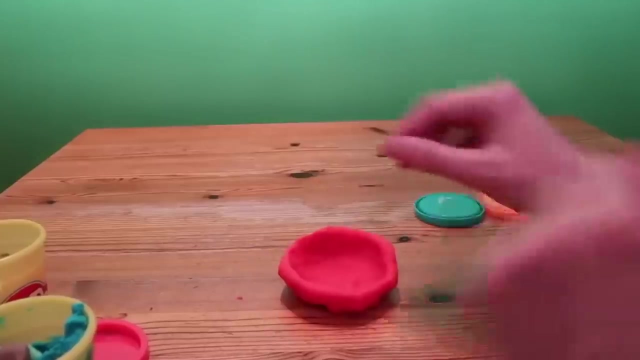 What do you like to make out of Play-Doh? Awesome, One thing I like to make out of Play-Doh is a bowl. I'll show you. It's so much fun to make a bowl out of Play-Doh. Making a bowl, Making a bowl. And then I like to make little balls. 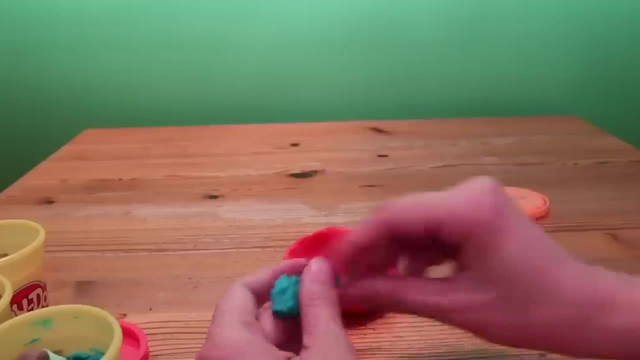 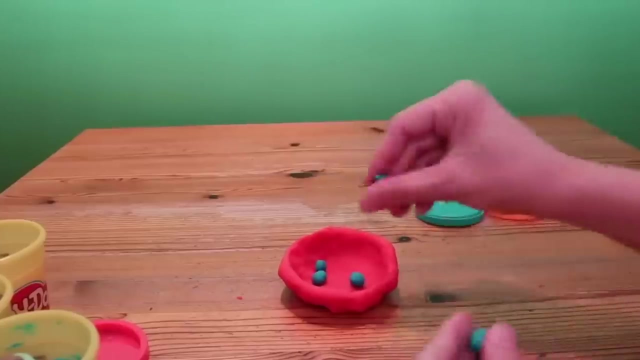 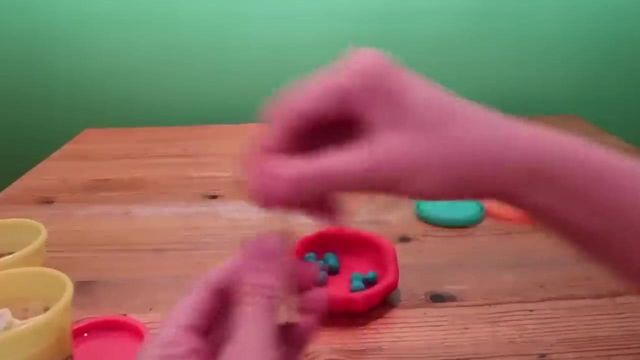 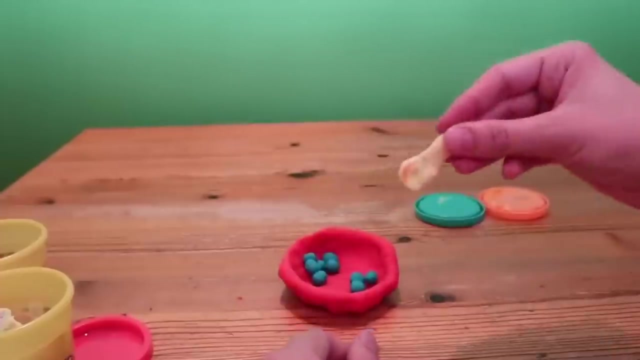 and pretend that it's cereal. Cereal Making pretend cereal. Do you like cereal? I like cereal. Making a bowl out of Play-Doh is fun. Now I'm going to make the spoon. Gotta use a spoon. Wow, here's a little spoon. I love playing with Play-Doh. 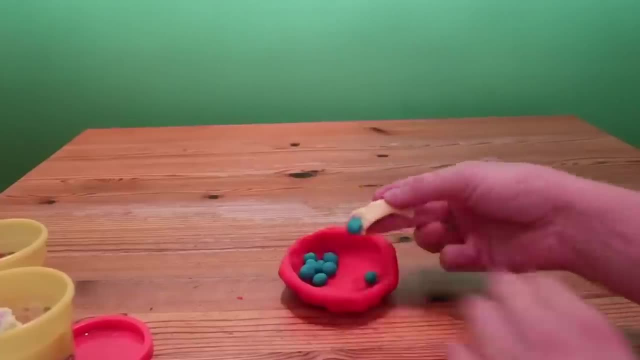 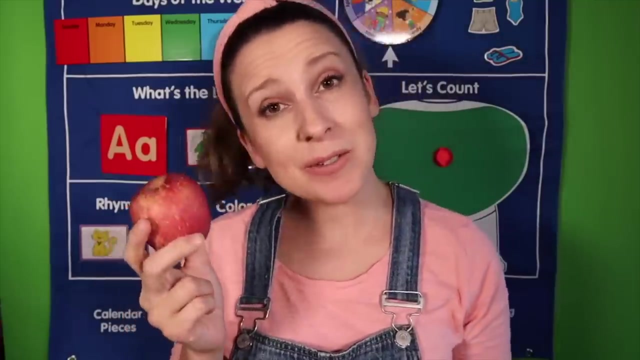 Oh, picking up the cereal with the spoon, So fun. Let's explore the apple with our five senses. Do you have an apple at home you can use? If not, you could try another fruit or any food. We can smell the apple with our nose. 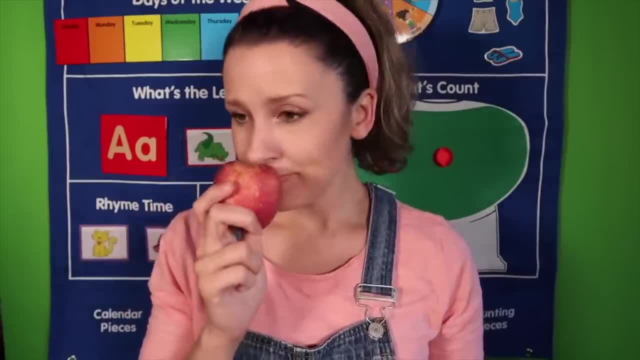 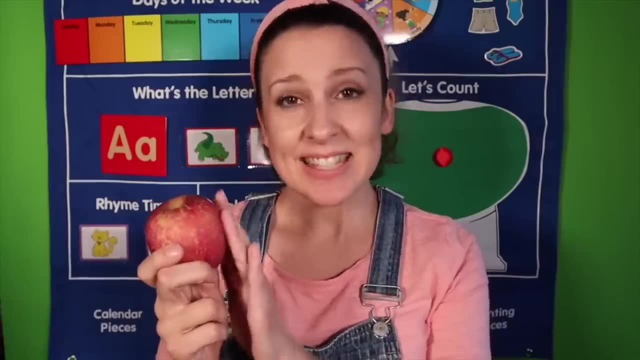 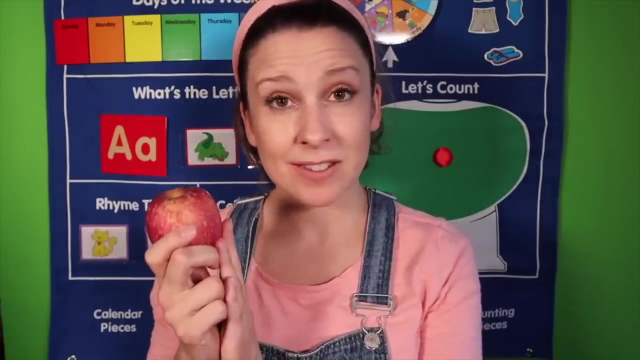 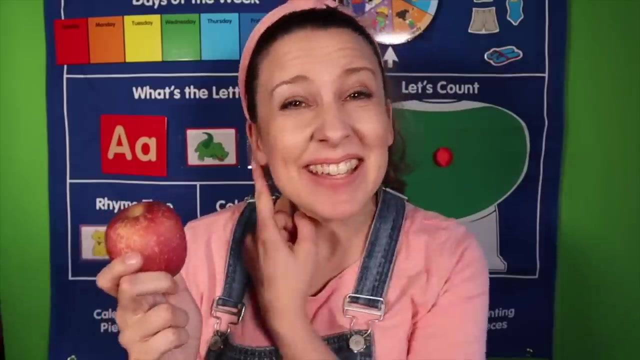 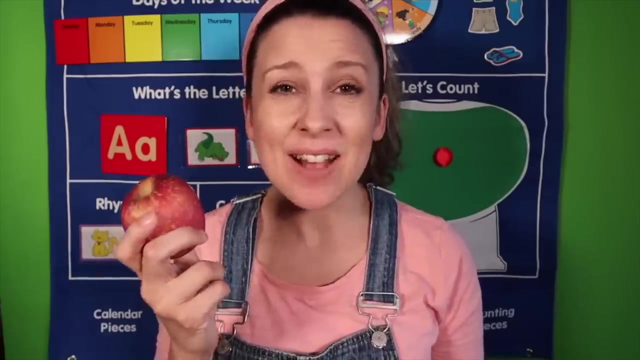 It smells fresh and sweet. We can feel or touch the apple with our hands. This apple feels smooth, A nice smooth apple. How does your apple feel? Wow, I can listen to the apple with my good job ear. There's no sound, But if I bite the apple it makes a sound. Listen. 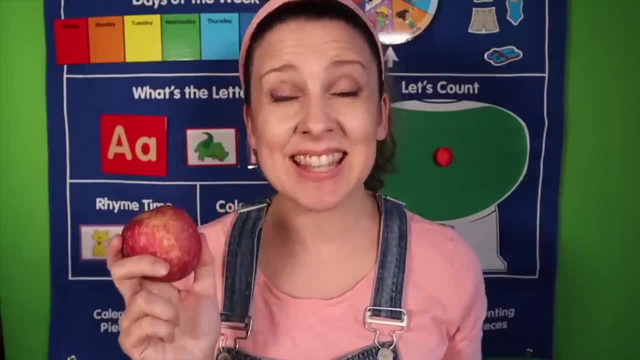 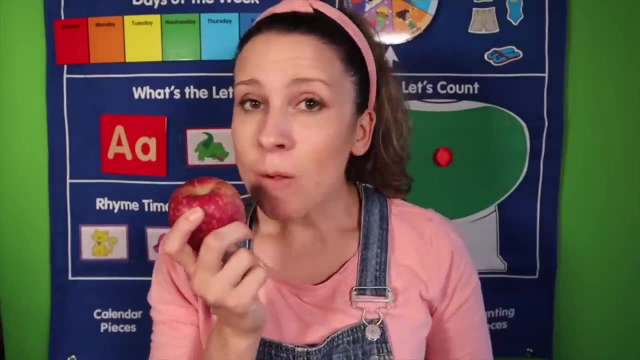 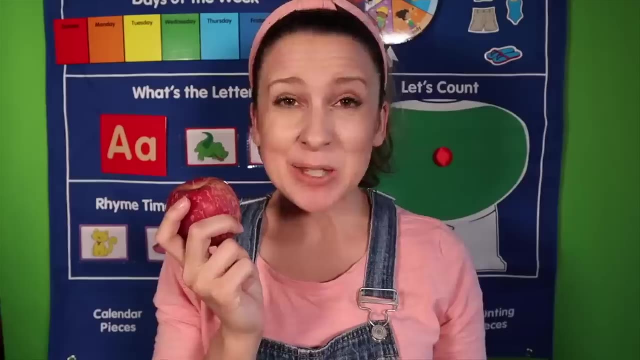 Do you hear the chewing? I can taste the apple with my mouth, Good job. Do you hear the chewing? I can taste the apple with my mouth, Good job, Mmm. The apple tastes really yummy and it's very juicy and sweet. It was crunchy, I can. 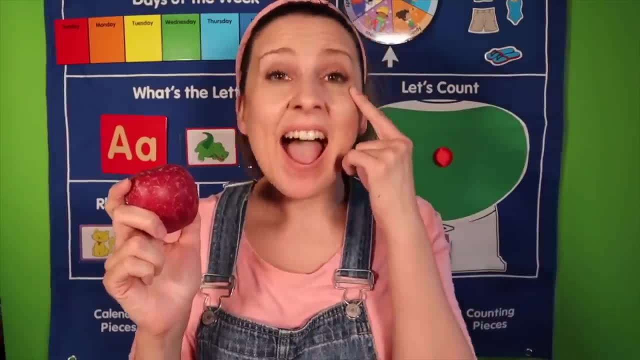 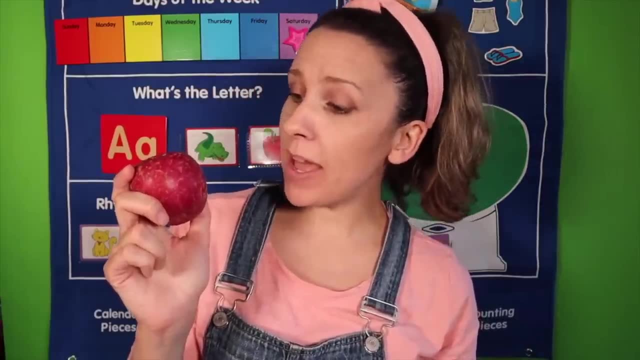 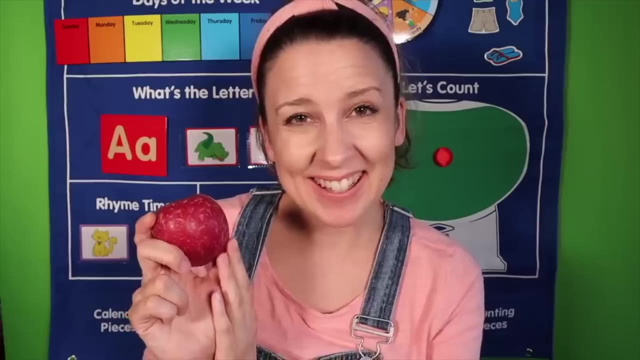 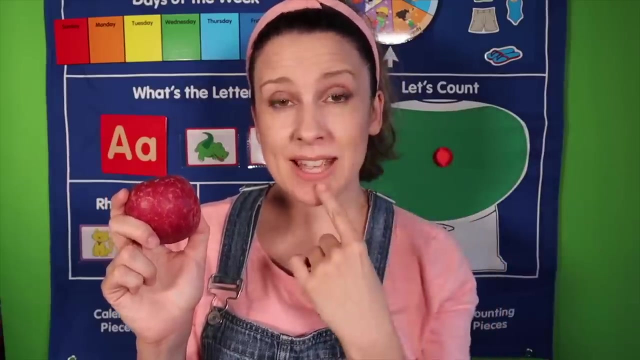 look at the apple with my eyes. Good job, Can you look at your apple? My apple looks red and a little bit brown and it looks shiny. How does your apple look? It's so fun to explore an apple with our five senses. We looked at the apple, we tasted the apple. 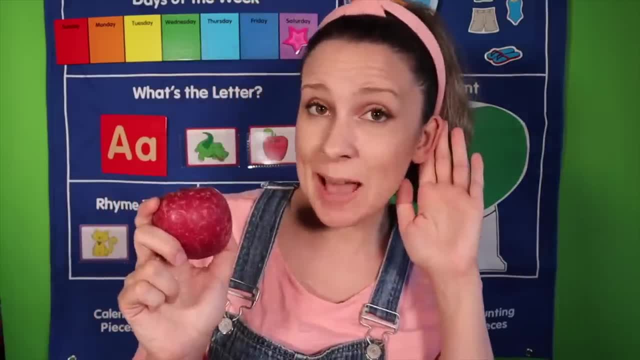 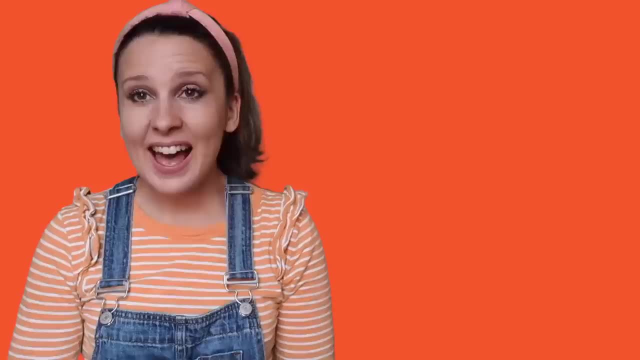 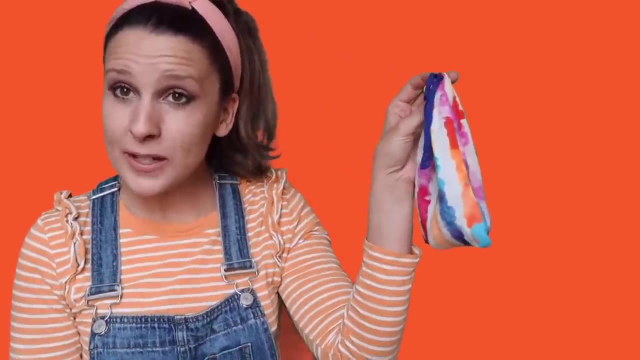 we smelled the apple, we listened to the apple and we touched the apple. Wow, Good job, High five. I have something special to show you. It's in this little bag. Let's open it. Can you say open, Open, Open the bag, see what's inside. 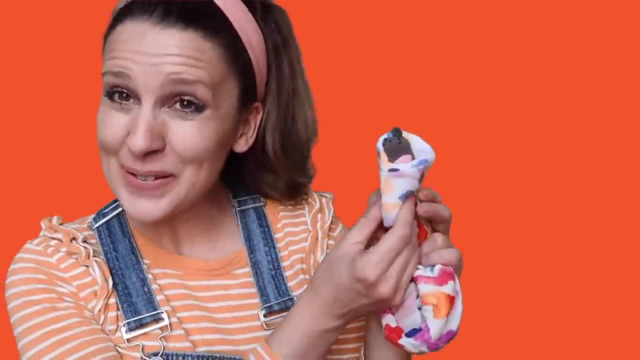 Oh, Ah Ah. It's an apple. Ah, Ah, Open with all your hands, Look All the ways and It's a mouse. Oh shh, the mouse is sleeping, But it's time for the mouse to wake up. 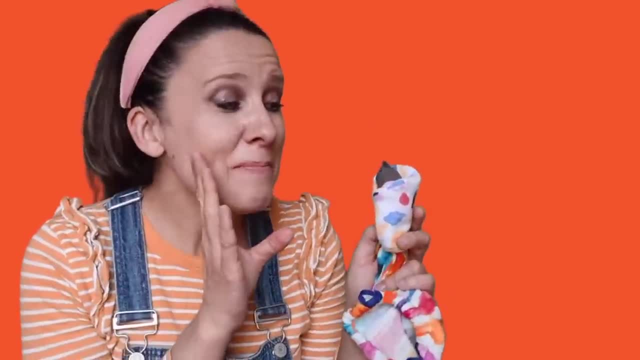 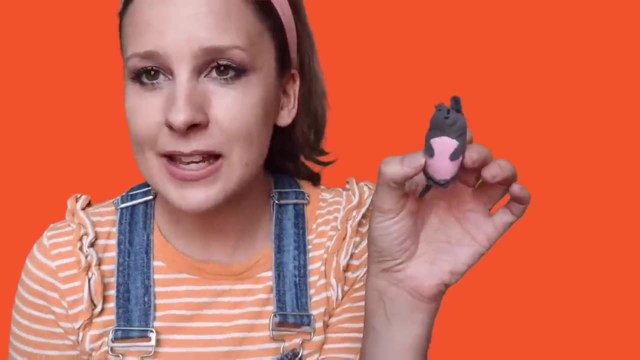 Let's say: wake up mouse. One, two, three, wake up mouse. Oh, good morning, Hi, I'm a little mouse, I want to climb up the clock. Can you sing Hickory, Dickory Dock? Sure, we can sing that. 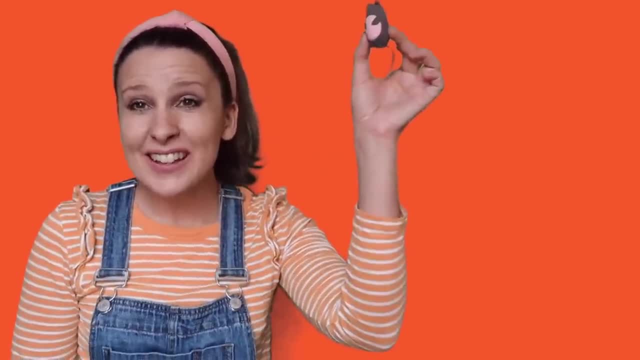 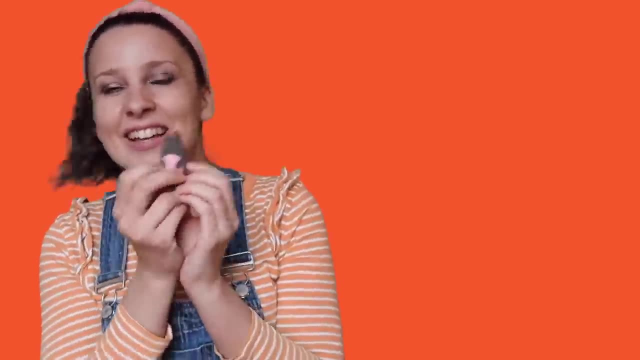 Hickory dickory dock. the mouse went up the clock. The clock struck one. the mouse went down. Hickory dickory dock. tick-tock, tick-tock, tick-tock. Hickory dickory dock. That was so much fun. 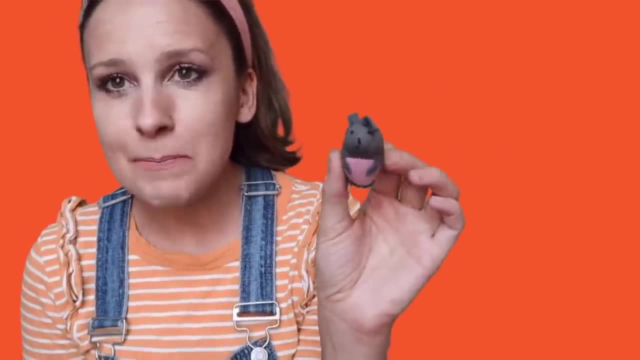 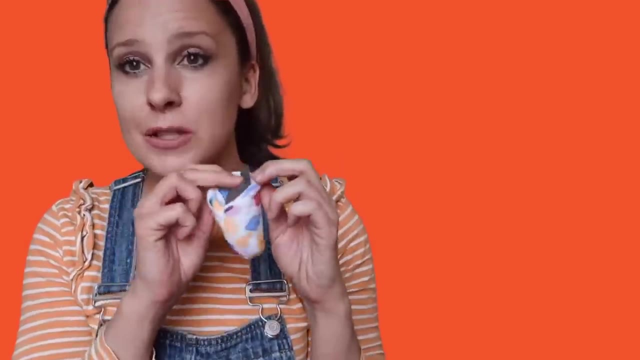 Thank you for singing my song. I'm going to go back to sleep now. Good night, Oh shh, the mouse wants to go back to sleep. Let's whisper. Okay, let's put the mouse back in the little bag. 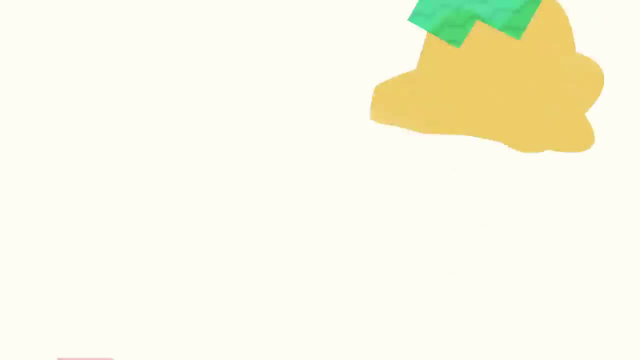 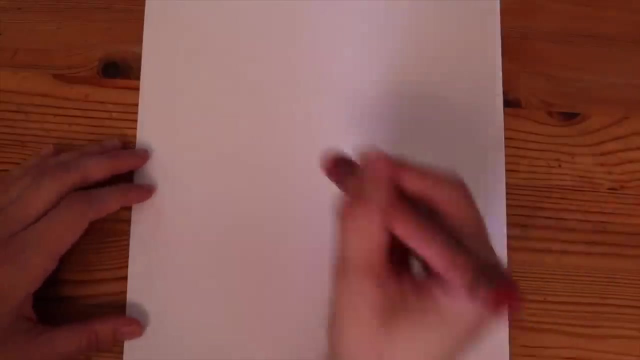 Good night mouse Say good night mouse Shh. Next, I think I'll draw an apple. Do you want to draw an apple with me? Yay, Okay, here's the apple shape. Oh, hello apple. 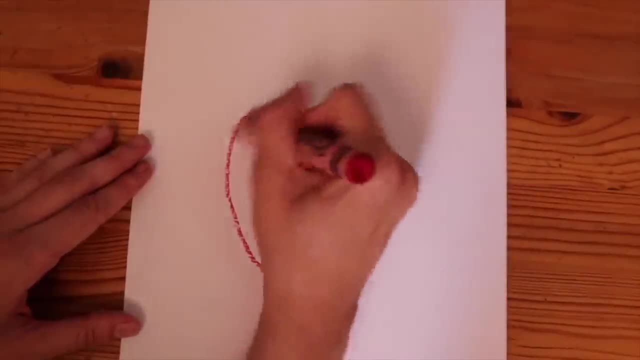 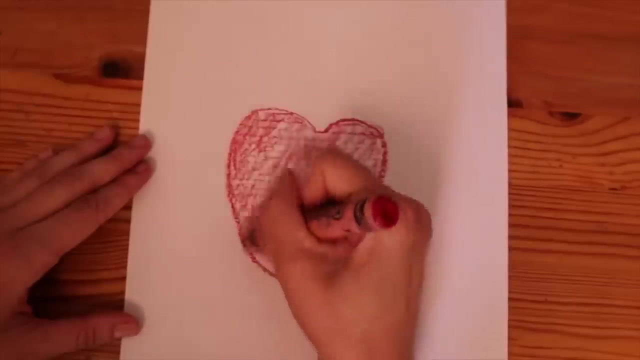 I'm using a red crayon. I color it in. Sometimes it goes outside the lines, and that's okay. It doesn't have to be perfect, It's wonderful because I made it. It doesn't have to be perfect, It's okay. 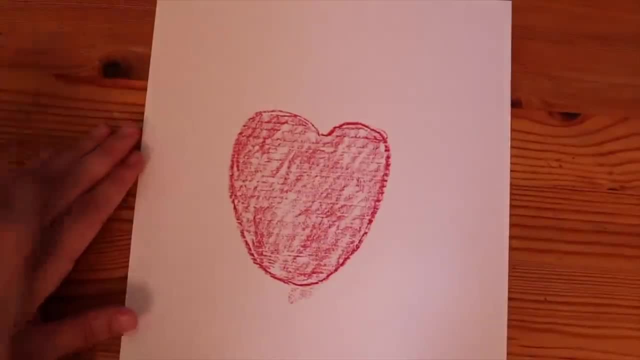 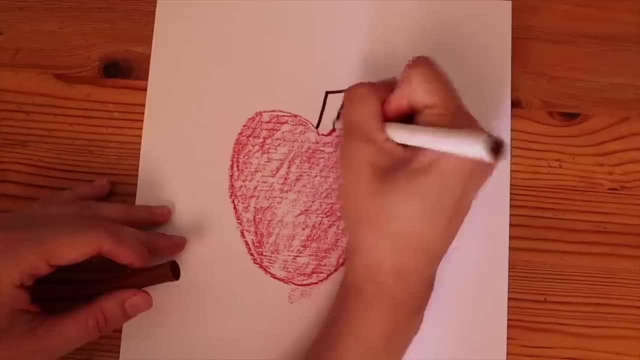 You can make mistakes. Wow, look at that apple. It almost looks like a heart. Now I'm going to do a stem. I have a brown marker. There's my stem. Color it in color, it in color it in. 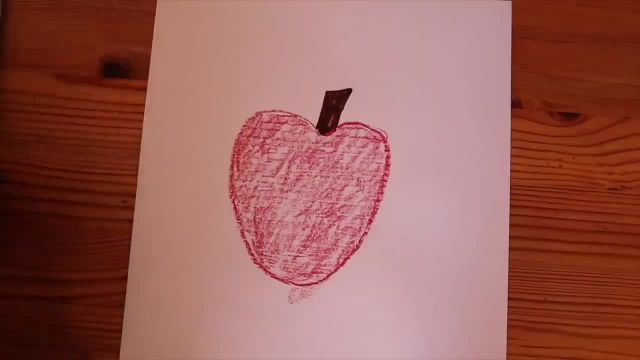 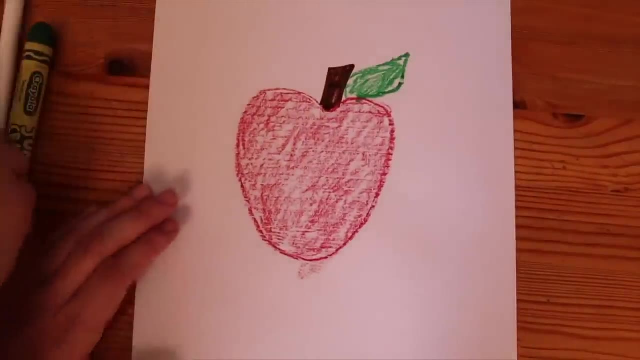 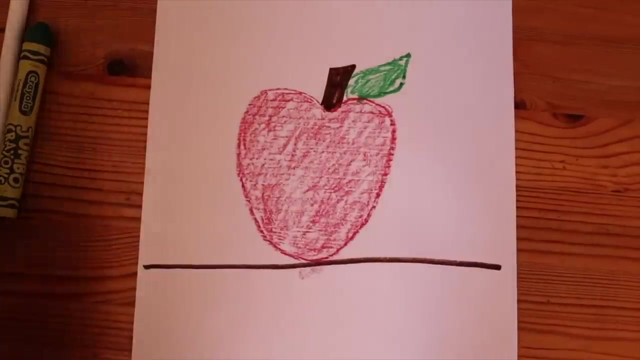 Now for the leaf. I think I'll use a green crayon. Here's the leaf And that's my apple. Maybe I'll put it on a table. Just draw a little table. Yay, I drew a yummy apple. Did you draw an apple? 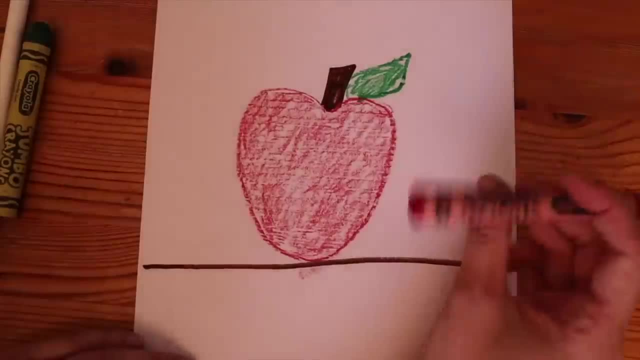 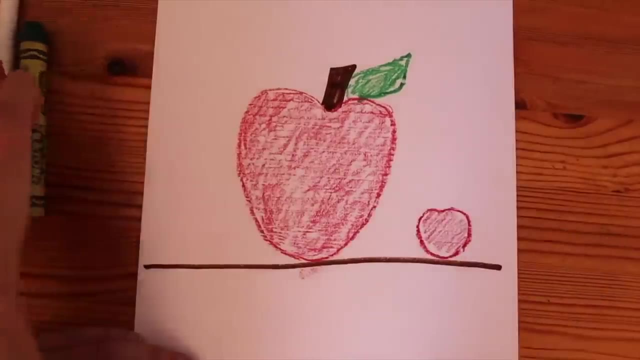 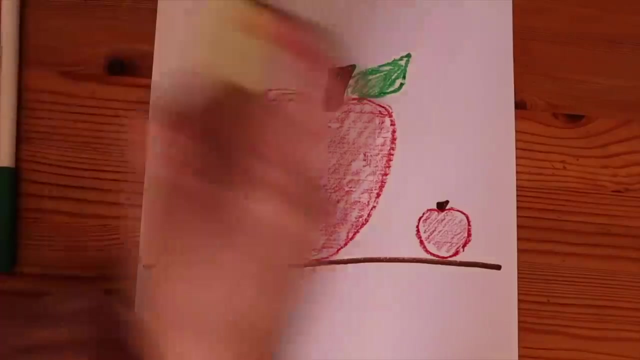 That was so much fun. This is a large apple. Maybe next to it I'll draw a small apple. Oh, I'm just a little tiny apple. There are apples that are very small called crab apples, And a lot of people like to use them for jelly. 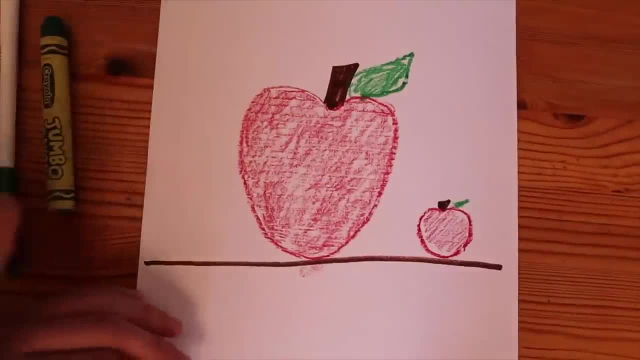 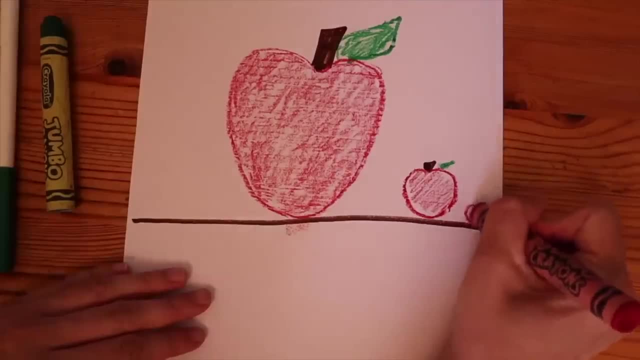 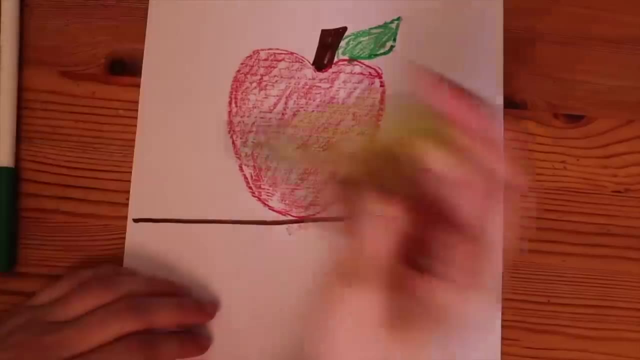 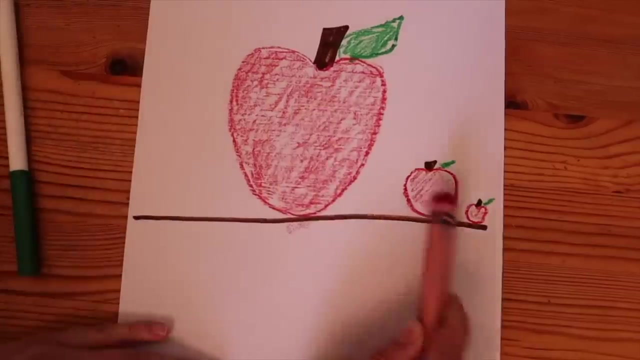 Do you think we could do it? I'm even smaller. Hee, hee, hee, hee. So small, Teeny weeny apple. Oh, that's fun. Now this one's large, this one's medium and this one's small. 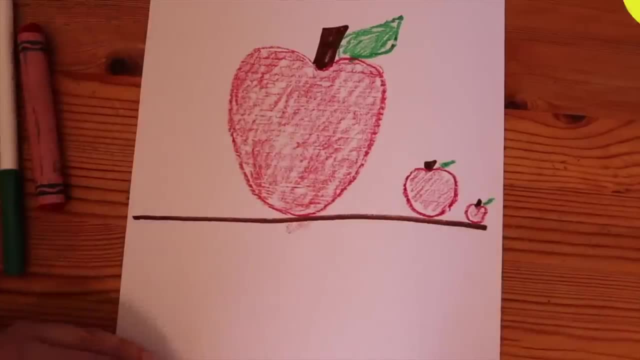 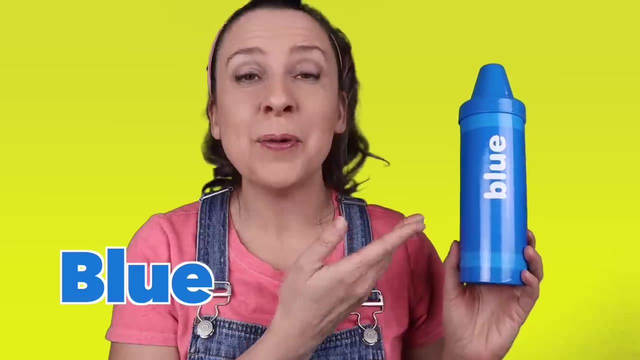 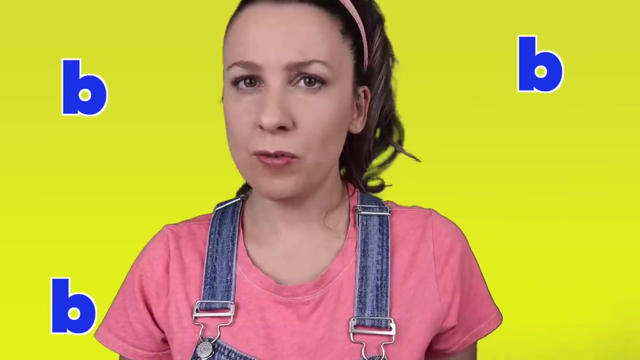 That was so fun. Thanks for drawing apples with me. I loved it. Our next color is blue. wow, Blue begins with B. Can you do a B sound? Buh, buh, buh. Can you do a fast, silly B sound? 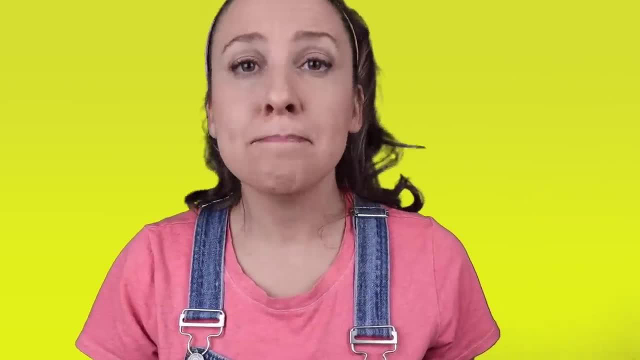 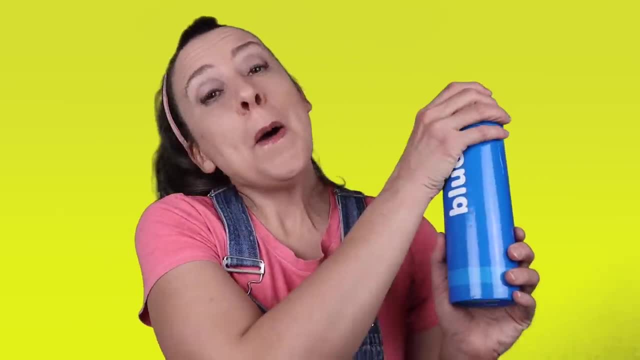 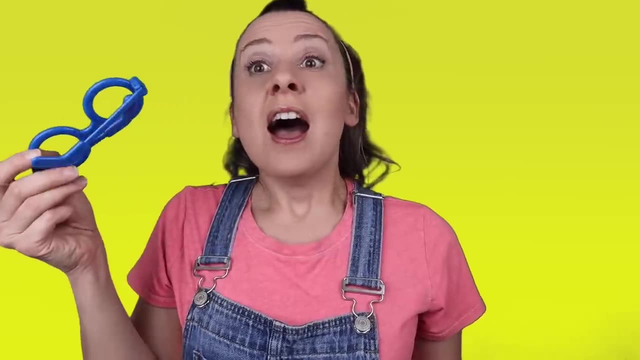 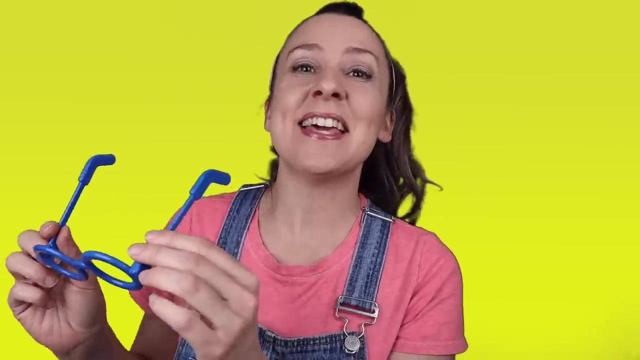 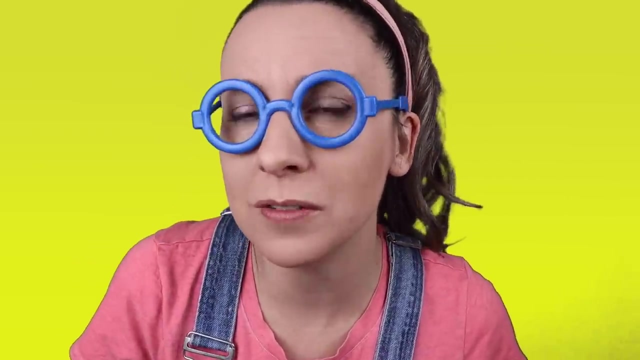 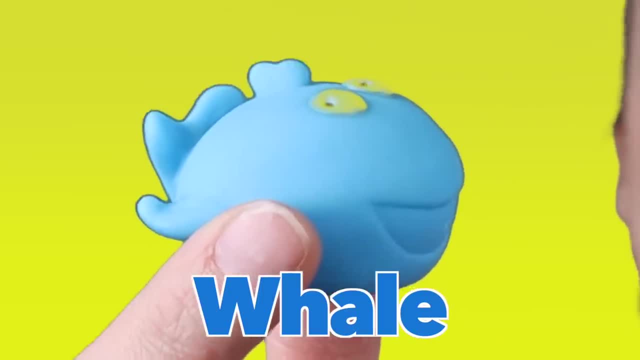 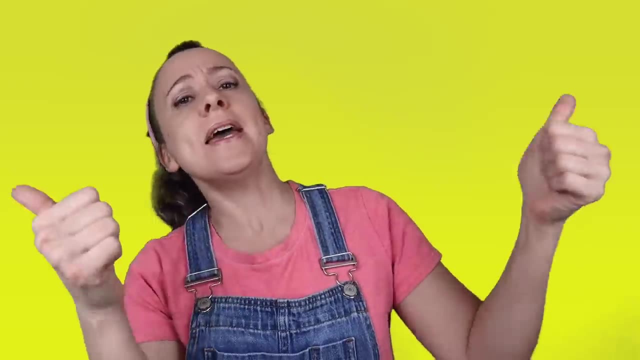 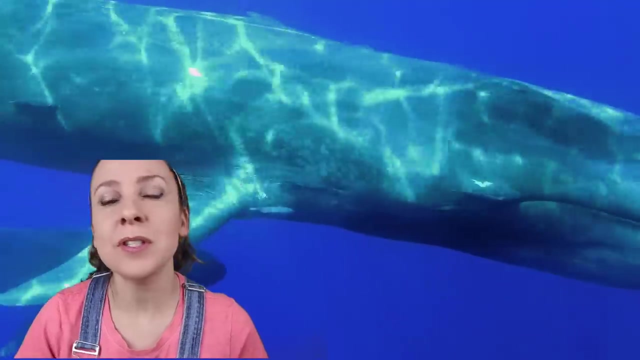 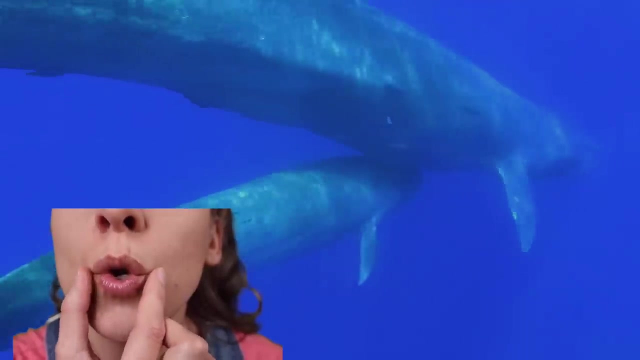 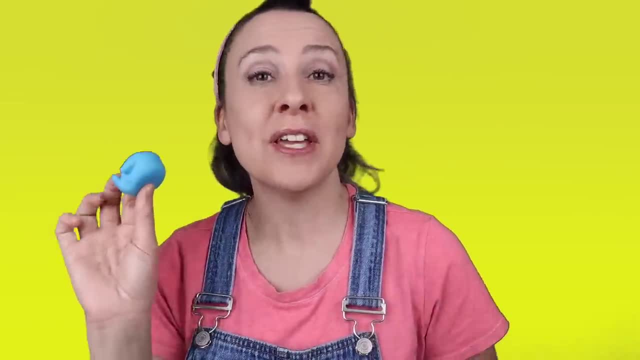 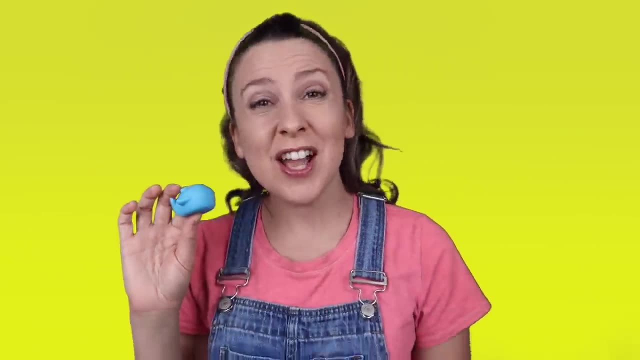 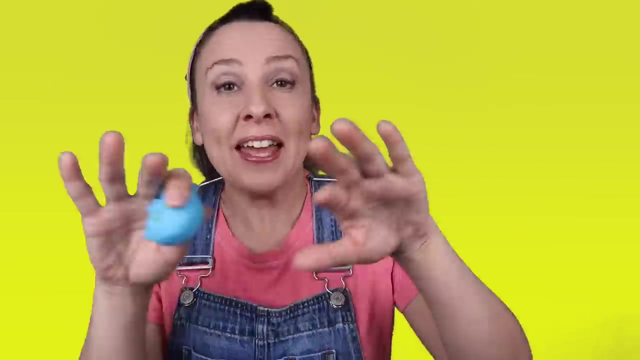 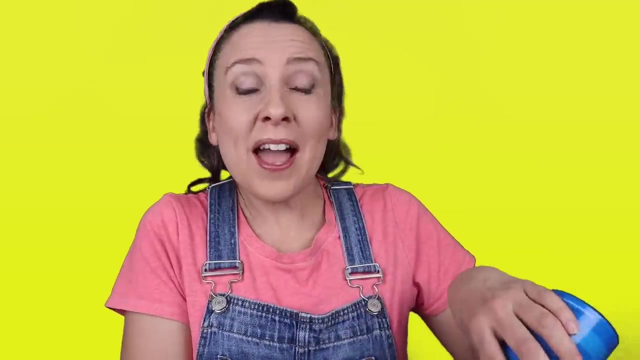 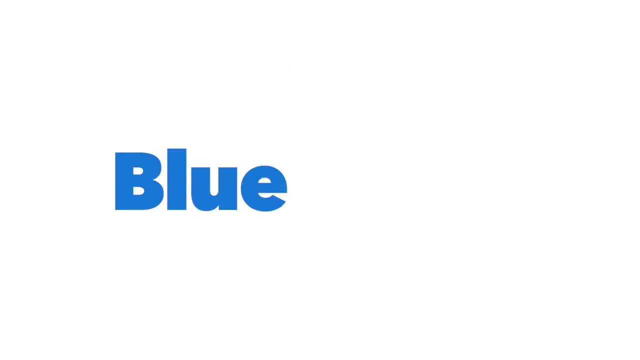 Whale. let's pretend we're a whale blowing out of our blowhole. Oh, good job. Swim, swim, Can you swim around the room? Swim, Wow, a blue boat. Blue and boat both start with B: Blue boat. 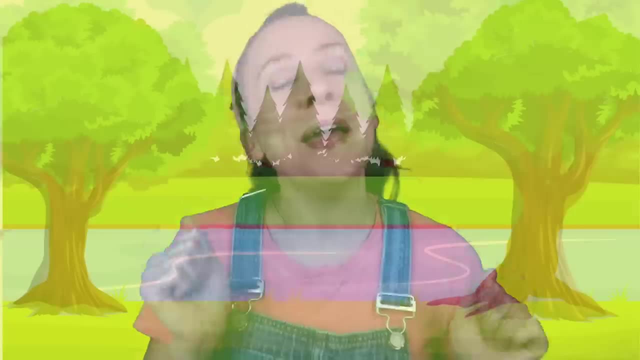 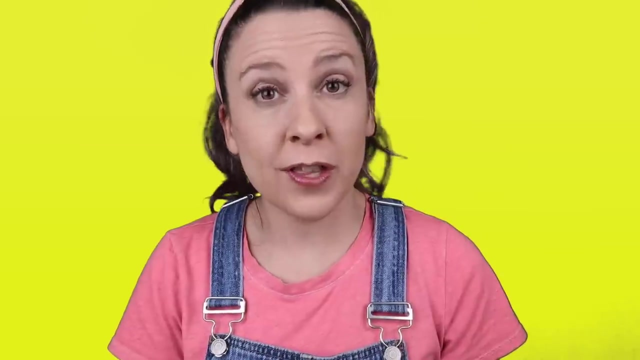 Row, row, row your boat gently down the stream, Merrily, merrily, merrily, merrily. life is but a dream. That was so fun. Now you fill in the words and we'll pretend to see a crocodile. 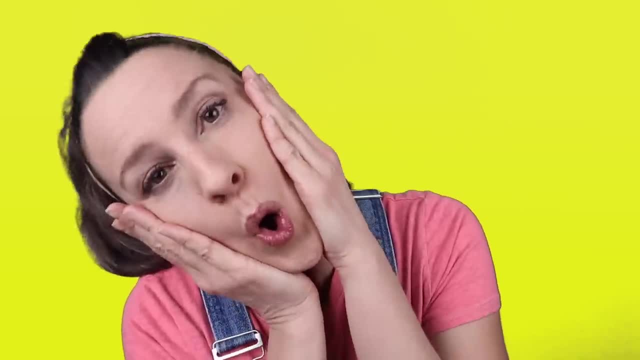 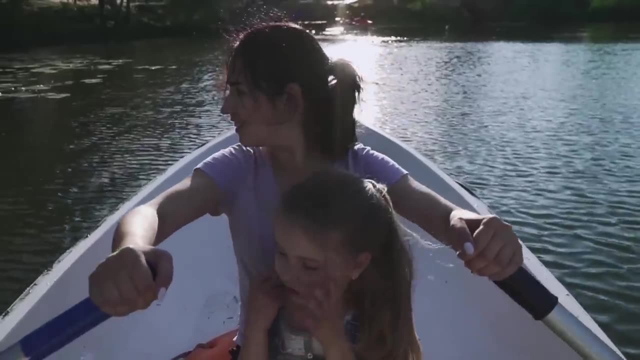 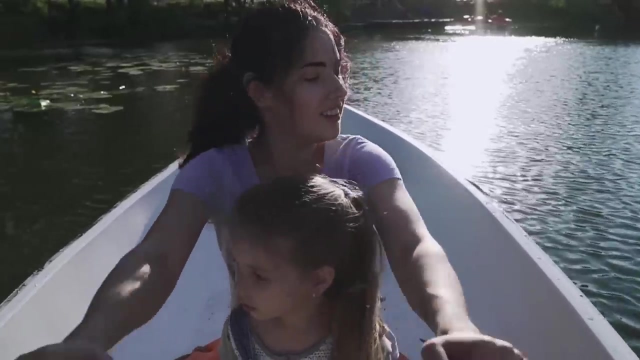 Oh, no, Uh-oh, Can you say that? Uh-oh, uh-oh, uh-oh, Row row, row your boat, Row row, row your boat gently down the stream. If you see a crocodile, don't forget to scream. 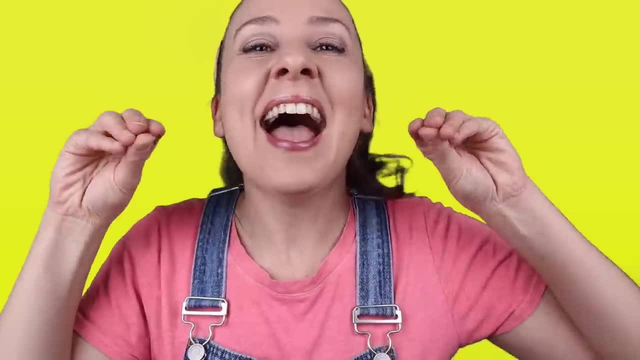 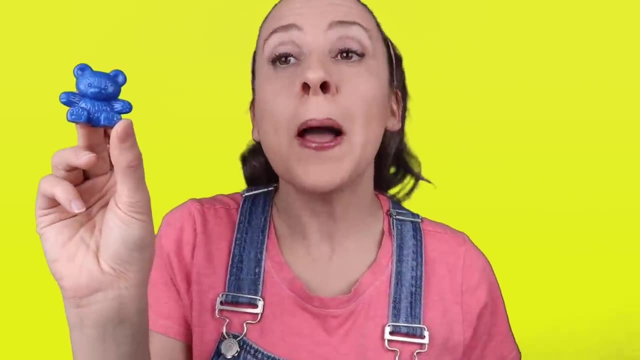 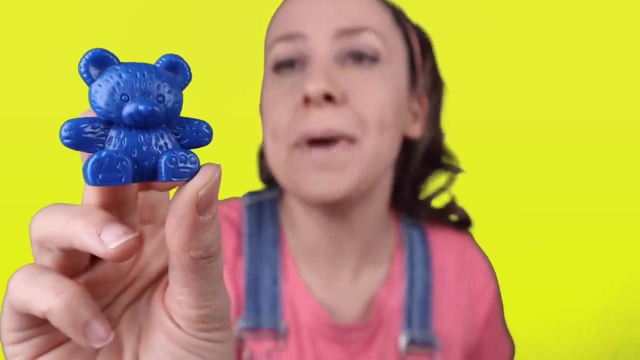 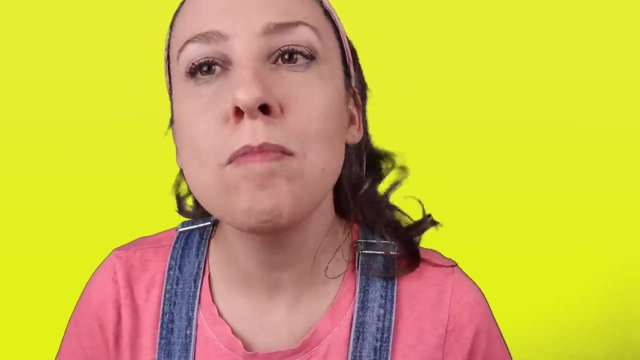 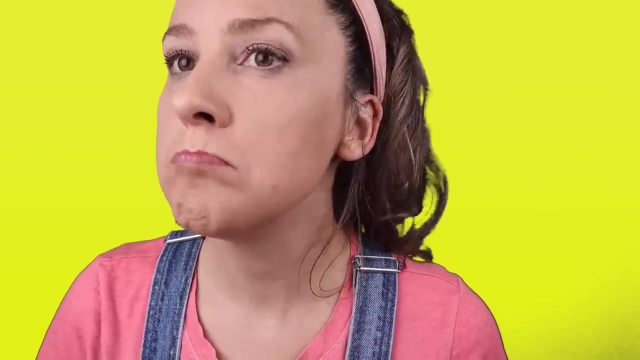 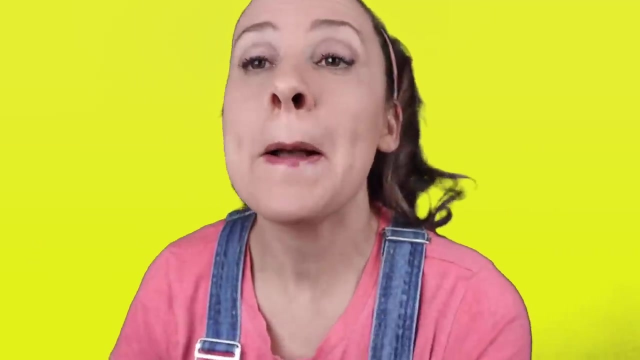 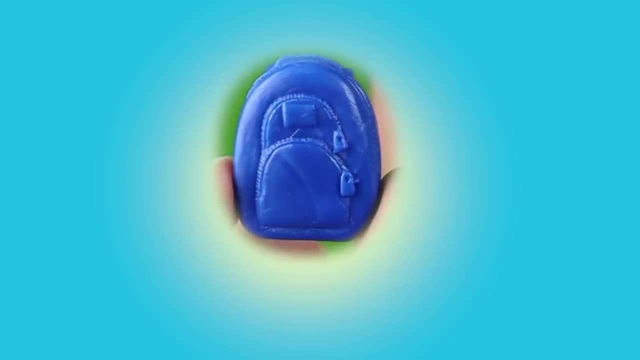 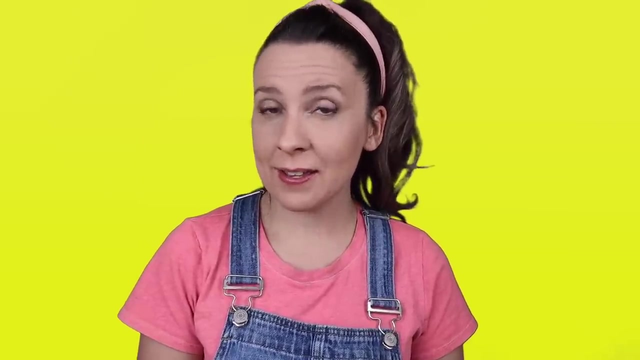 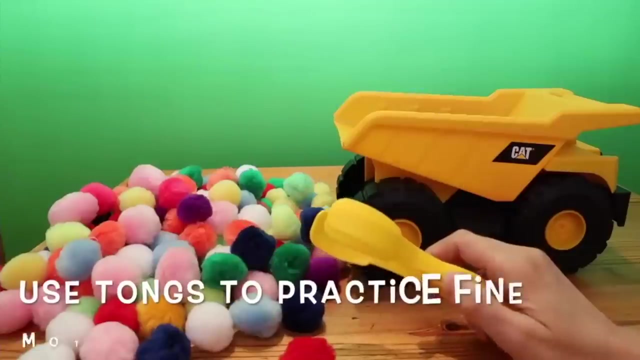 It's a blue backpack. Wow, Have you ever worn a backpack? B-B-Backpack also starts with the letter B- B-B-Backpack. Our friend Georgie's doing an art project with red puff balls. Let's fill up the truck and bring the puff balls to Georgie. 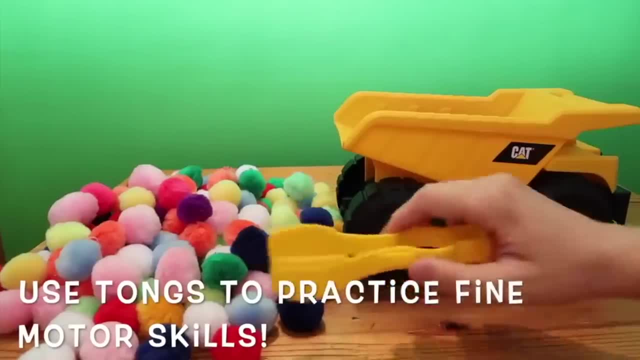 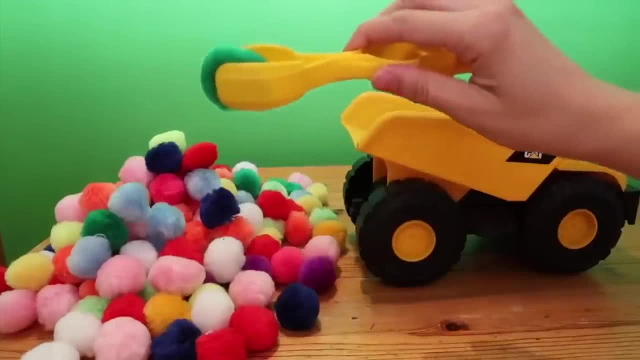 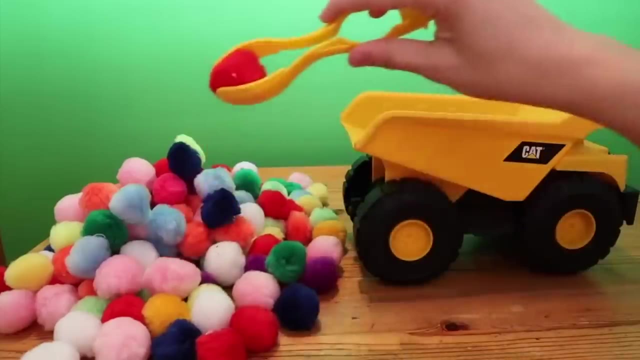 He needs red puff balls because he's making an apple project. Should this one go in? Yeah, it's red. Does this go in? No, we want the red puff balls. Does this go in? Yeah, This is red. This is red. 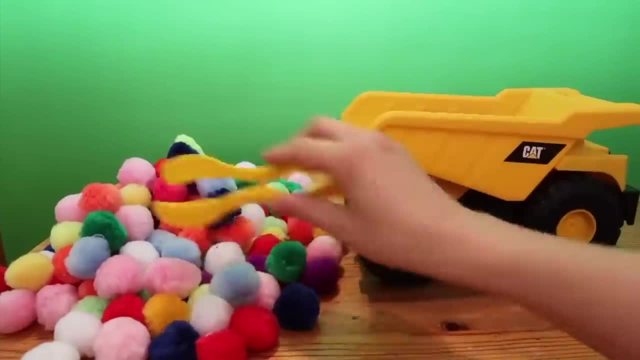 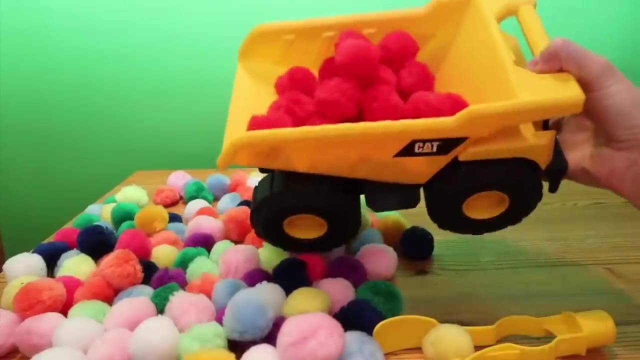 Does this go in? No, it's blue. Does this go in? No, it's green. We filled up the truck with red puff balls. Yay, Awesome job. Now we can bring them to Georgie. Can you help me? 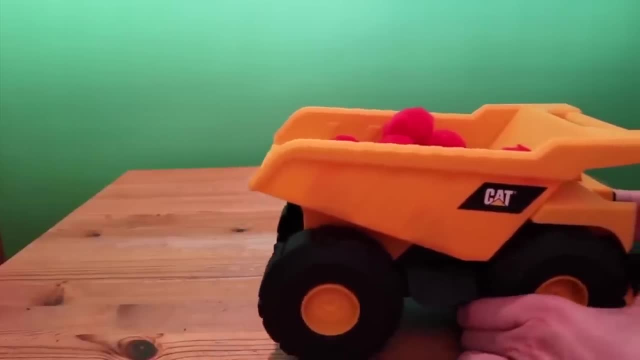 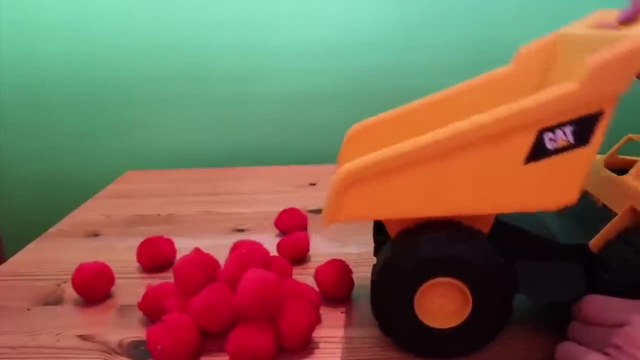 Can you help me dump out the puff balls? Say out, and I'll dump them out. One, two, three out. Yay, Oh, we dumped them out. Great job, So many puff balls for Georgie's apple project. 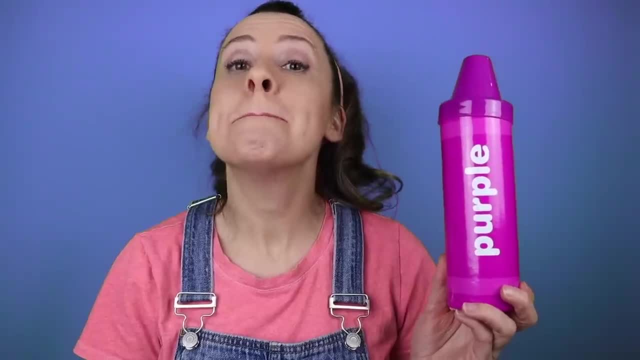 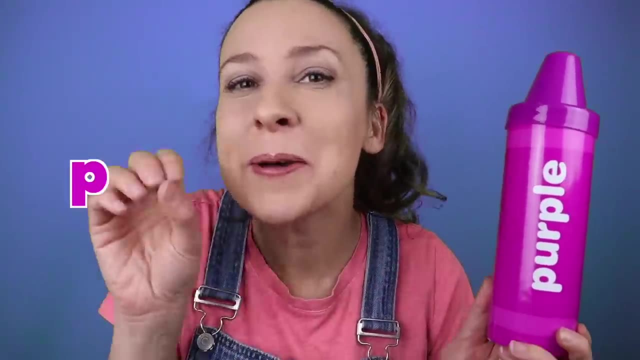 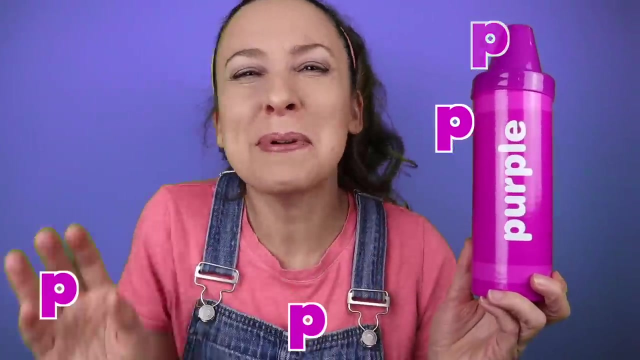 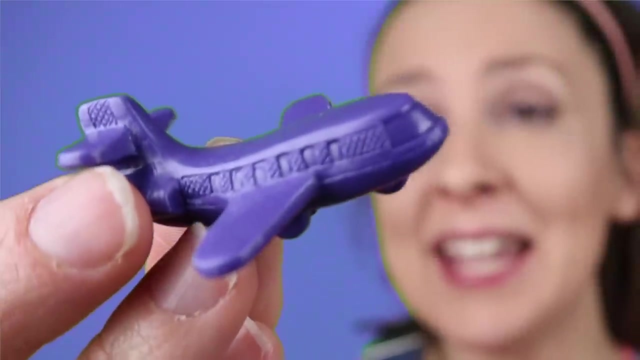 What's this color? It's purple. Wow. Purple begins with P. Let's do the P sound. P-P-P-P-P-P-P. Is that some popcorn popping? P-P-P-P-P-P-P. It's a purple plane, Wow. 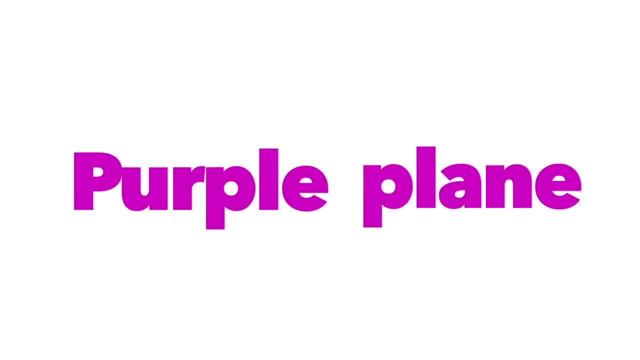 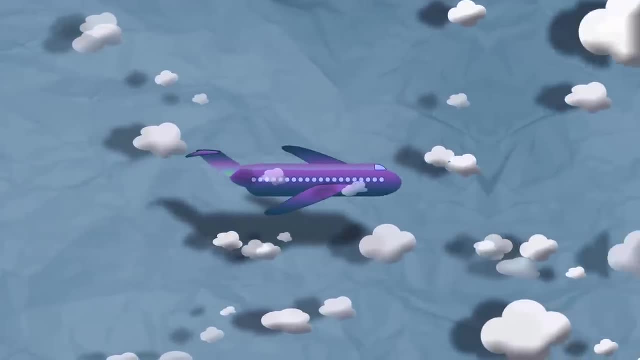 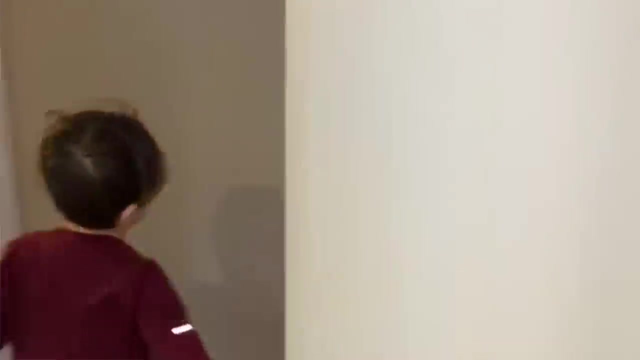 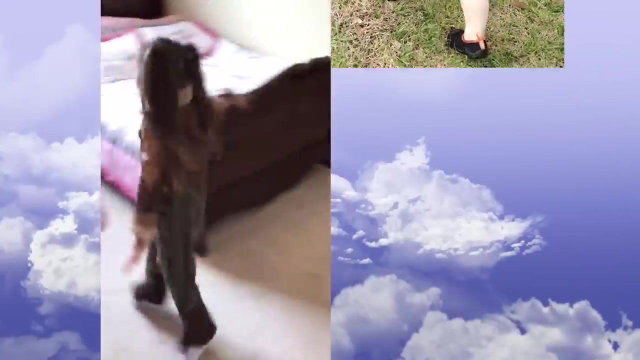 Purple and plane both begin with P- P-P-P-P-P-P-P-P. A plane can fly through the air. Can you zoom around your room like a flying plane? Zoom? P-P-P-P-P-P-P. P-P-P-P-P-P-P-P. 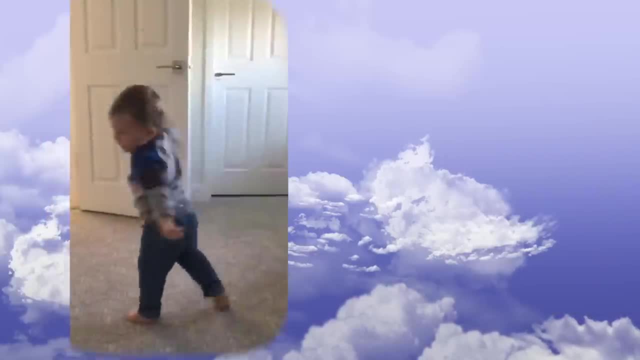 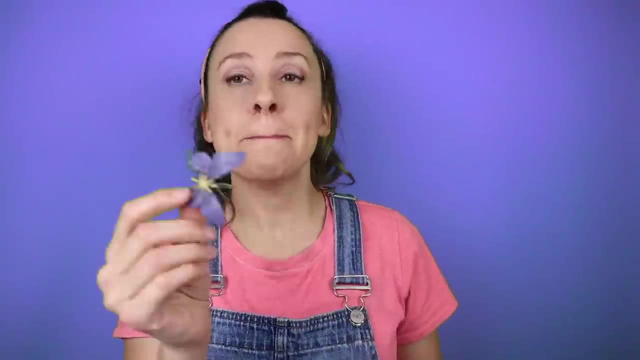 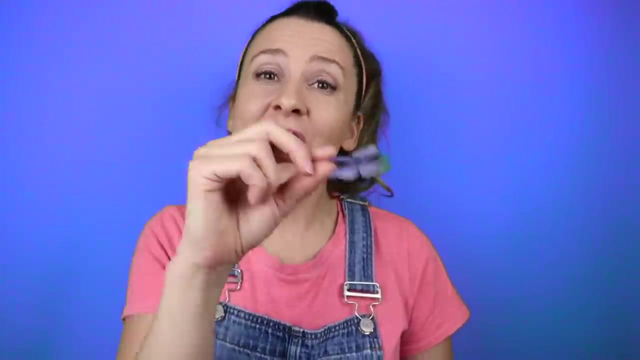 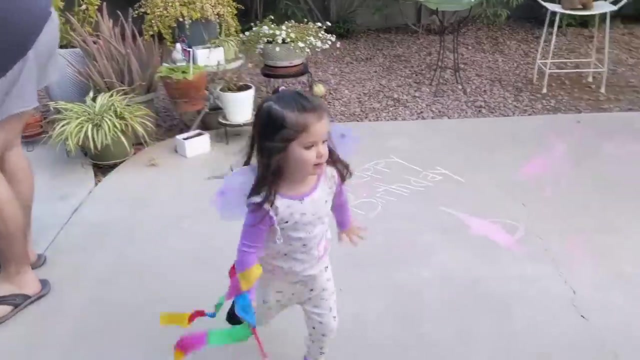 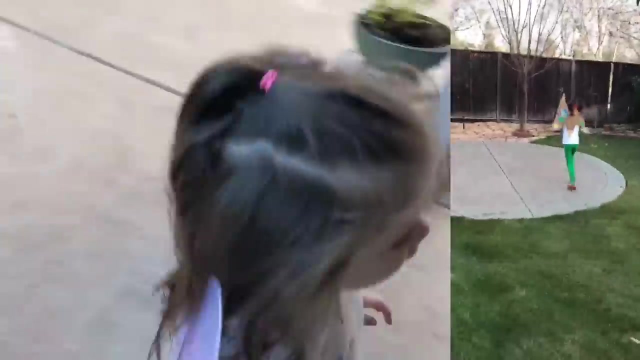 P-P-P-P-P-P. Oh wow, It's a butterfly, beautiful butterfly. Butterflies also fly. Let's pretend to be butterflies. Can you fly around with me? Good job, Fly, fly like a butterfly. Fly, fly like a butterfly Fly. 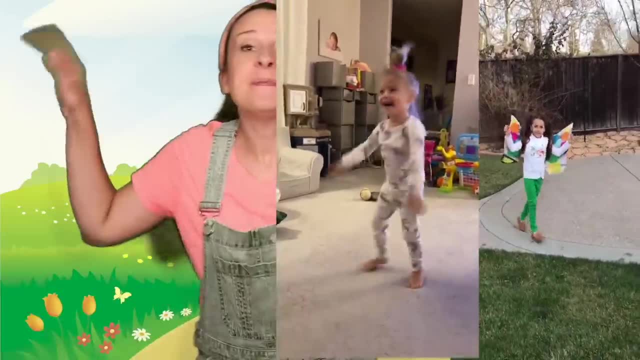 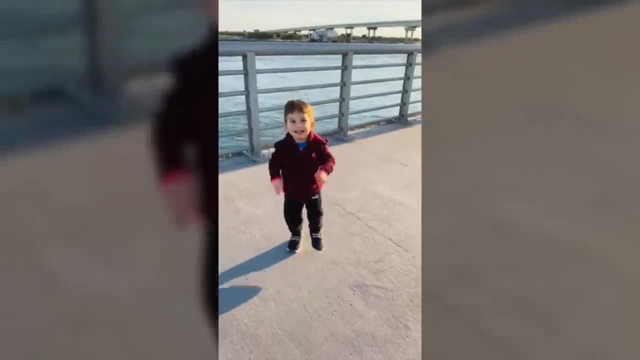 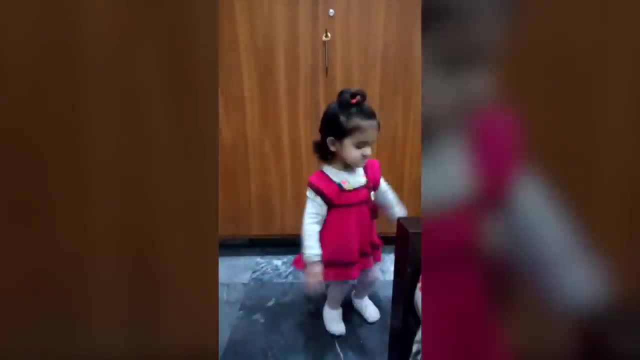 fly like a butterfly, Fly around the yard. Now let's pretend we land on a flower. Did you know that butterflies taste with their feet? Yum, yum, yum. This flower tastes yummy. Then they drink the nectar, like this Land on a flower, and drink the nectar up Land. 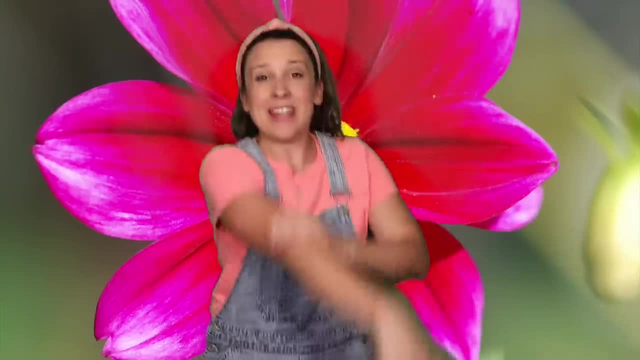 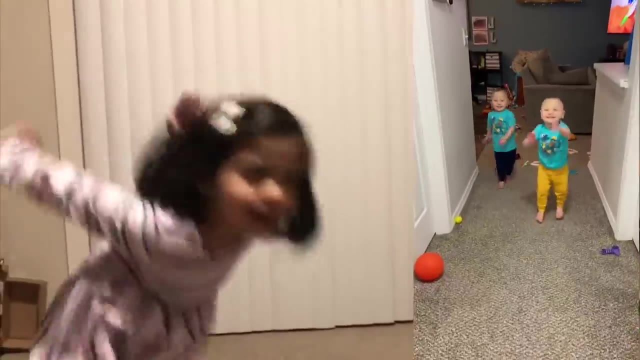 on a flower and drink the nectar up. Land on a flower and drink the nectar up. The nectar tastes so yummy, Good job. Now let's fly around a little more. Are you getting tired? Let's take a rest on a leaf Butterflies. don't like leaves Butterflies, don't like leaves- Butterflies. 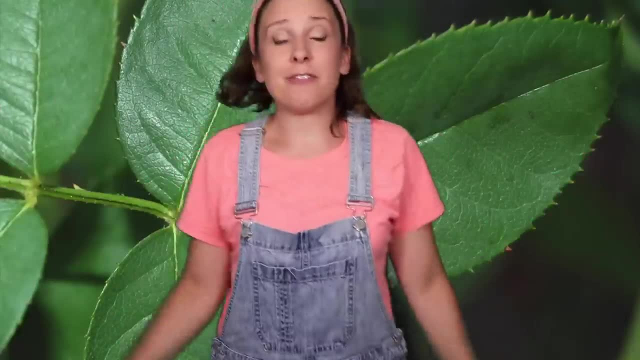 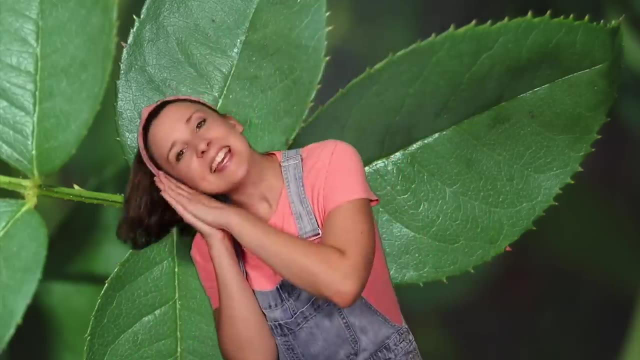 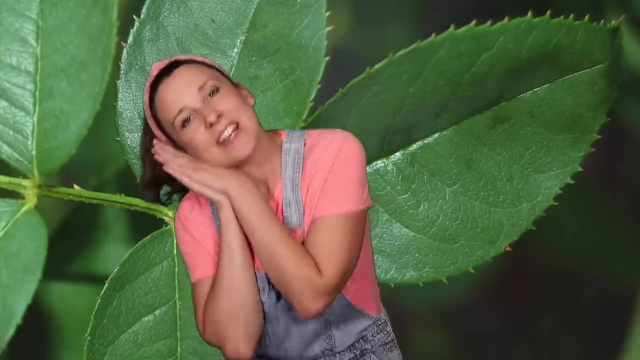 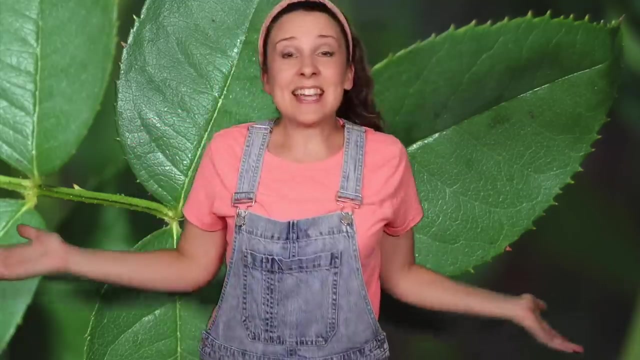 don't sleep, But they rest. Let's rest on a leaf. Land on a leaf and take a rest. Land on a leaf and take a rest. Land on a leaf and take a rest, Because we are so tired. Let's rest on this leaf. So nice to take a rest. Let's get up and fly again. Are you ready? 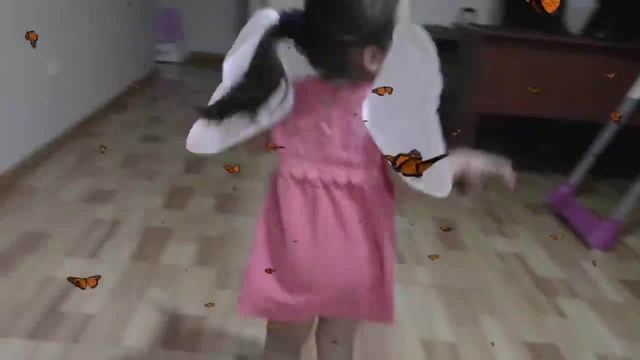 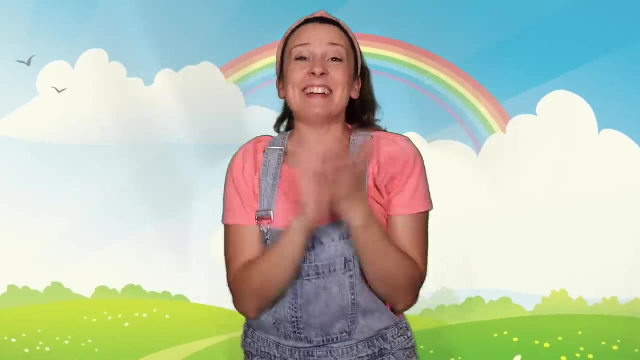 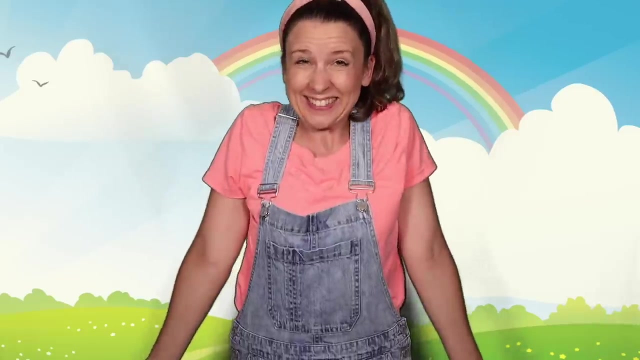 Fly, fly like a butterfly, Fly, fly like a butterfly, Fly, fly like a butterfly. Let's fly, fly, fly like a butterfly, fly, fly like a butterfly, fly around the yard. Great job, Wow, You did a wonderful job being a butterfly. 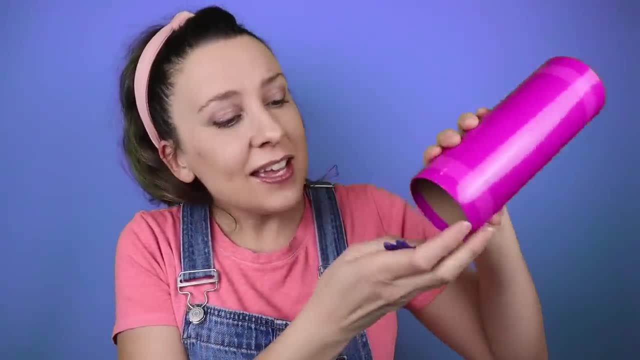 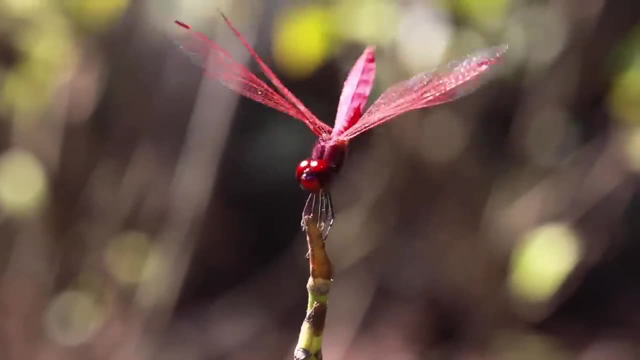 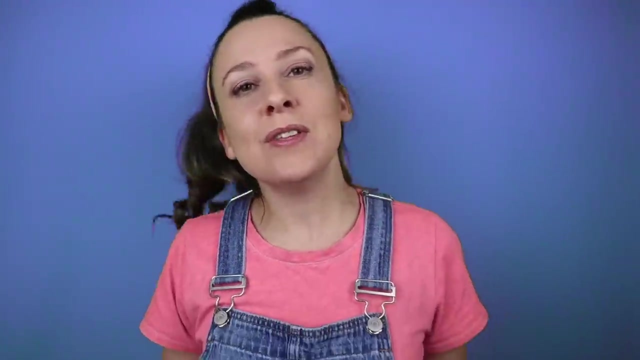 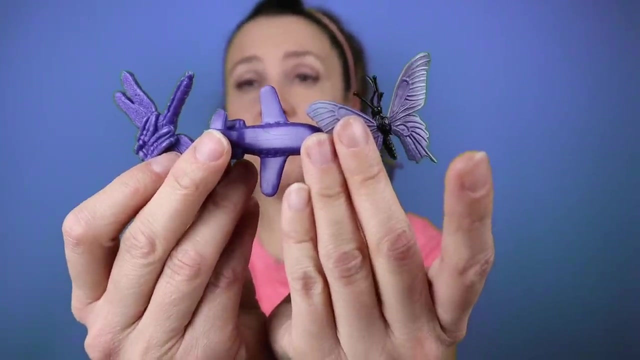 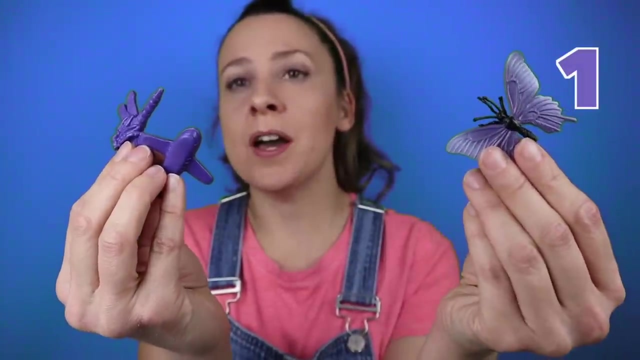 It's another thing that flies. It's a dragonfly. Oh, can you fly like a dragonfly? Maybe we can buzz a little bit. Can you do that? You're a dragonfly. Wow, I can't believe it. We found three things that fly: A butterfly, a plane and a dragonfly. One, two, three. 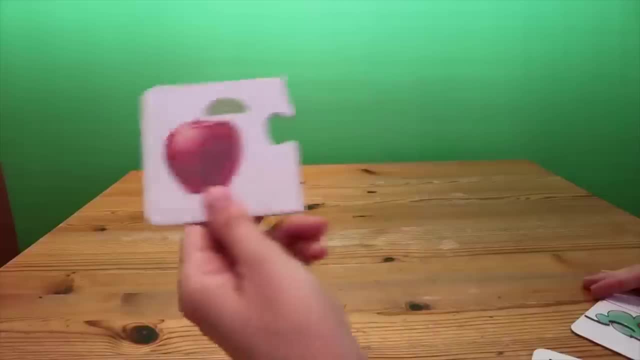 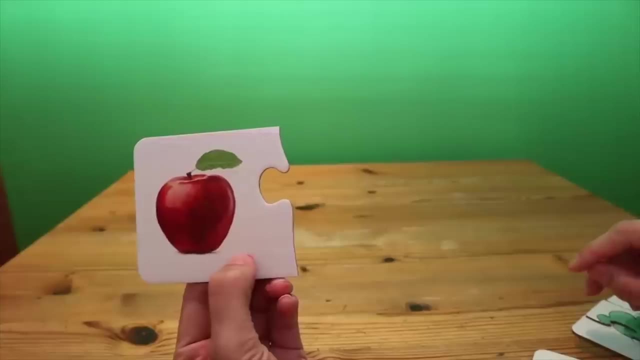 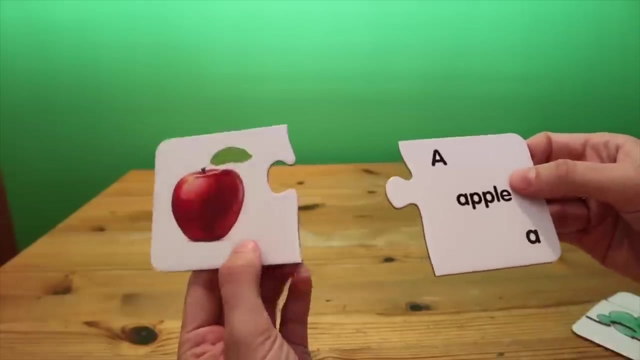 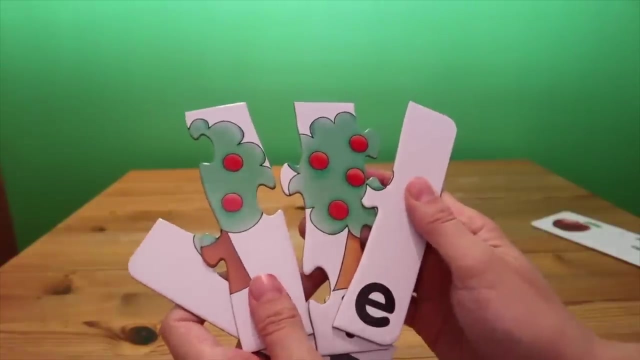 I found some puzzles. Can you help me with them? Thank you. So here's an apple. What letter does apple start with? Apple? Yeah, A. So let's see if this fits. It fits Good job. Oh my goodness, This puzzle looks hard. Can you help me? What do you think it's going to be? 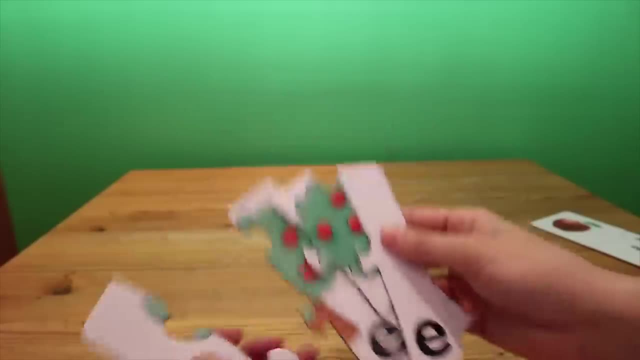 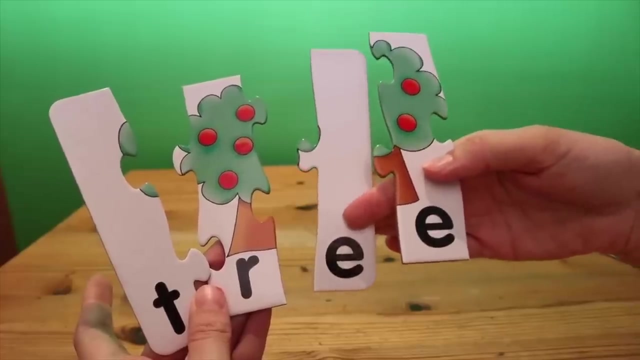 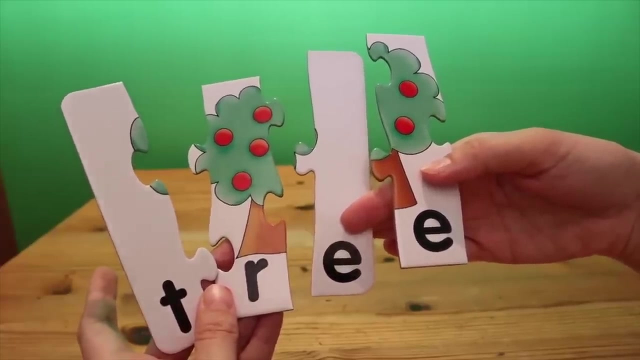 Hmm, let's see. Wow, I see a lot of letters. Let's sound them out and see what it spells. The T says T, The R says R And the E's say E, T-R-E, T-R-E- Tree- I think it might be a tree. 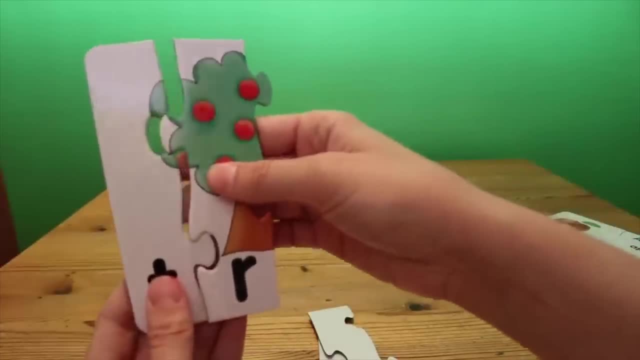 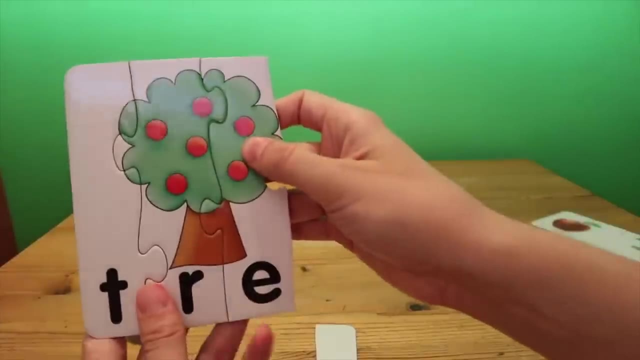 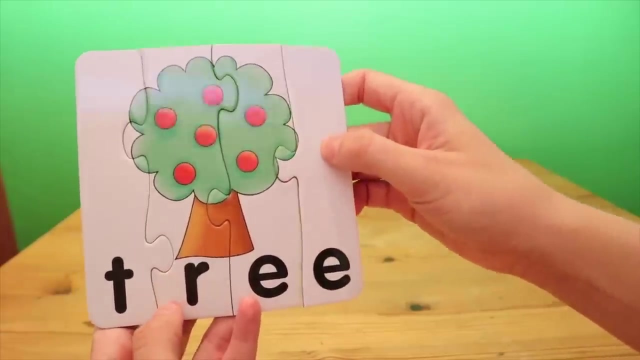 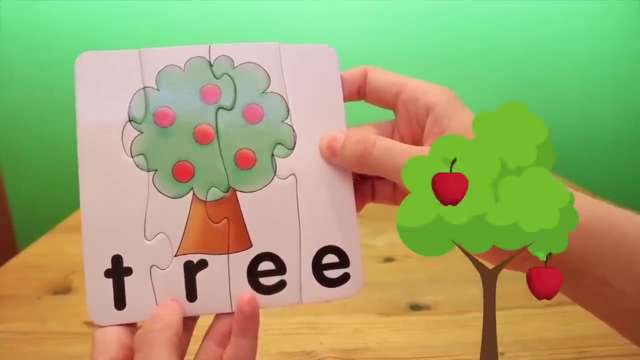 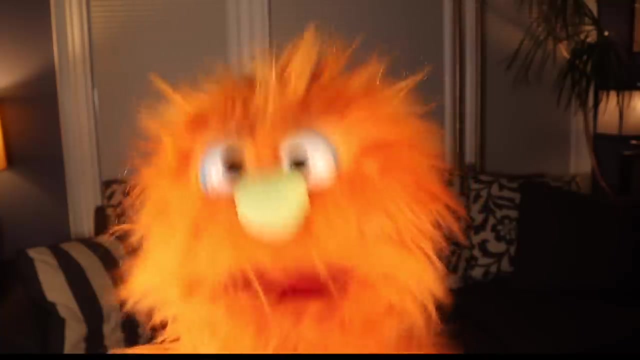 Let's see, Put it in, put it in, put it in. Oh, coming together. put it in, put it in, put it in. wow, i think we were right, you got it. it's a tree, cool tree, an apple tree. i like to ite, ite, ite apples and benign eyes, so silly. wow, i have a big letter a. 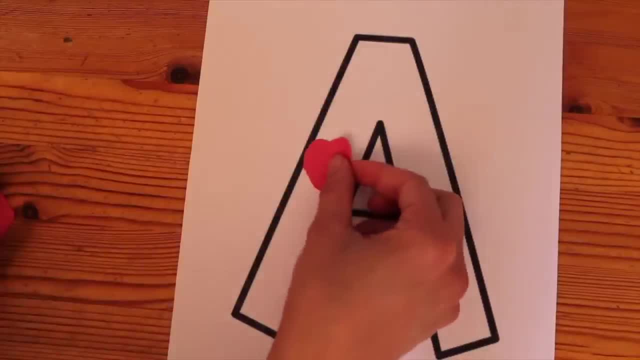 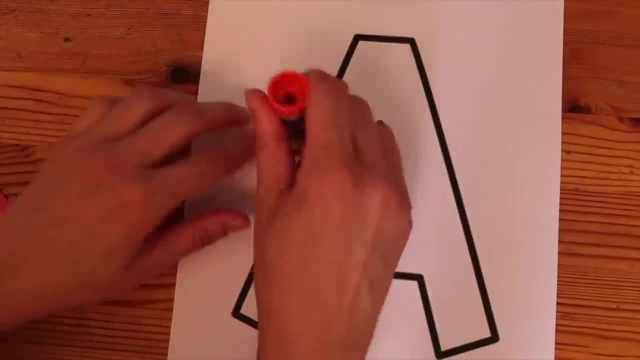 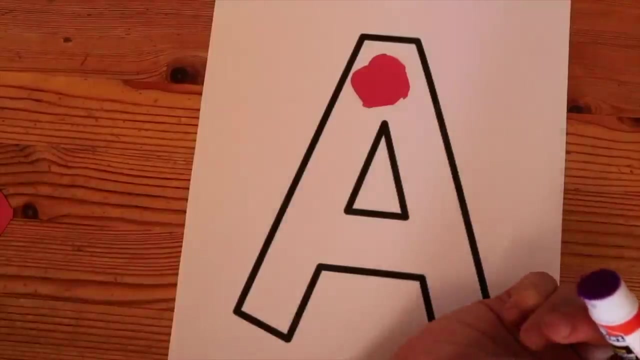 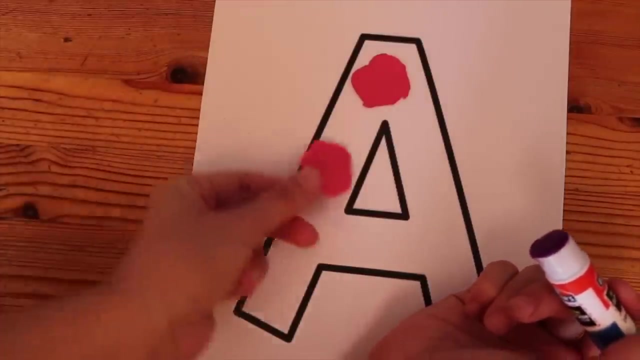 now can you help me glue some little apples onto it? be so much fun. okay, let's get out our glue stick. we put glue on the apple, see, and then we put it on the a. wow, that was fun. take a little apple, put on the glue, say on, and i'll stick it on on. 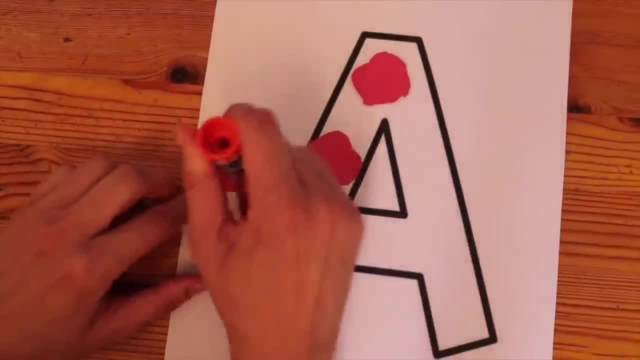 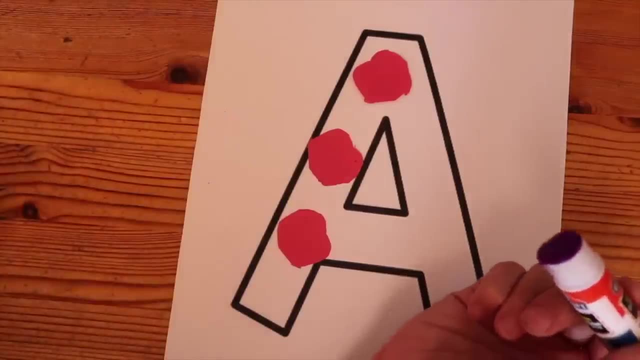 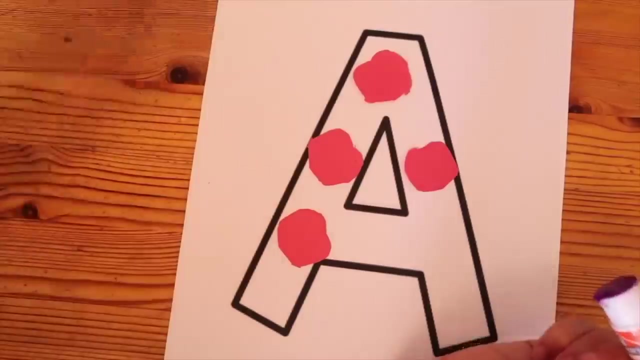 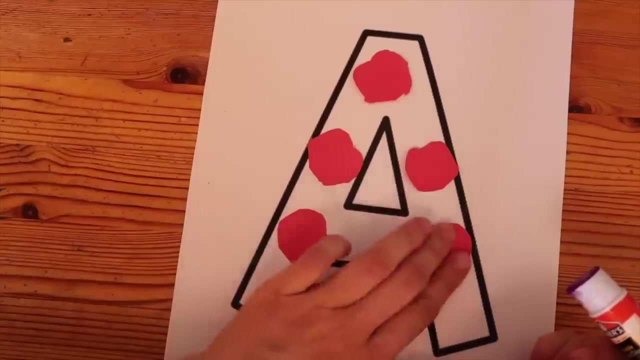 wow, this a is getting covered in apples. the glue is purple. wow, and then i stick it on. can you help me with this one? put on the glue and then say on on, good job. wow, i think the a is so happy to have all these awesome apples on it. On, Let's put one in the middle, Can. 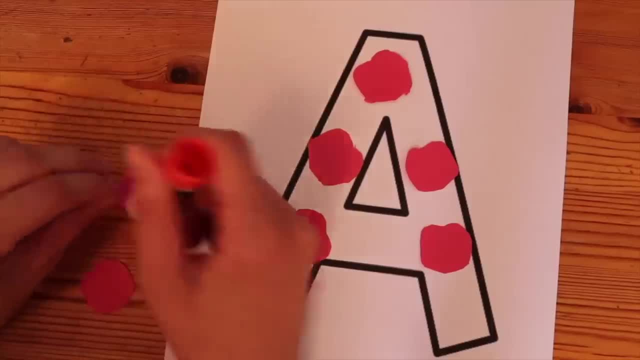 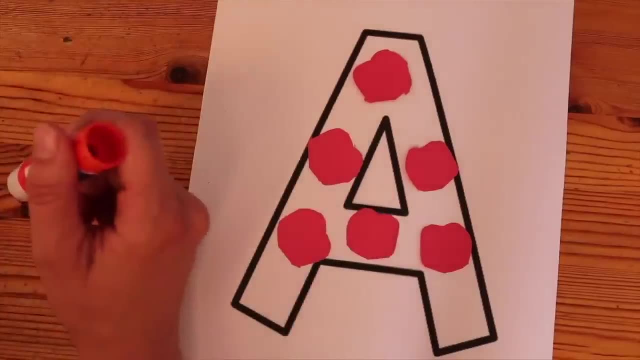 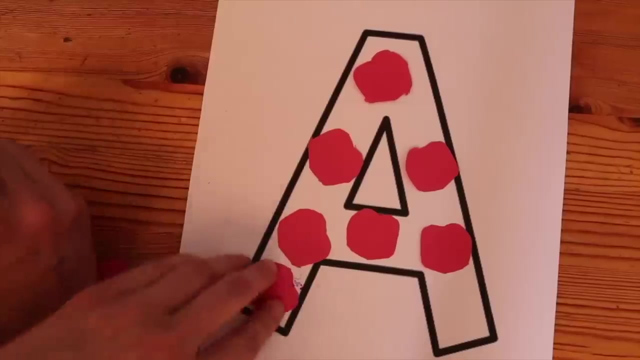 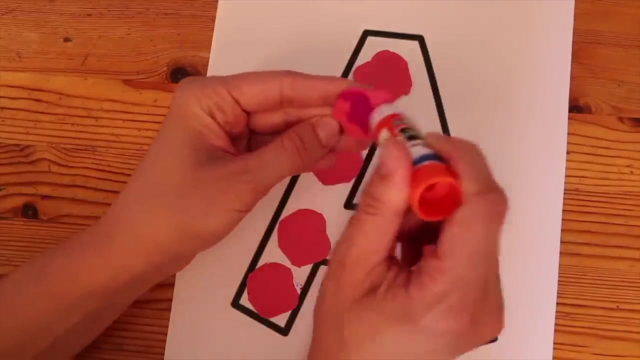 you help. You're such a good helper. I'm so happy to be spending time with you. On Good job. You helped me Say on, and I'll put one right here On Good job. See how I put the glue on. Yeah, fill it with glue so it sticks. Put it on, put it on, put it. 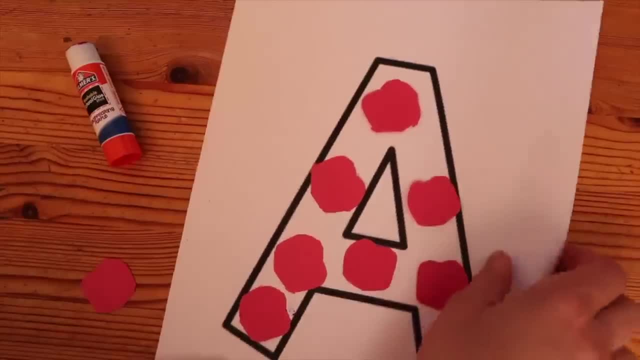 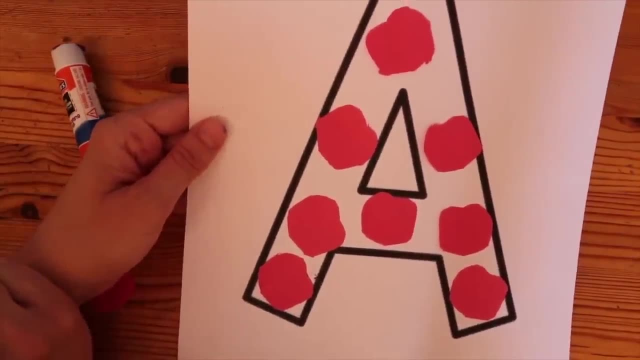 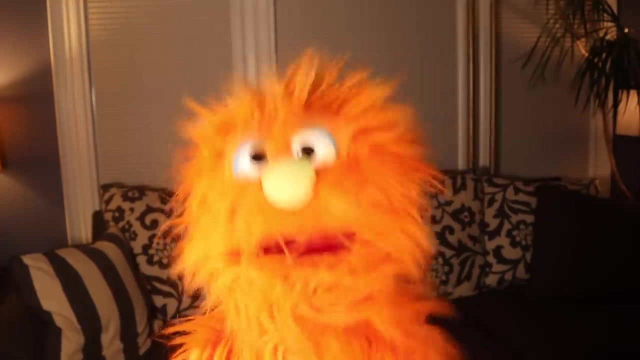 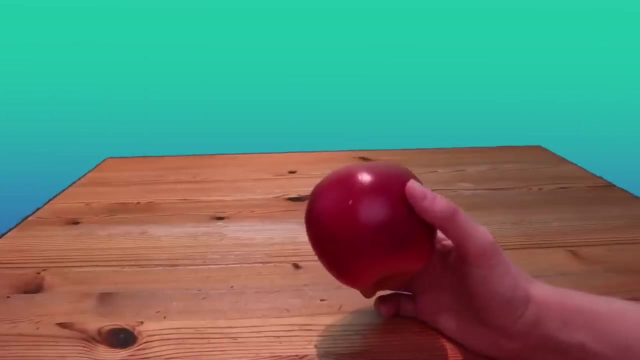 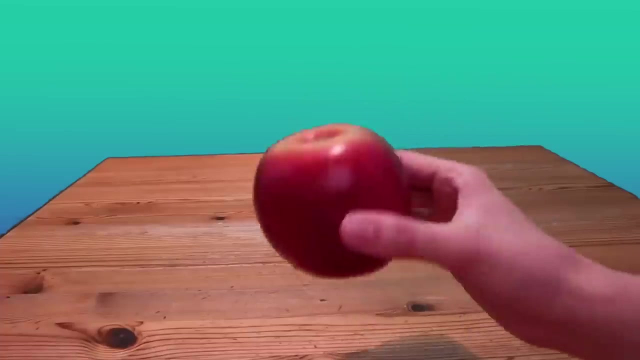 on. Wow, friends, Look what you helped me make. I'm so proud of you. We made an A with apples stuck all over it- So awesome. Why do oranges do so well in school? They concentrate. Guess what I found in our music bag. I found a shaker That's an apple, A red apple, Apples. 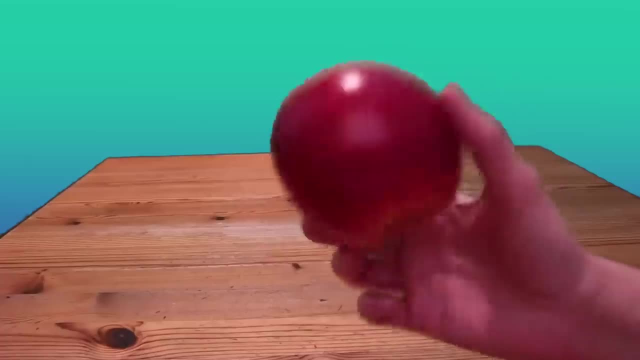 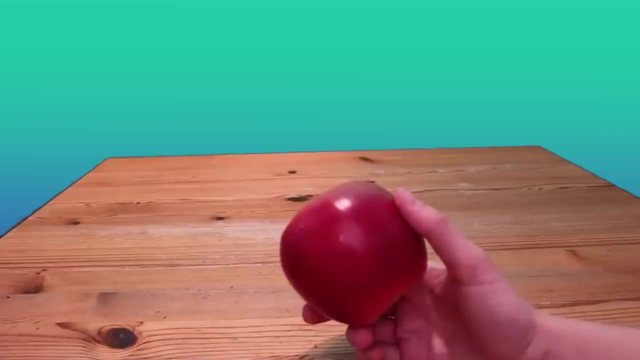 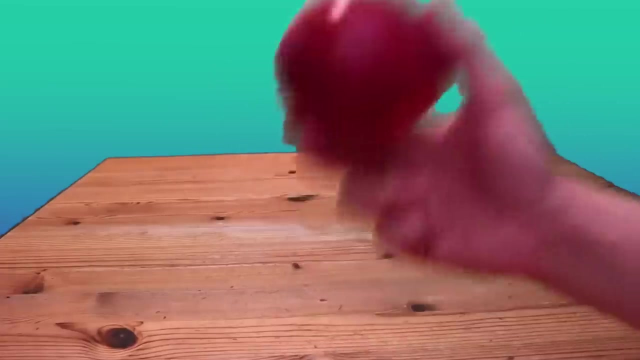 are what we're learning about today. And it's red And it's musical. Let's shake it and sing a song with it. Hmm, remember how we were doing a beat to the Muffin Man? Let's try that. Do you know the Muffin Man? the Muffin Man, the Muffin Man. 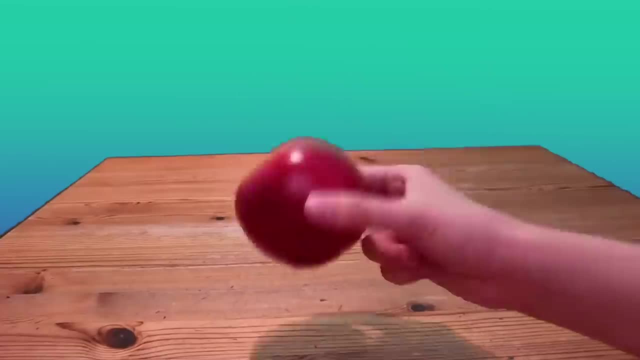 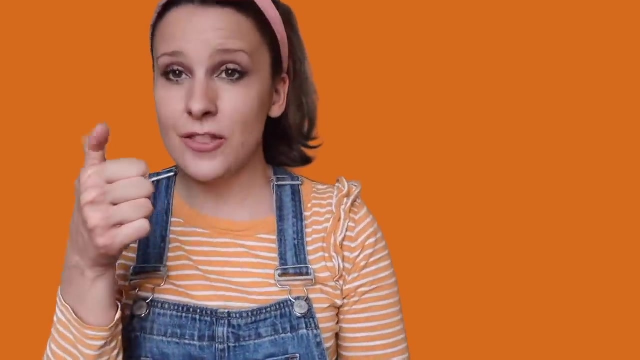 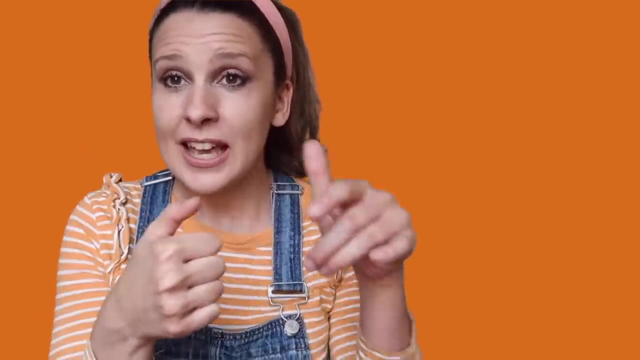 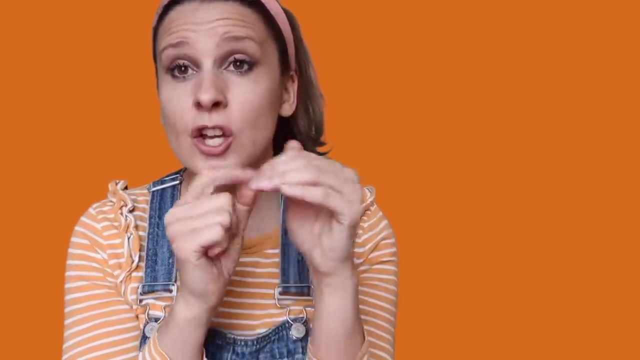 Do you know? the Muffin Man who lives on, true remains, Wow, an apple shaker. So fun. Can you pretend your little thumb is a mouse? Then your other hand's going to be the house. A quiet little mouse in a quiet little house, When all was quiet as quiet can be. Sh, sh. 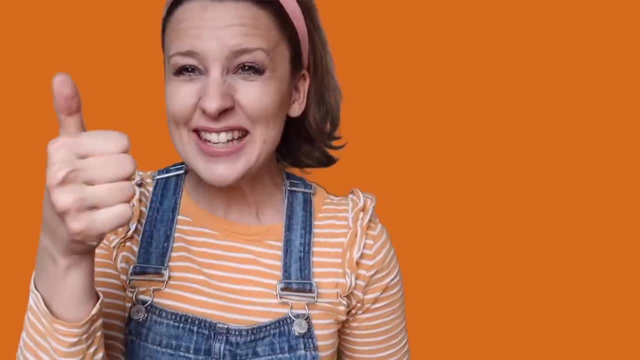 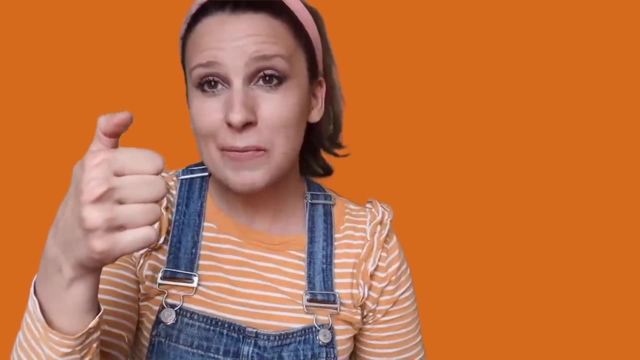 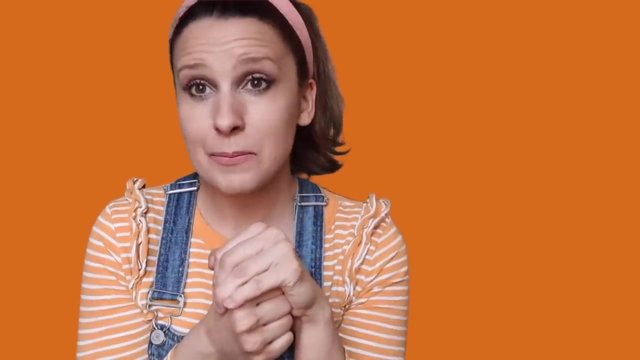 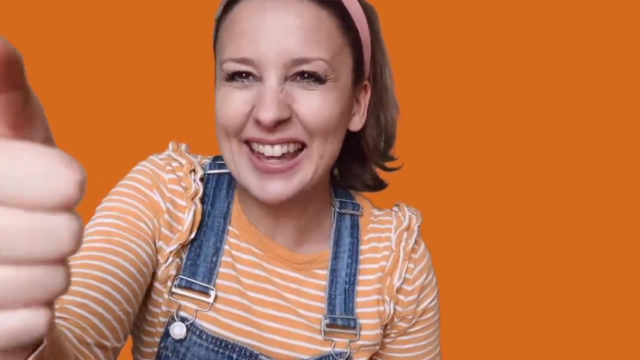 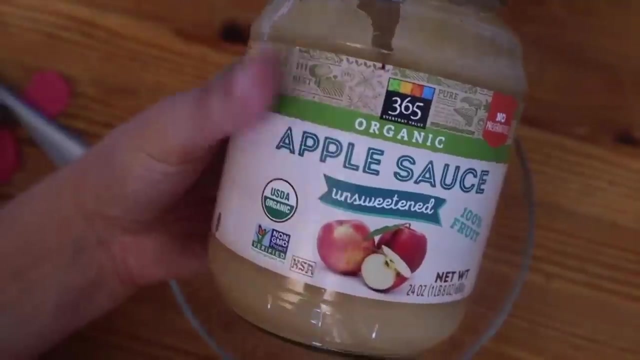 sh Apple tea. That was so silly. A quiet little mouse in a quiet little house, When all was quiet, as quiet can be. Sh sh sh Apple tea. That was so silly. The little mouse surprised us. Good job, Look what I have: It's applesauce. 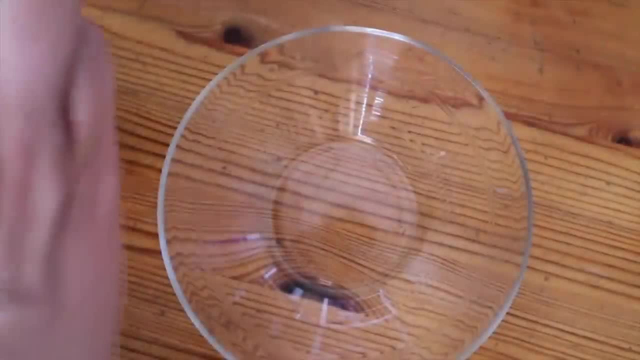 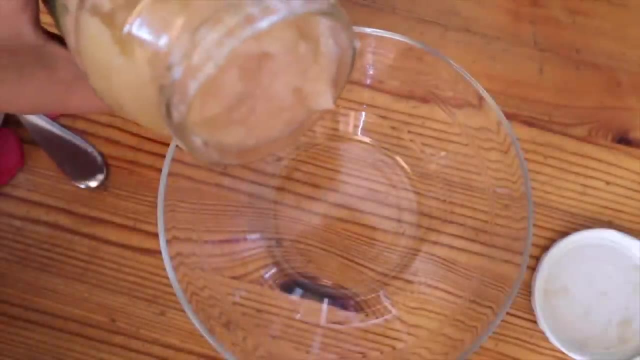 What are they For our next project? we're going to pour the applesauce into the bowl. We twist off the cover, Twist, twist. Now we're going to pour the applesauce in. Can you say pour, Pour Good job. 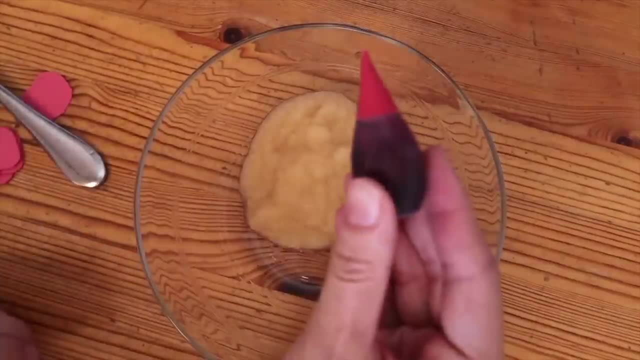 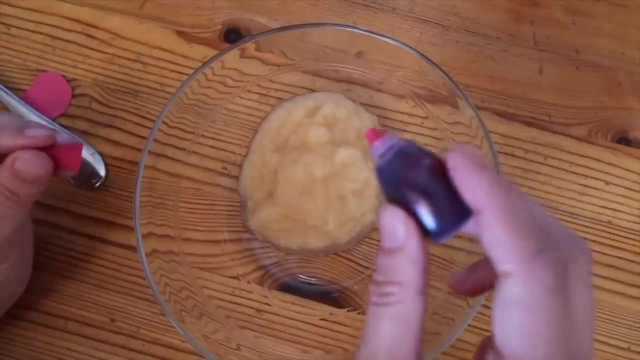 Pour. Since the color of the day is red, I'm going to get out some red food coloring. If you want to do projects, remember always to ask for a grown up's help. Now we put a little food coloring in. Let's try one drop. 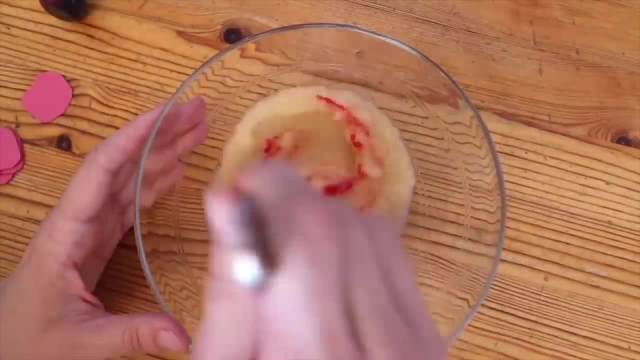 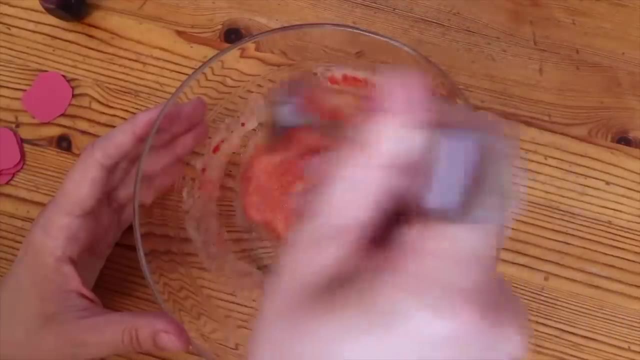 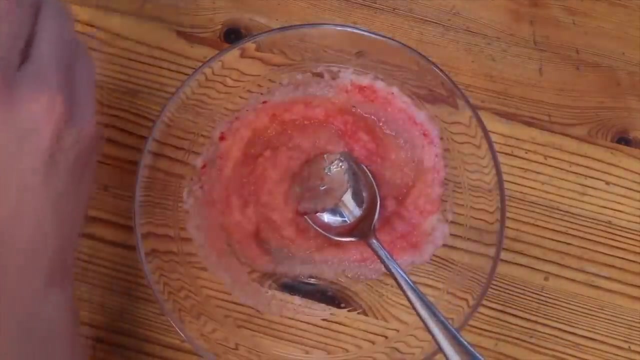 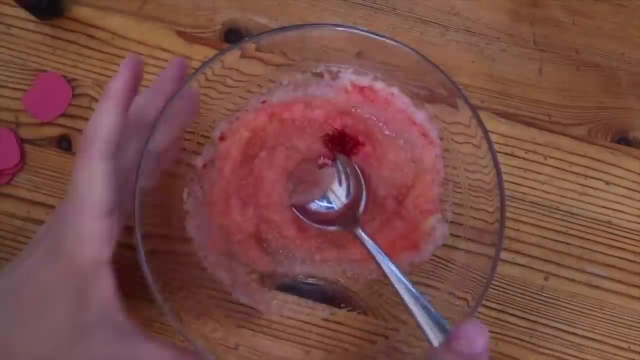 We're going to mix it. Can you say: mix, Mix. Wow, The applesauce is turning red. It looks kind of pink. I think we need more drops. Let's squeeze, Squeeze it. Two more drops and we'll see what color it is. 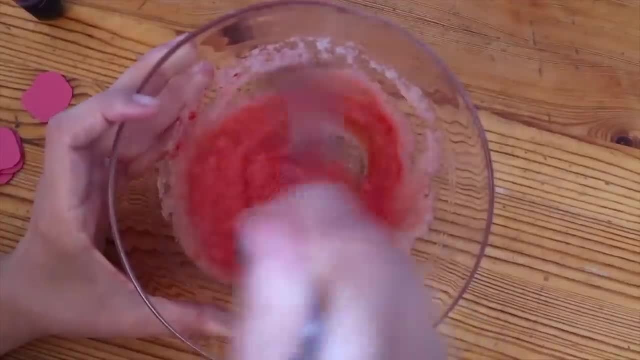 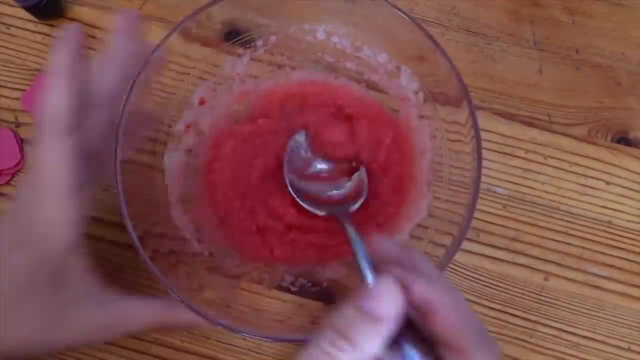 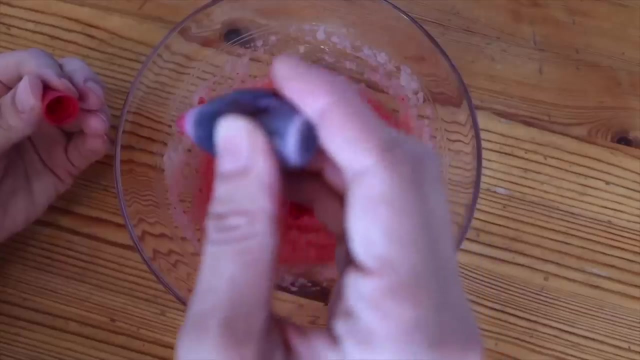 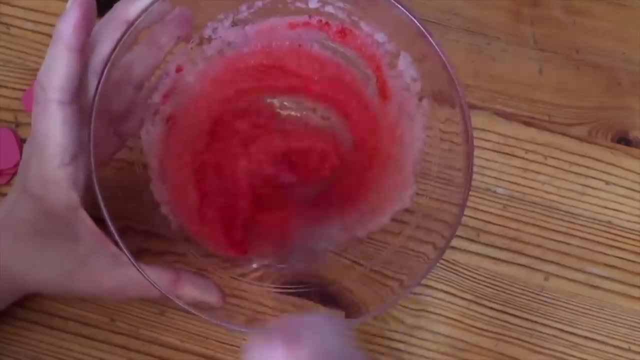 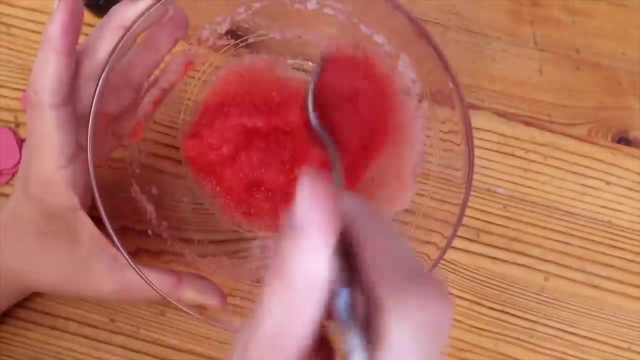 It's starting to get more red. This is called mixing. It still looks kind of pink. Let's add more drops. Let's add three drops. One, two, three. Wow, We have red applesauce. The color of the day is red. 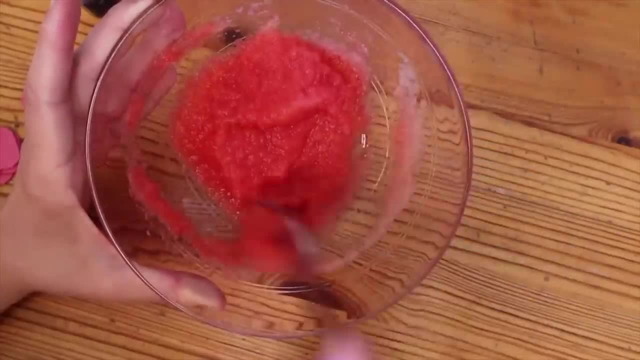 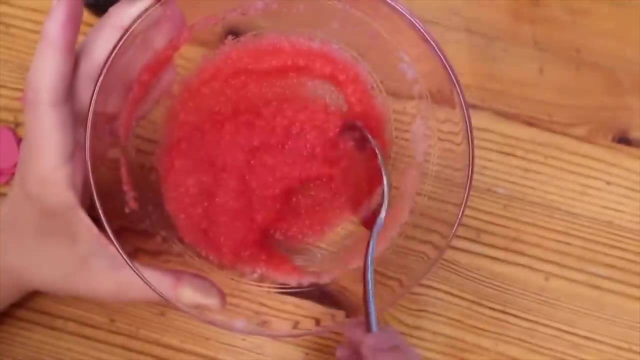 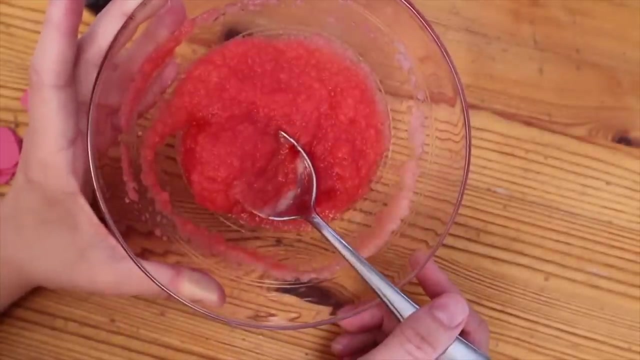 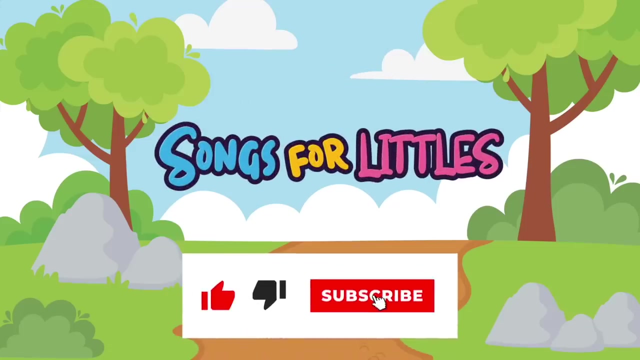 Yummy, Yummy, red applesauce. Good job, Let's mix it a little more. Mix, Mix, Mix the applesauce. Wow, Let's pretend to eat it. Wow, Great job, making red applesauce with me. Songs for Littles. Songs for Littles.